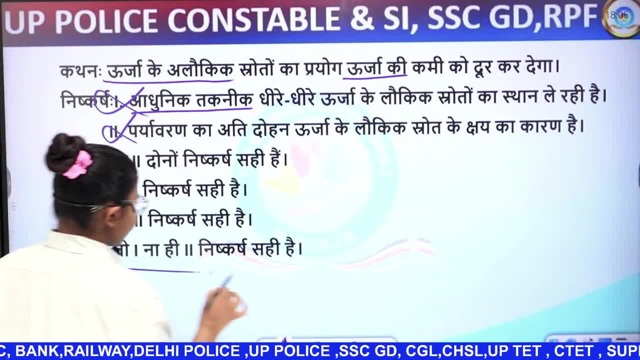 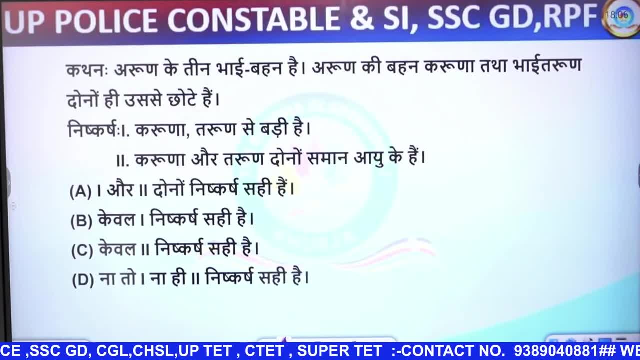 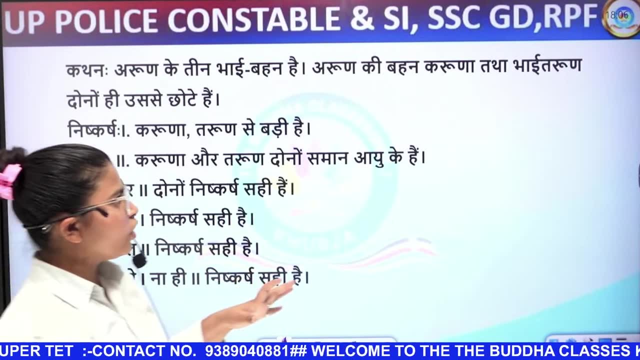 What will be the correct answer to this? Neither the first nor the second is correct. Option number D will be the correct answer to this. Look at the next question. The question is given. Arun has three brothers and sisters. Arun's sister Karuna and brother Tarun are both younger than him. 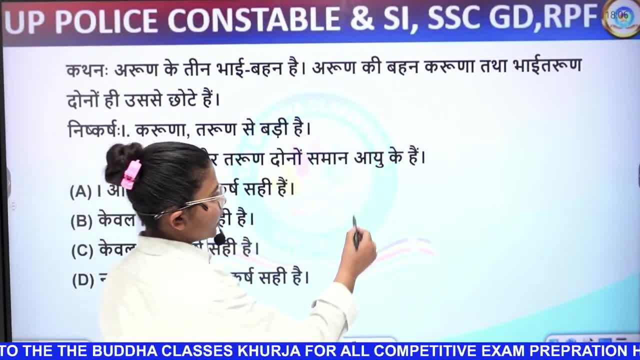 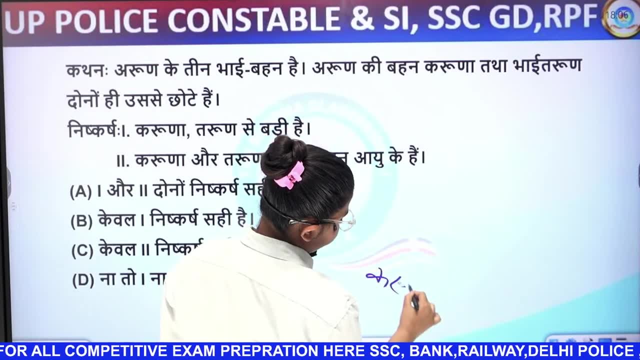 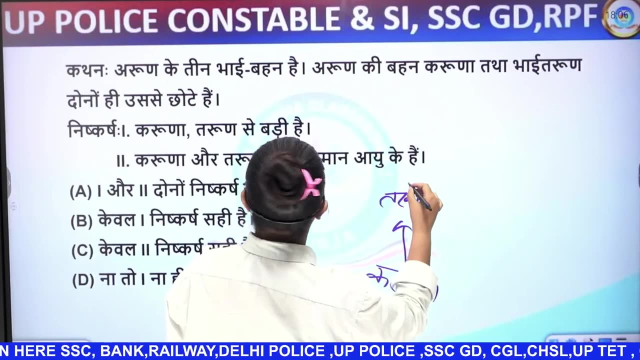 Arun's sister. What is the name of Arun's sister, Karuna? Karuna is younger than both her brothers. That means Karuna is the youngest. She has two brothers: One is Tarun and one is Arun. What is the difference between Arun and Tarun? 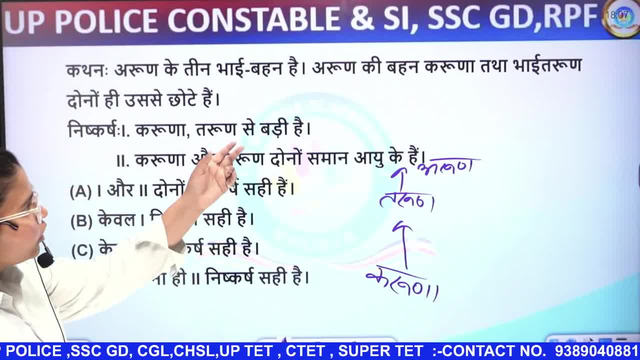 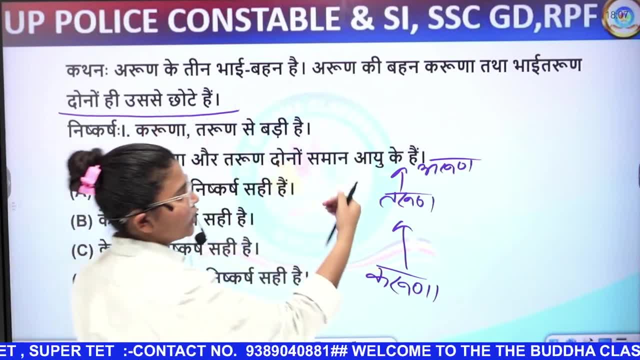 What is the difference? All three of them have younger brothers and sisters. Okay, Karuna is the eldest here. Karuna is the eldest here. Karuna is the eldest here. Arun and Tarun are younger than him all. What is the difference? 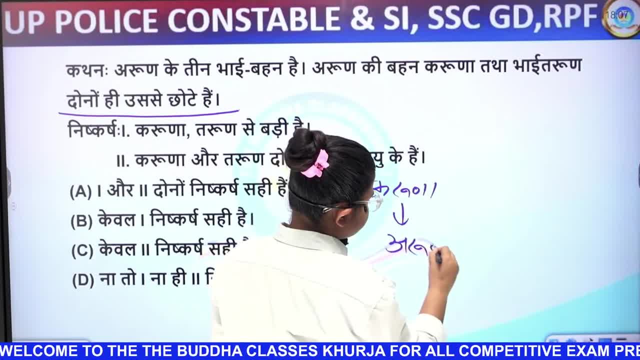 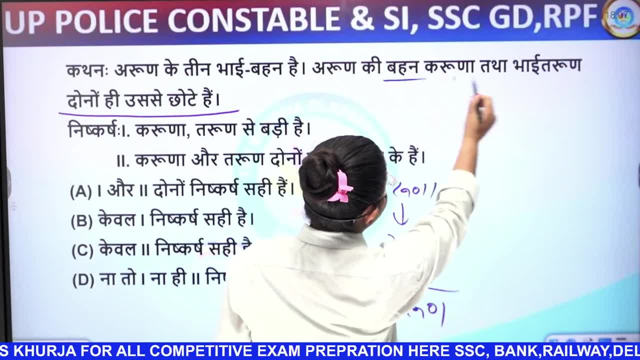 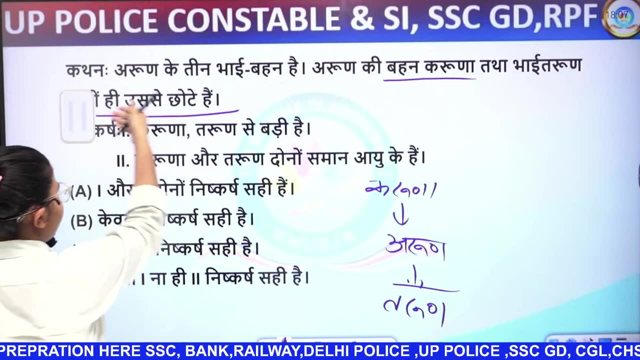 This is the difference. All three are younger. here, Arun and Tarun are both younger than him. Look It is written: Sister Karuna, sister Karuna, Brother Tarun is younger with Karuna and brother Tarun, And Both brother and sister-in-law are younger than him. 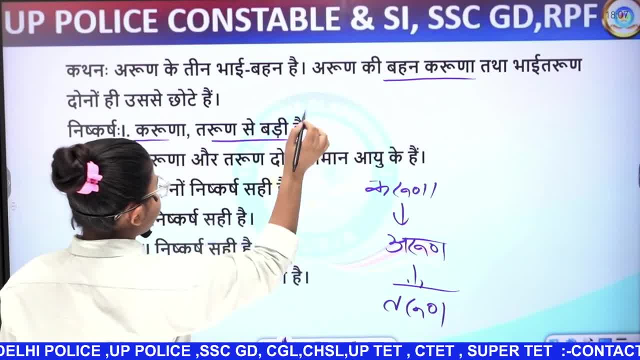 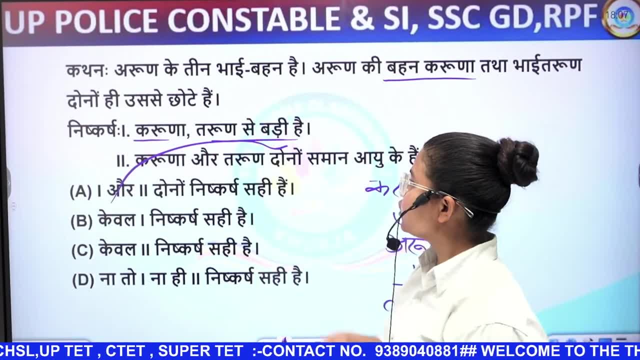 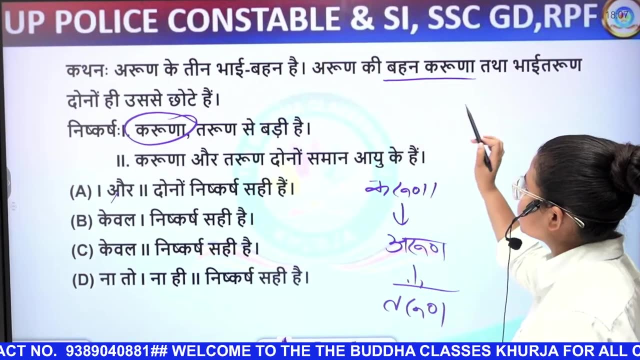 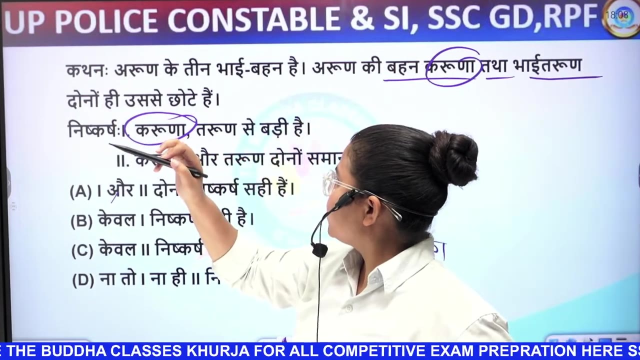 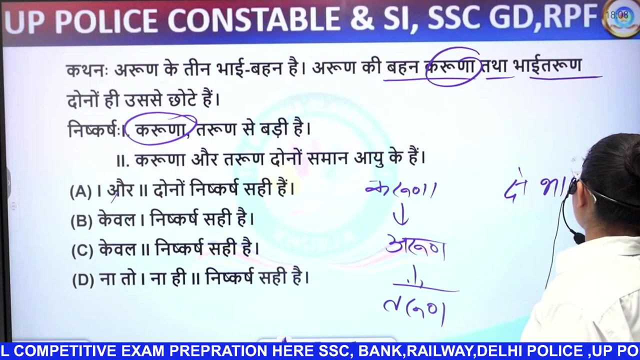 Discuss. number 1 is that: is Karuna older than Tarun? Can Karuna be older than Tarun? Is Karuna older than Tarun? It is said that Karuna and Tarun are younger than Karuna. Both brothers are younger than Karuna. 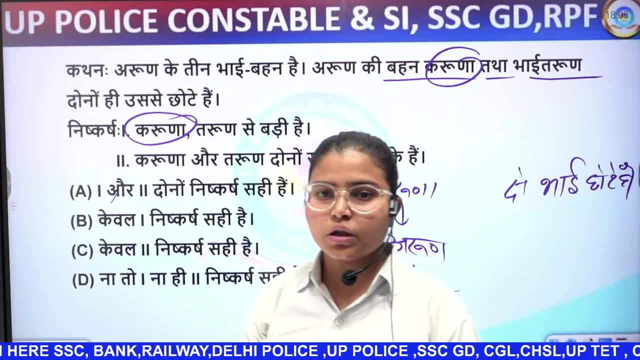 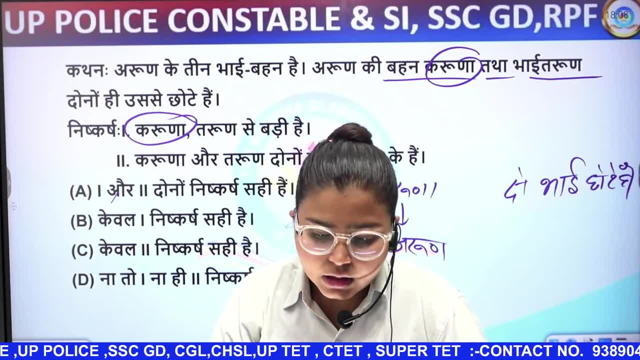 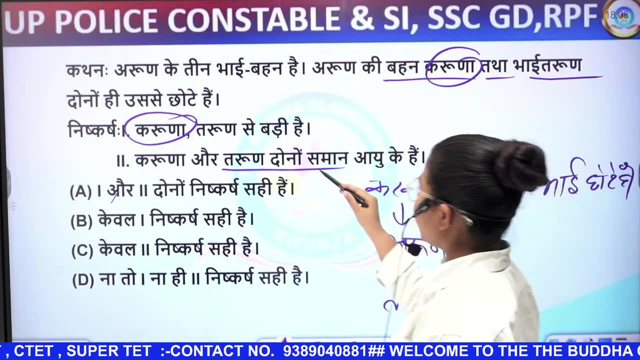 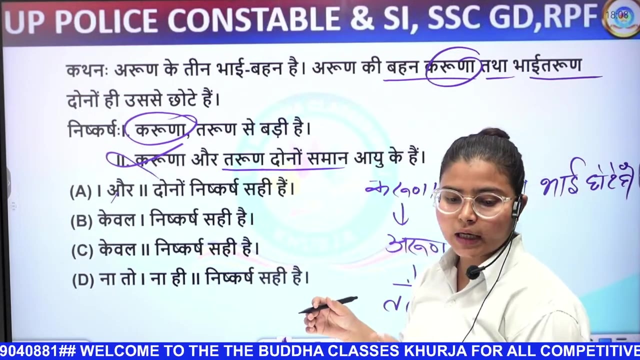 Discuss. number 1 is that: is Karuna older than Tarun? Is Karuna older than Tarun? Is Karuna older than Tarun? It is said that Karuna and Tarun are of equal age. It is said that Karuna and Tarun are of equal age. 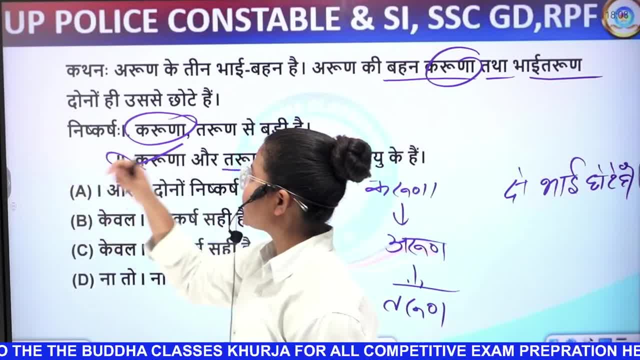 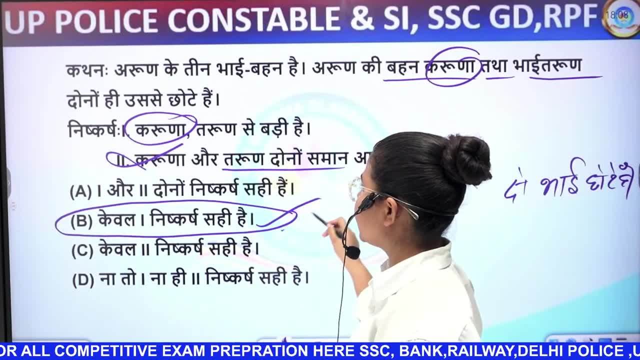 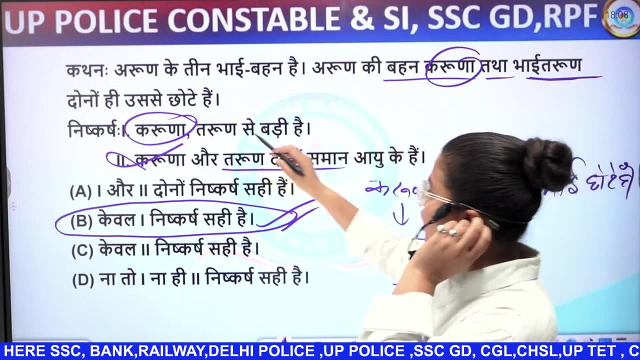 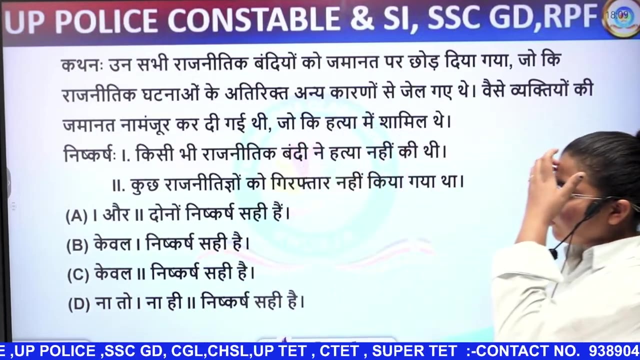 It is said that Karuna and Tarun are of equal age. The correct answer is Discuss number 2.. It is said that Karuna is older than Tarun. Both brothers are younger than Karuna. Next question: It is said that all political prisoners were released on bail. 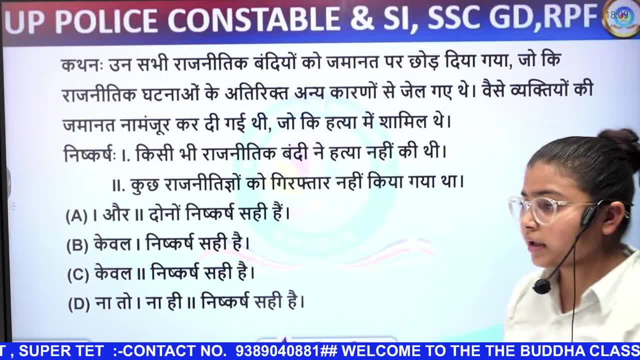 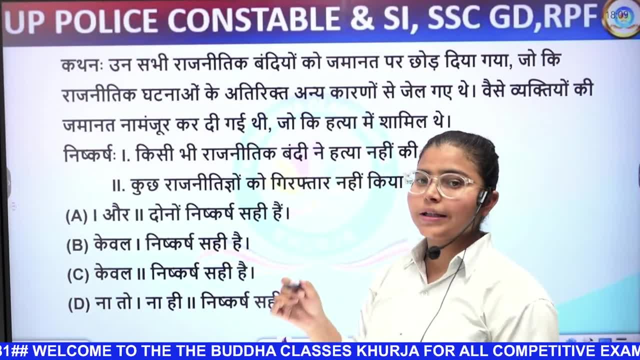 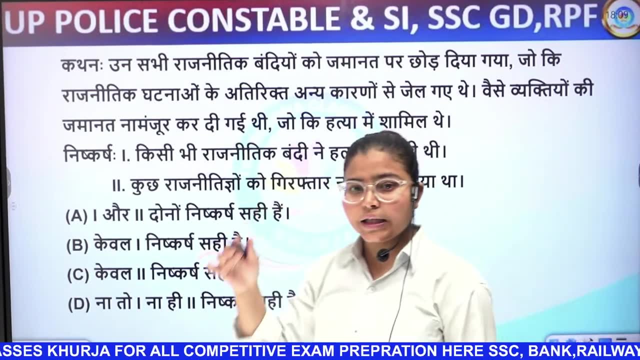 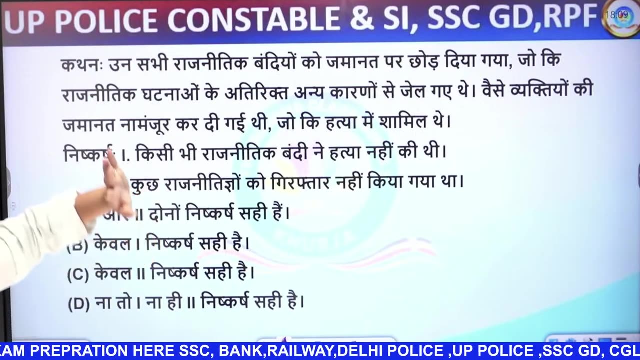 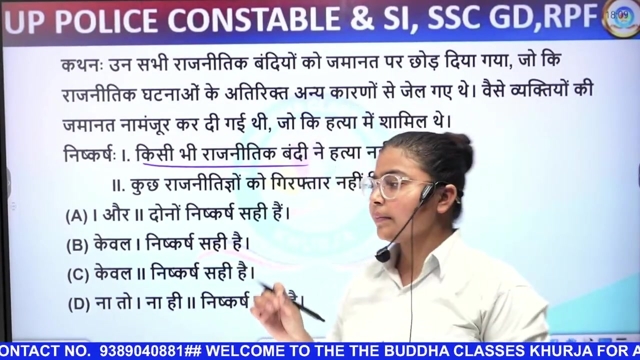 who were imprisoned for other reasons other than political incidents. The bail of such people was not approved. who were involved in the murder: The bail of such people was not approved. who were involved in the murder? who wereporteilles? Did not any political prisoner kill? 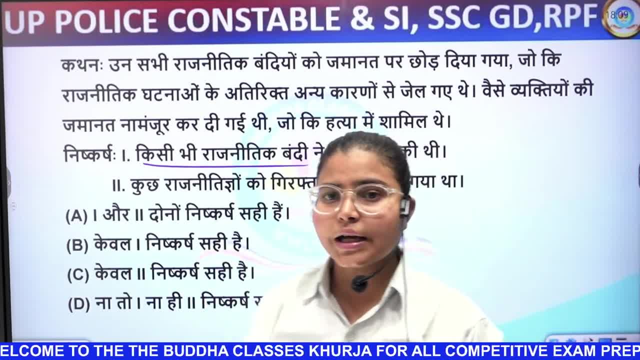 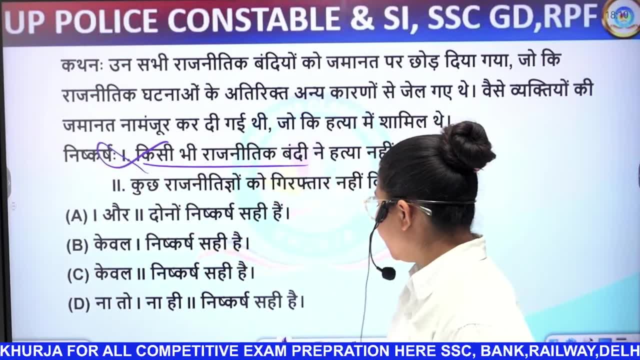 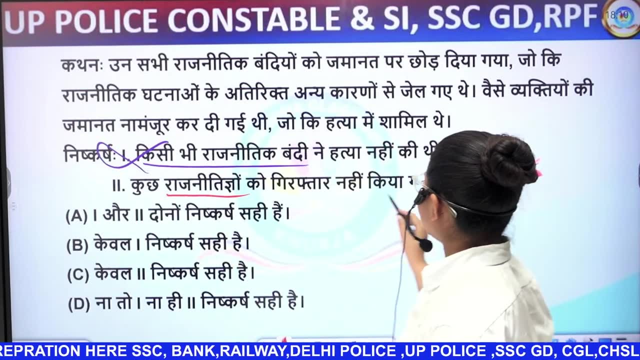 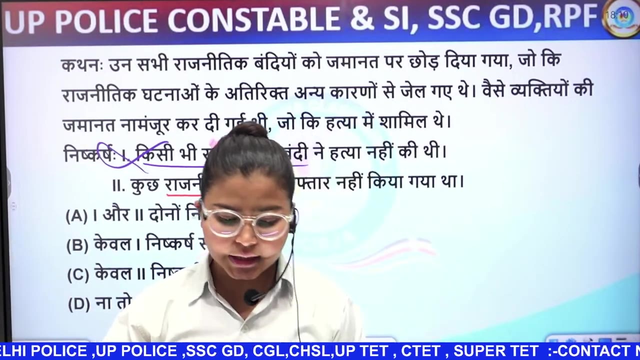 Can we say that the political prisoner cannot kill? If we can't say that, then the first question is wrong. In the second question it is said that some political prisoners were not arrested. Yes, we can say that some political prisoners were not arrested. 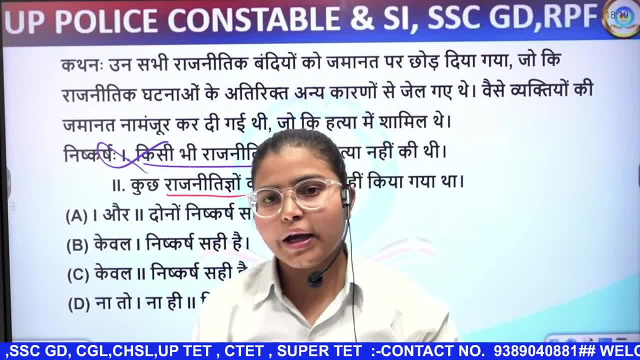 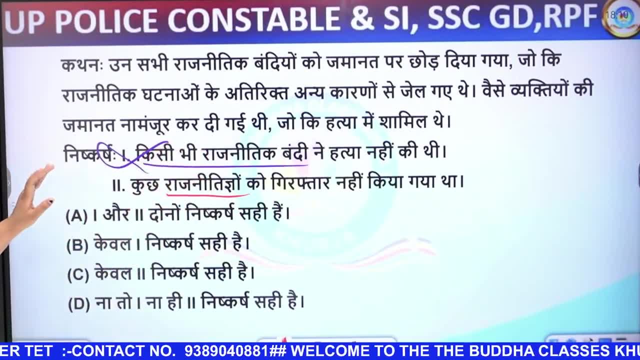 Okay, Some political prisoners were not arrested Because in the question it is said that they were jailed for other reasons. Right, They were jailed for other reasons. Because they were jailed for other reasons, Right, Some people were not arrested. We can accept this. 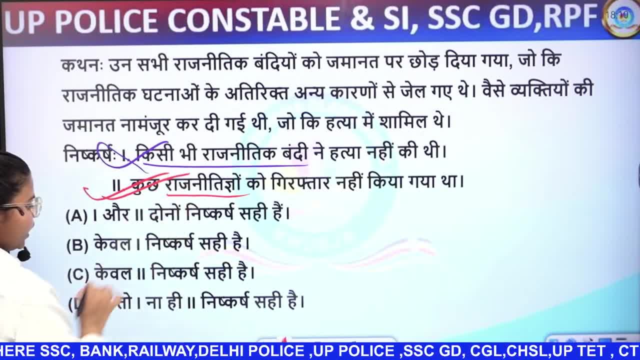 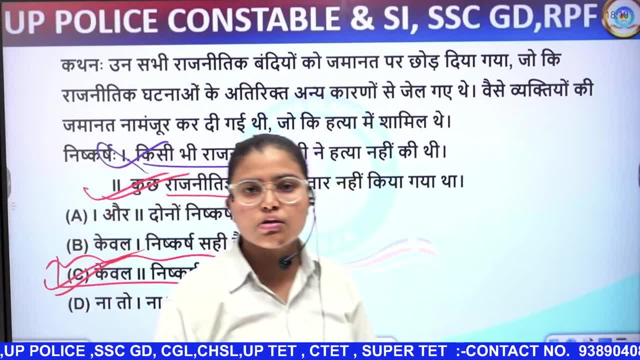 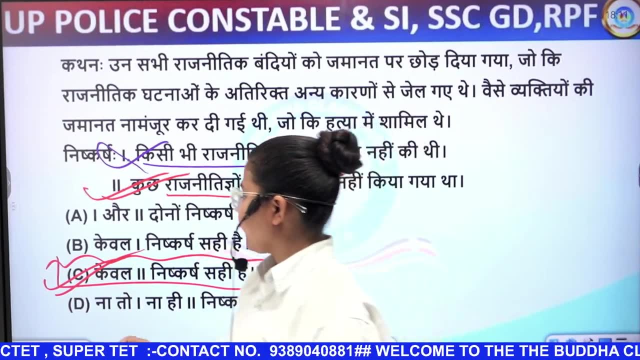 So the second question is correct. The correct answer is option number D. Option number C: The correct answer is option number C. The second question is correct. Okay, What is it? The second question is correct. Look at the next question. 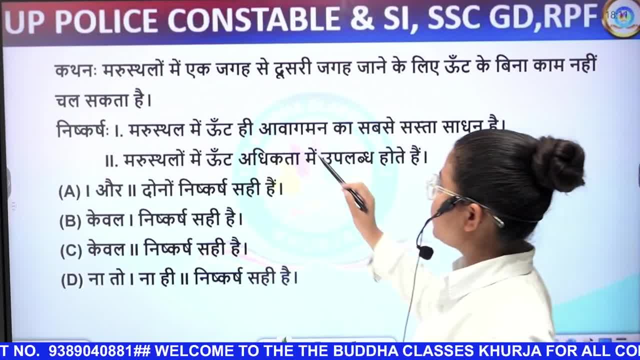 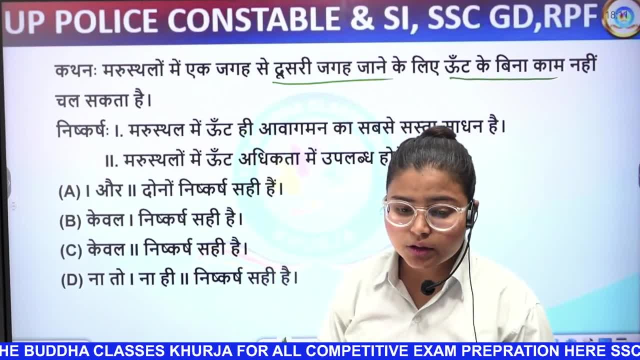 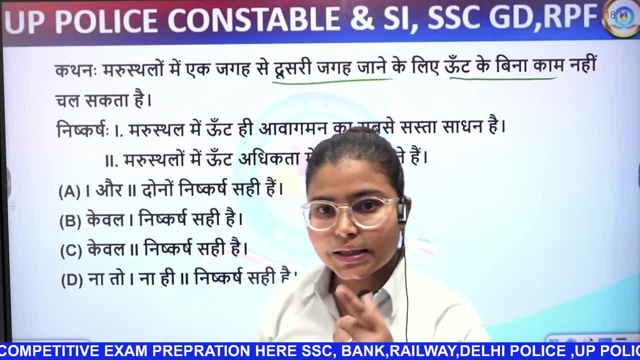 The next question is given: In Maroons, to go from one place to another, work cannot be done without camels. In Maroons, to reach from one place to another, work cannot be done without camels. Option number 1 is given. 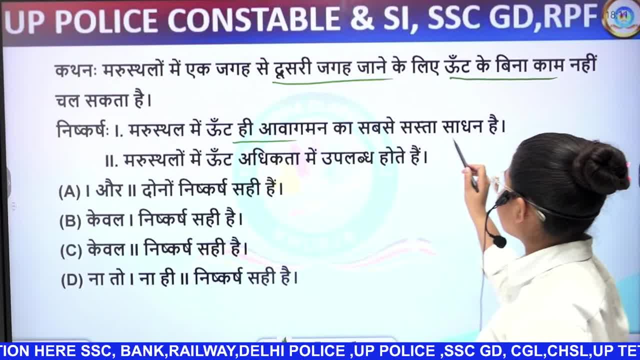 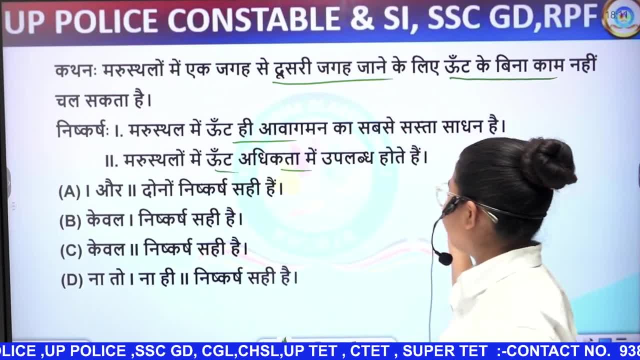 In Maroons, camels are the cheapest means of income. Option number 2 is given. In Maroons, camels are available in abundance. Which option will follow in this? How do we know which option will go? Let me explain it to you. 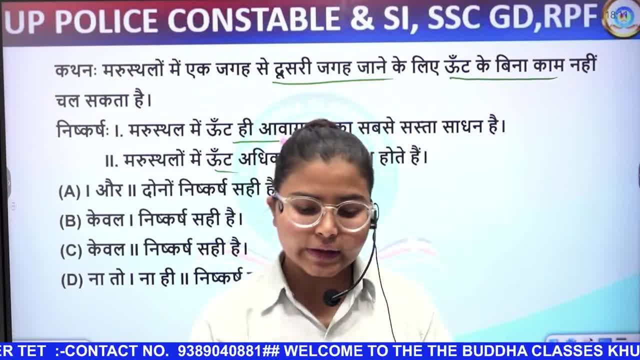 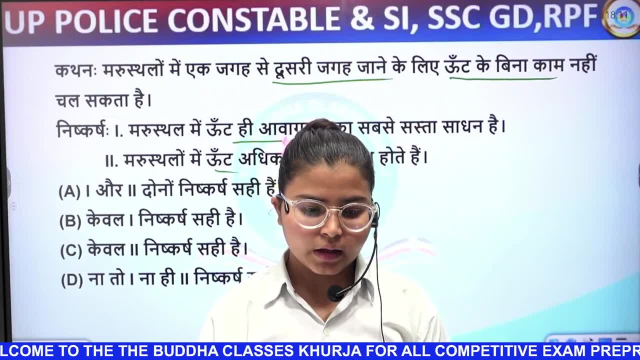 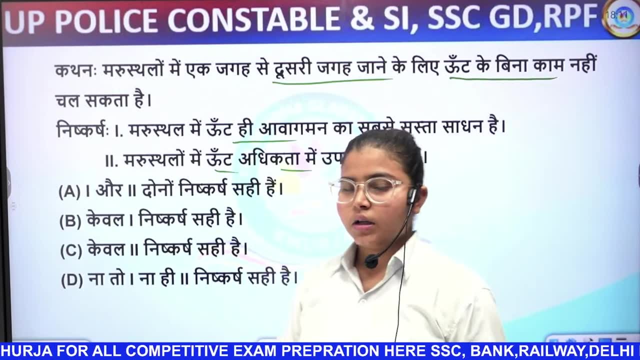 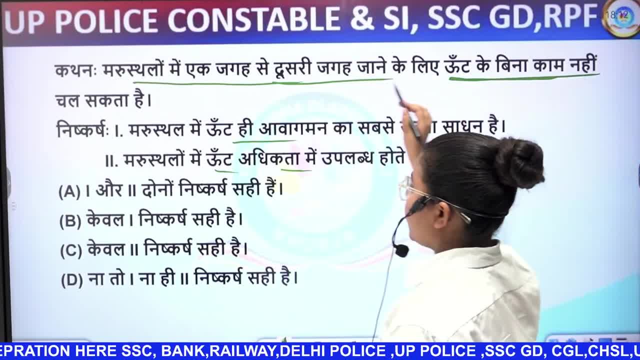 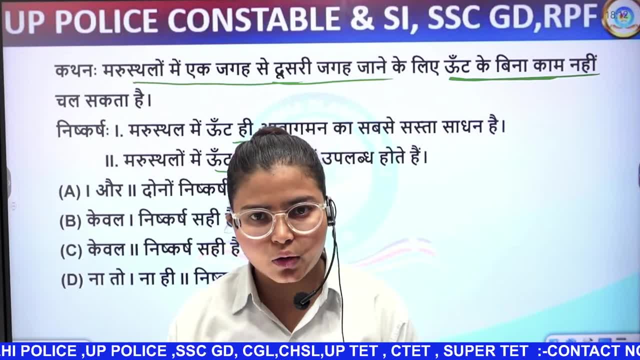 Yes, Yes, Yes, Yes. It is possible that in Marunsthal the camels that do Awa Gavan have a cheap rent. Like we go from here to Delhi, we have to pay a cheap rent on the train, right. 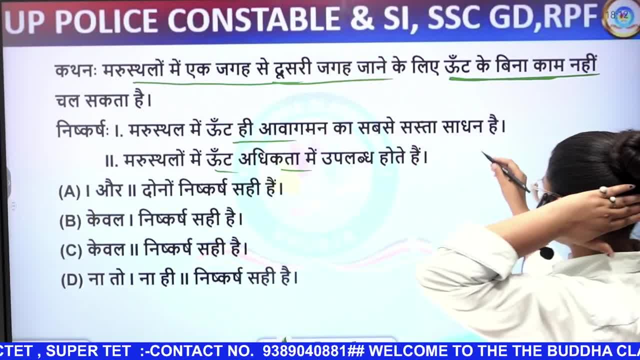 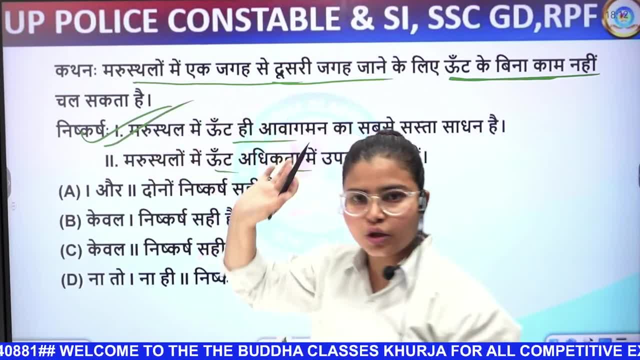 So, in the same way, it is possible that Awa Gavan has a cheap resource, Yes, it is possible that camels have a cheap resource in Marunsthal. Now we can follow this first: Camels are mostly available in Marunsthal. we cannot say this. 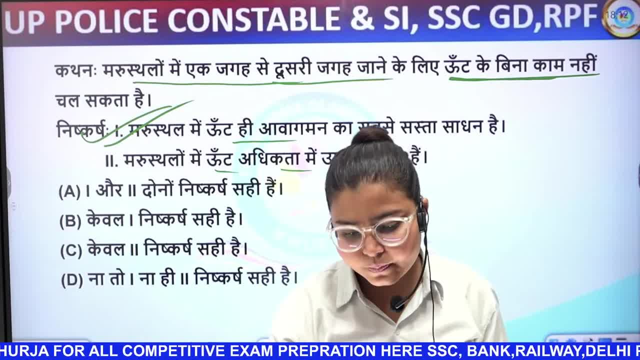 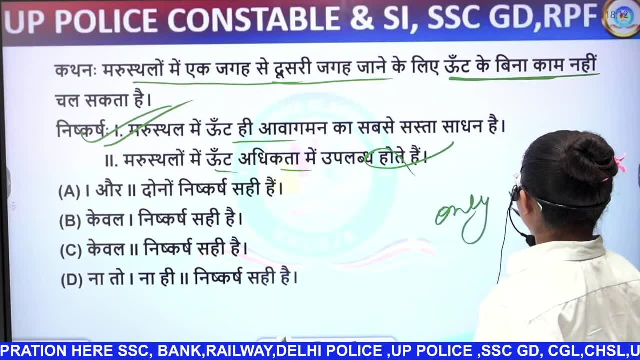 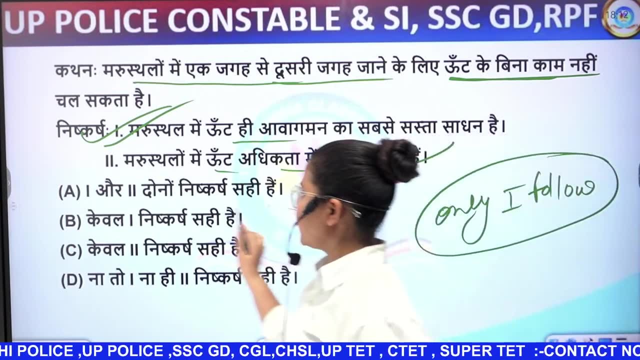 Camels are mostly available in Marunsthal. we cannot say this. So the option is not to follow the number two, Only first to follow. What will you say? Only first to follow, Only the number one follows. The right answer to this will be that only the number one is correct. 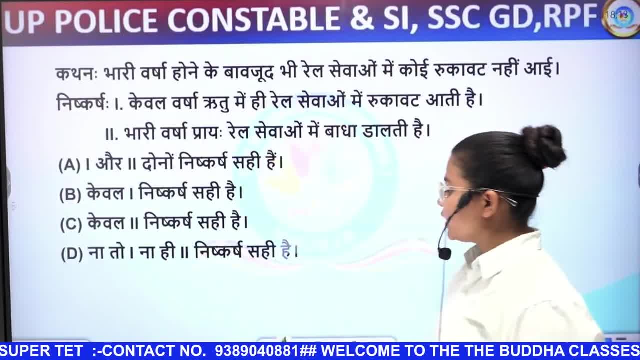 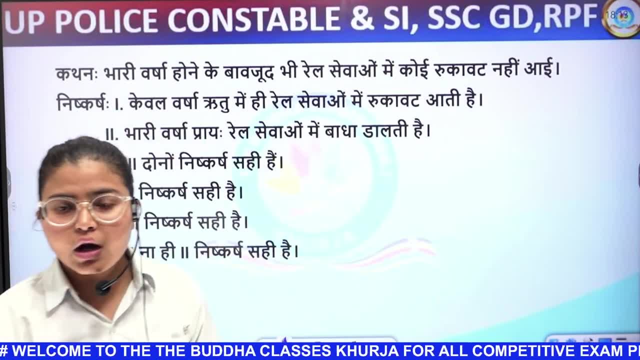 Okay, is it clear? now Go ahead. This is a very important question. This is a very important question. All the questions asked in the previous year are very important for you, friends. Okay, What has been said in this Next question? 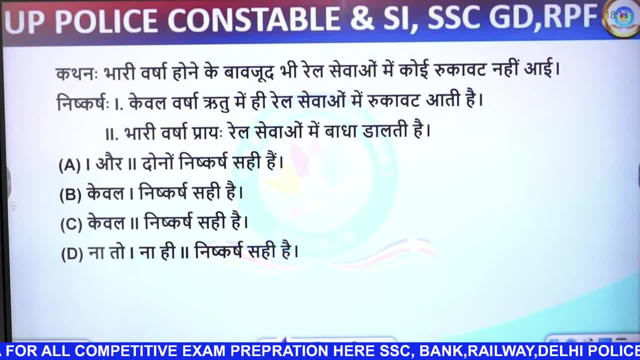 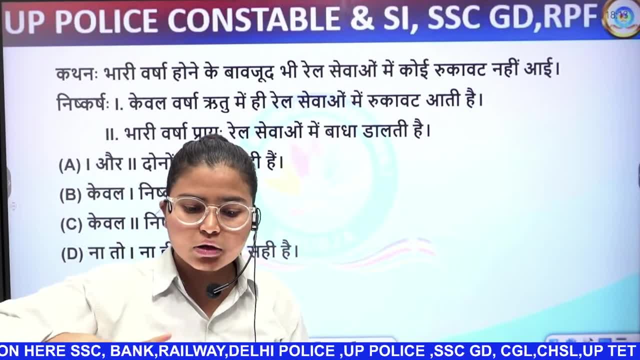 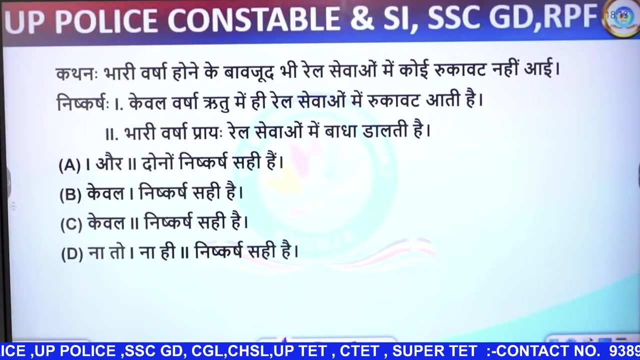 Despite heavy rains, there has been no hindrance in train services. Despite heavy rains, there has been no hindrance in the train that runs. Discuss number 1 is given Only in rainy season. Only in rainy season there is a hindrance in train services. 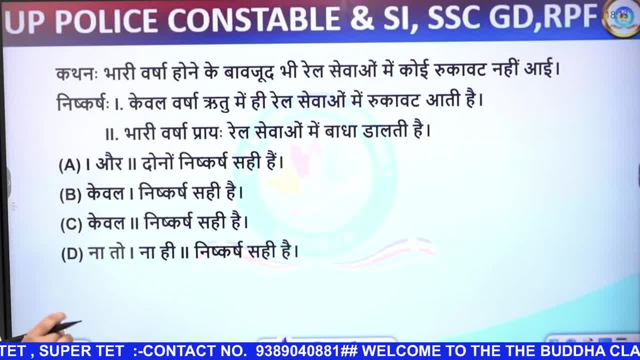 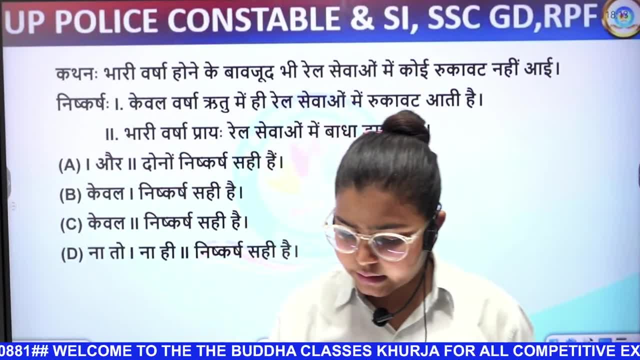 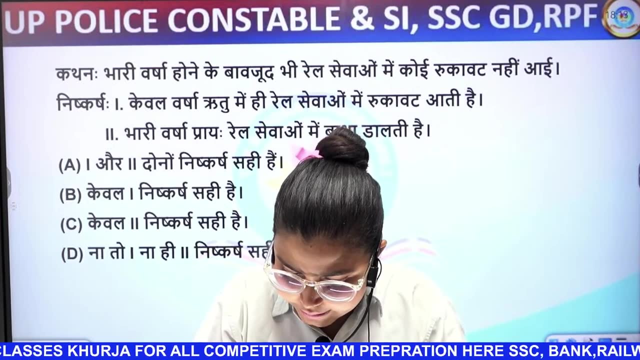 Number 2 is given: Heavy rains put obstacles in train services. Which of these will be correct? Once you tell me which of these will be correct, friends, What will be the correct answer to this? Will someone tell me What will be the correct answer to this? 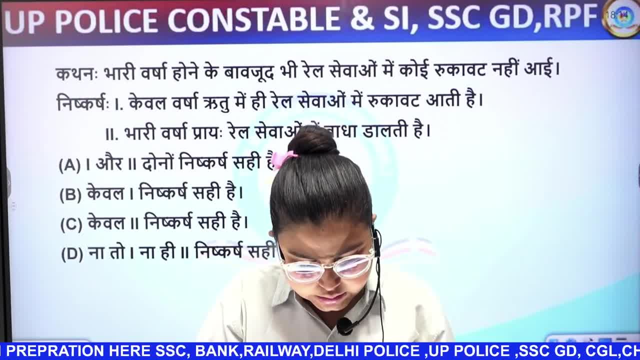 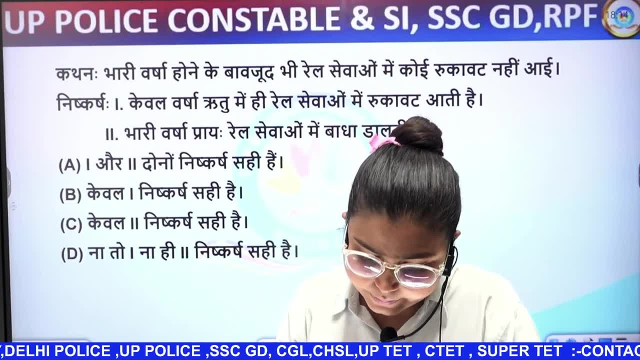 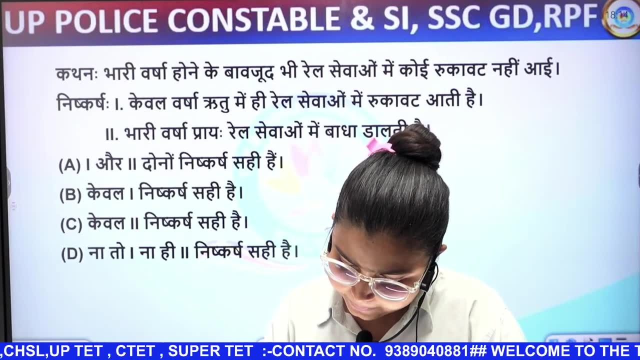 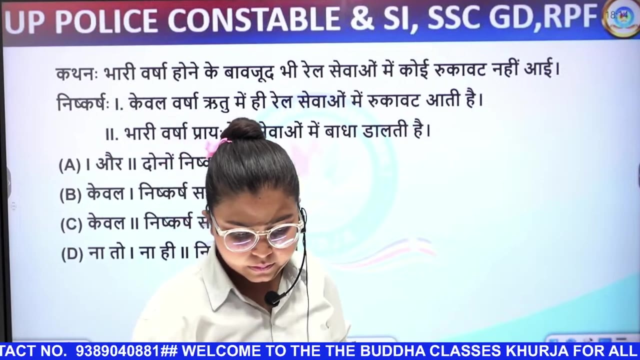 Once you comment the answer quickly: All the friends. What will be the correct answer to this? Will someone tell me Any friend, any brother, or how much did to me this relating to this? what will the right answer to this? will Any friend who should answer like this: 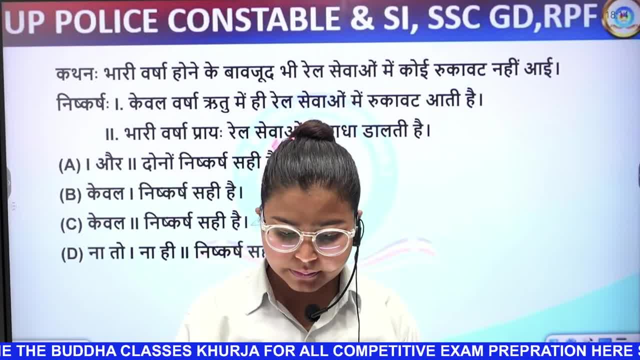 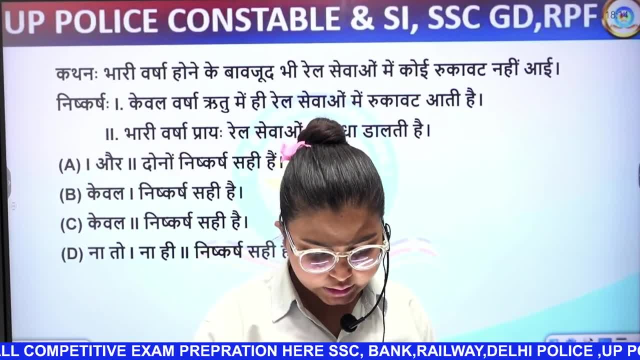 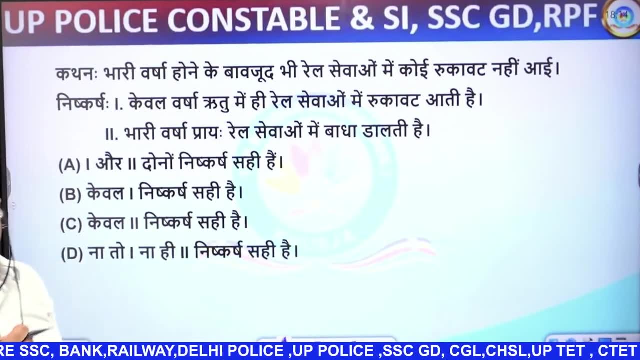 Yes, brother, Will someone tell me, Tell me once, what will be the correct answer for this question? Let's move on to the next question. Let's see once. Let's see, what is said in the question. Friends, what is said in the question is that, despite heavy rains, there are no obstacles in rail service. 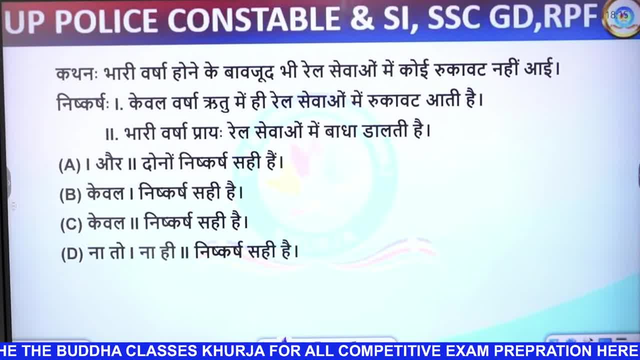 So it has been said that only heavy rains, only in the rainy season there are obstacles in rail service. What has been said, Only in the rainy season there are obstacles in rail service? Or put a ban on heavy rains prior to rail service. 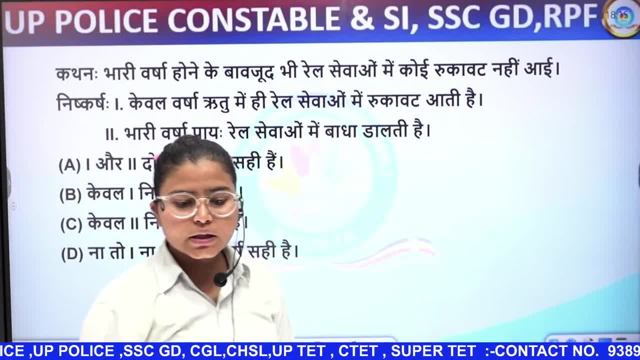 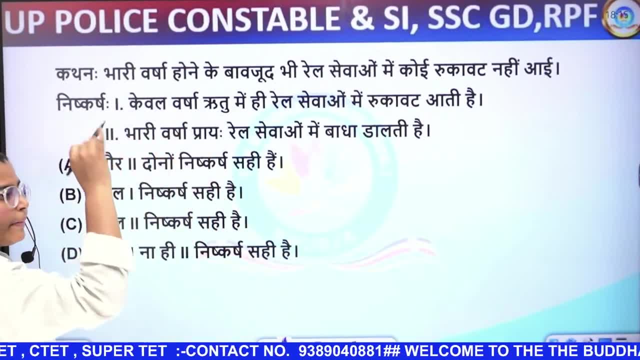 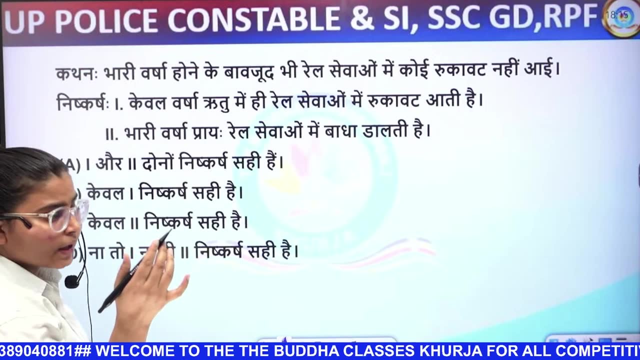 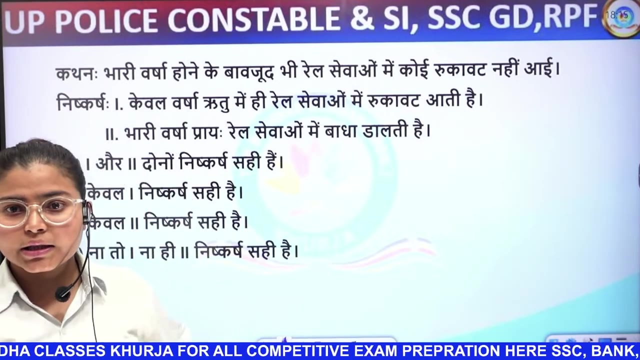 Which one of these will be correct. Both of these will be correct. Why will they be correct? Because when heavy rains happen, there are obstacles in rail service. Because of heavy rains, the tracks become wet And the empty space between the tracks is filled with water. 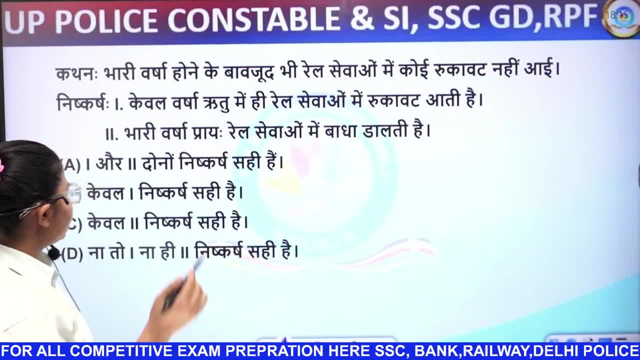 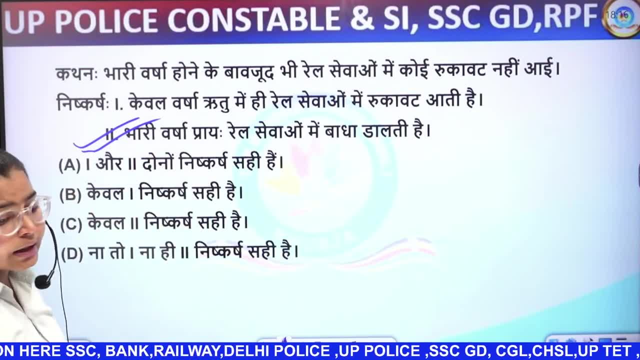 Because of this, there can be obstacles. This is right. This is right. So NISQRS number 1 is correct. There are obstacles in rail service only in the rainy season. It is not that there are obstacles in rail service only in the rainy season. 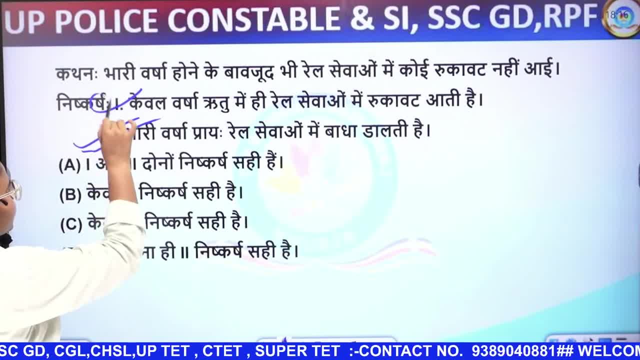 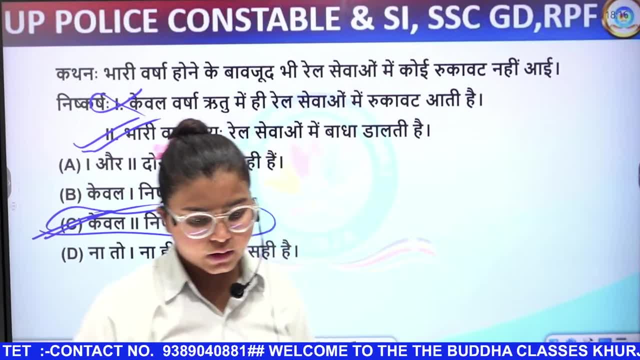 It can happen in the summer as well. We cannot accept this. In this, only NISQRS 2 is correct. Option number C is the correct answer. Okay, Let's move on. Next question: Fashion Clarity. Is there so much quality? 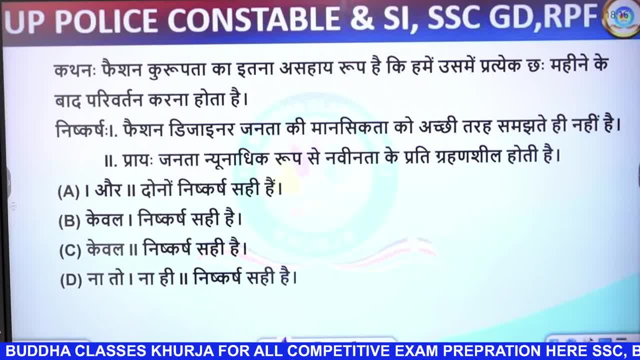 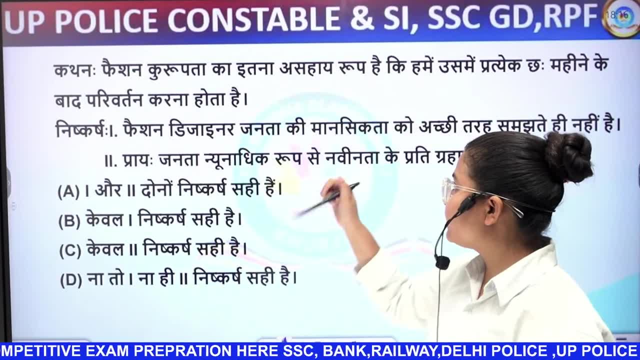 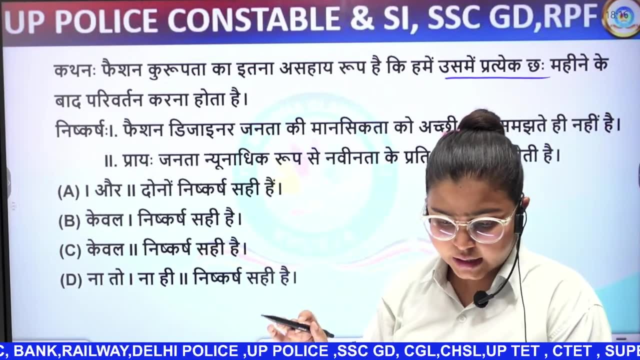 Is there so much quality that we have to change it after every 6 months? Is there so much quality of fashion that we have to change it after every 6 months? Okay, NISQRS number 1 is correct. Fashion designers do not understand the mentality of the public. 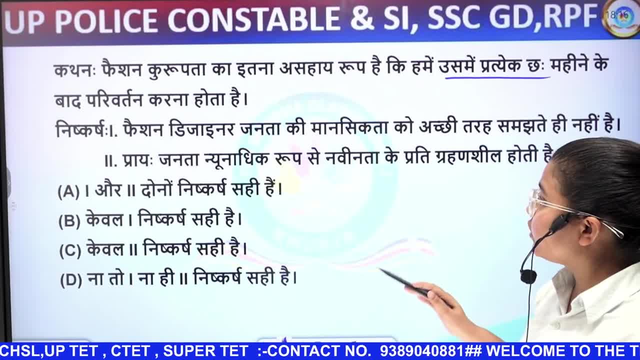 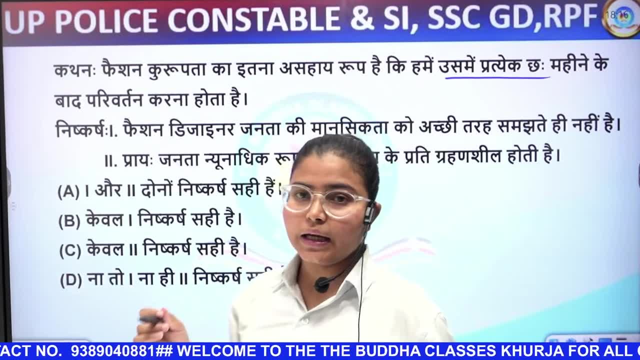 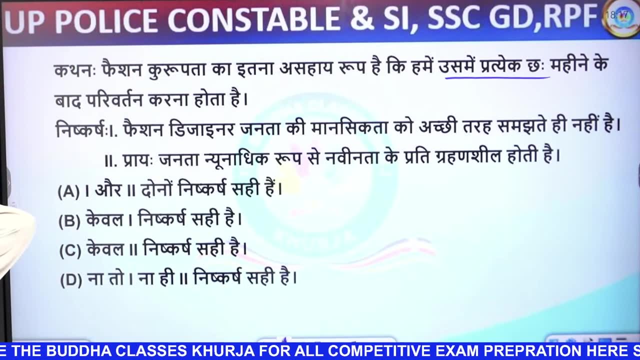 Or is there so much novelty in the public? Fashion designers do not understand the mentality of the public. Which NISQRS will you believe right? Think about it and then answer me. Think about it first and then answer me. What will be the right answer? 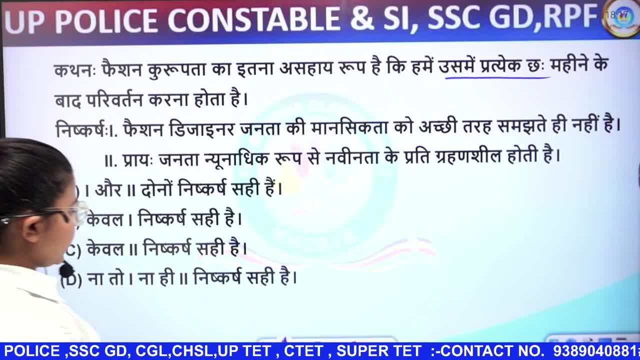 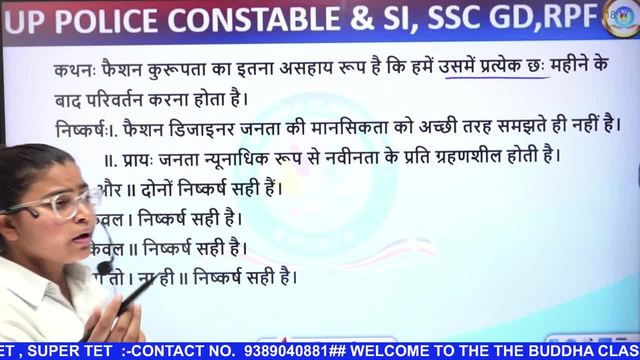 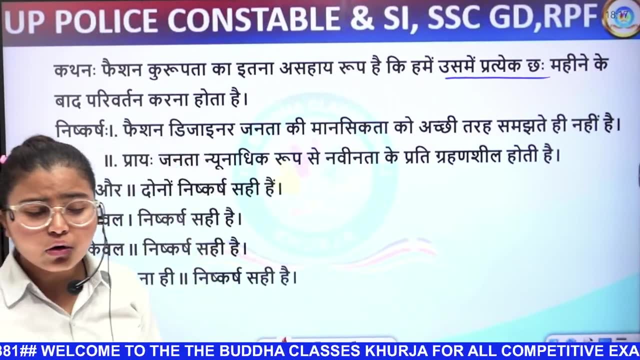 What is the correct answer to this question? Pay attention to what has been said in this: That after every six months, a change has to be made. In this, the change has been given the number first. Do fashion designers not understand the mentality of the people? 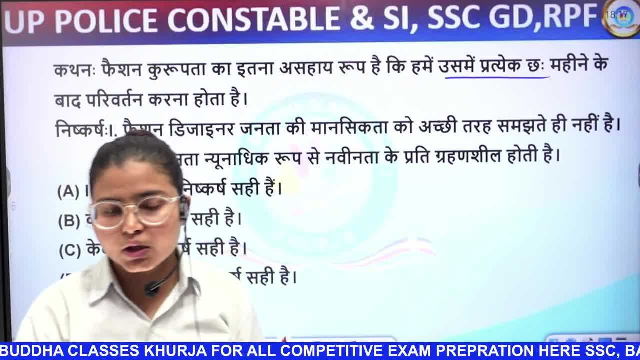 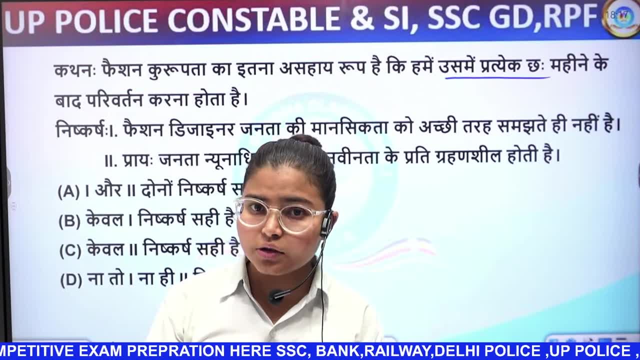 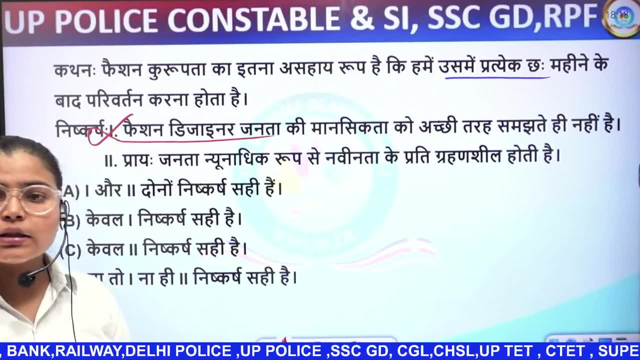 It is not that they do not understand the mentality of the people. If they do not understand the mentality, then there is no pressure of changes. So the first question is wrong. Fashion designers understand the mentality of the people very well. That is why changes come. 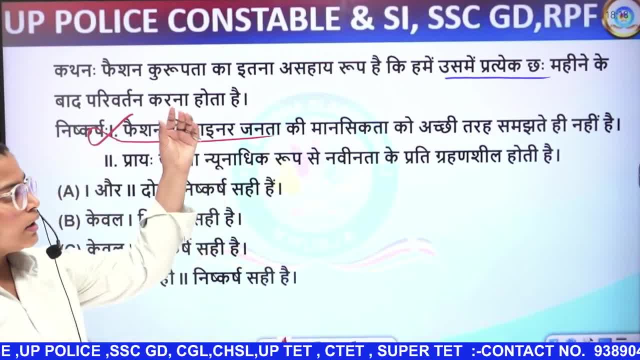 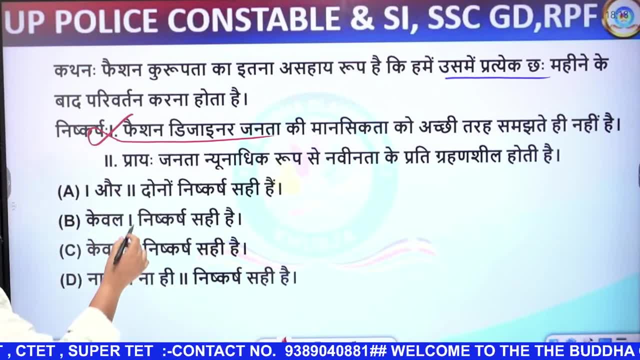 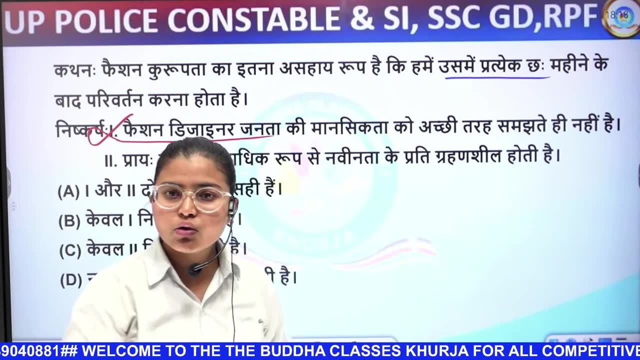 That is why changes come. If they do not understand the mentality of the people, then there is no option of change. Okay, The general public is very sensitive to novelty. Does the public always look for new things? This is fine. That is why there is no pressure of changes. 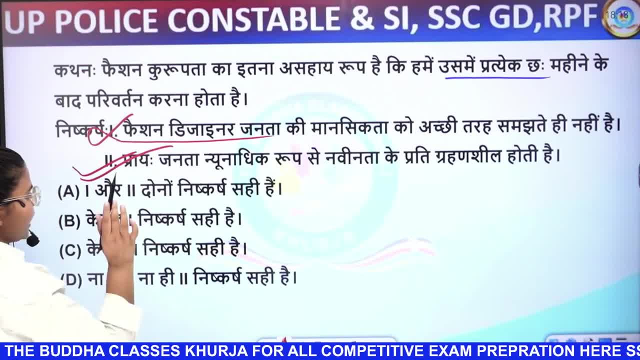 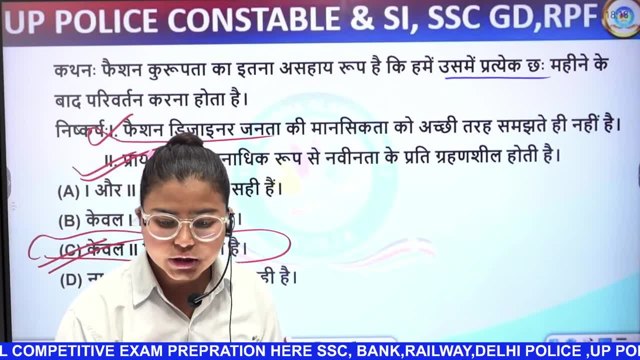 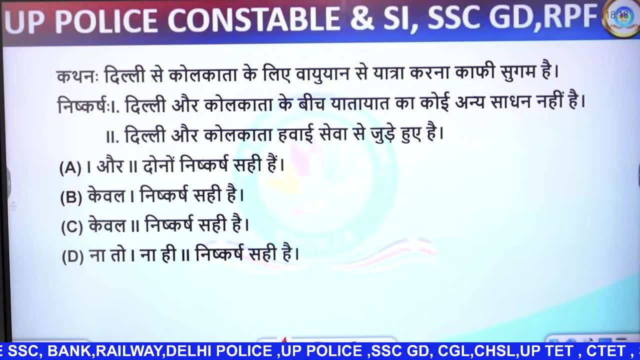 Okay, Then this next question, question 9.. Question number 9 is correct. Its response will be correct As per its suggestion. it doesn't matter if it is the answer of the question number, but if the answer of the question number am stroeshhru. 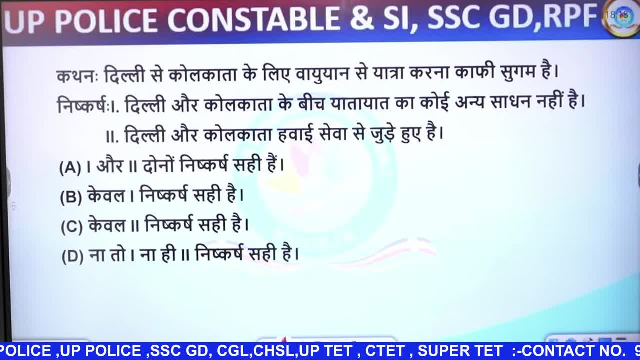 is correct, because the 저기 appears to be correct, then I will accept the question. Alright answer, for that will be correct. There is no agreement between Delhi and Kolkata. Delhi and Kolkata are connected by air service. What will be the correct answer? 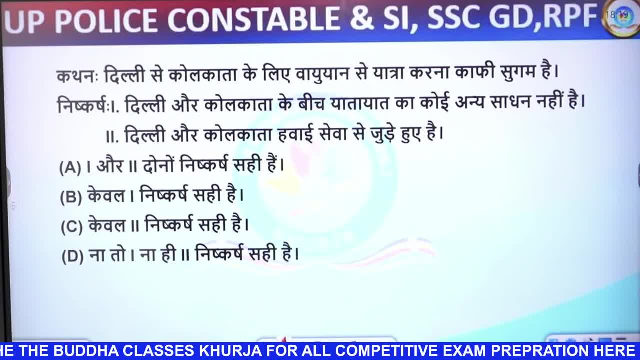 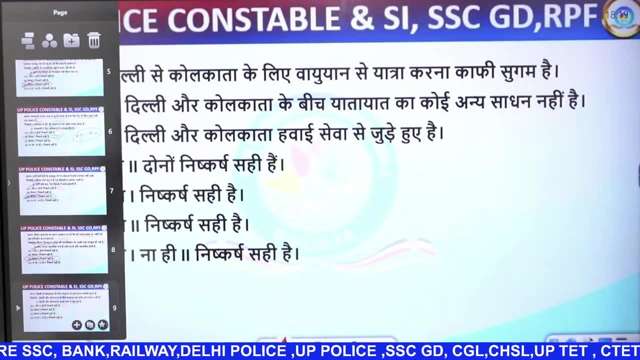 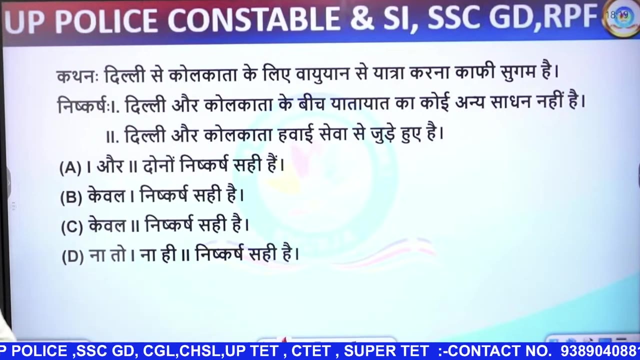 You have to tell the correct answer What will be the correct answer. We will tell you quickly what will be the correct answer. What will be the correct answer? We will tell you quickly What will be the correct answer. It is said that it is easy to travel alone from Delhi to Kolkata by air. 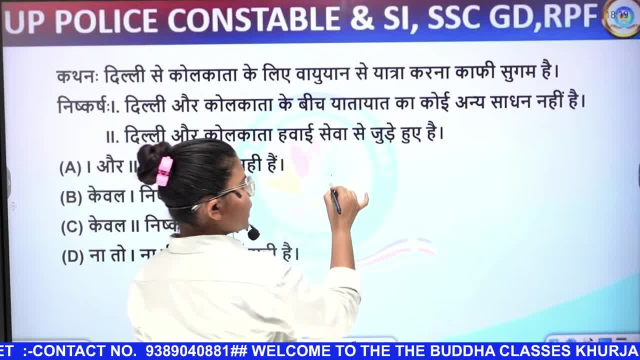 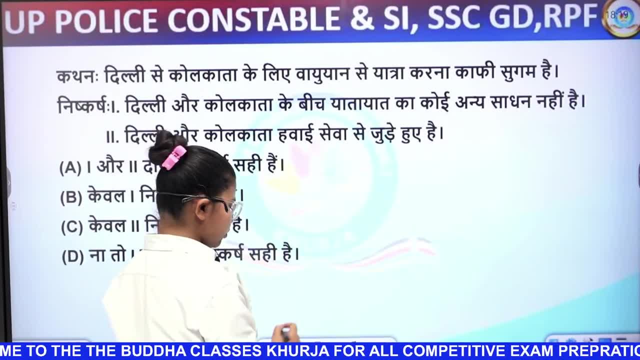 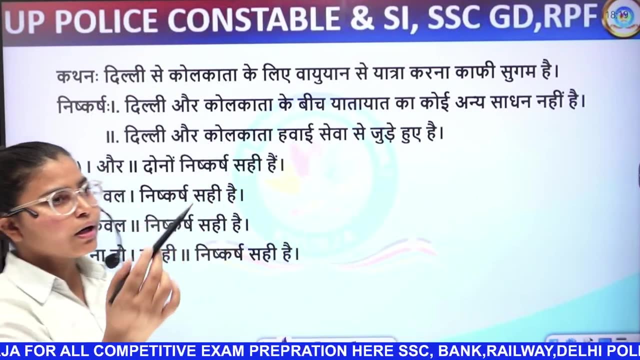 Yesterday, I told you a question To go from Delhi to Agra. I told you the question: from Delhi to Agra. Think about this question accordingly. Think about this question. It is said that it is easy to travel alone from Delhi to Kolkata by air. 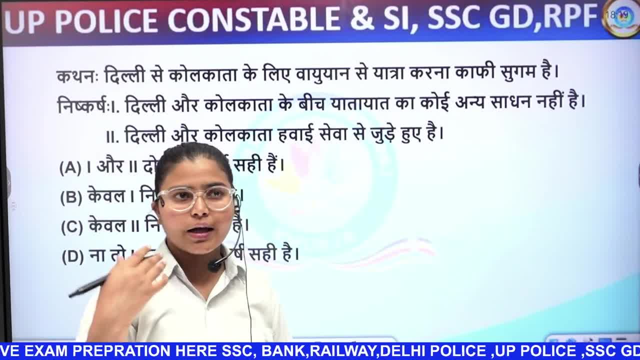 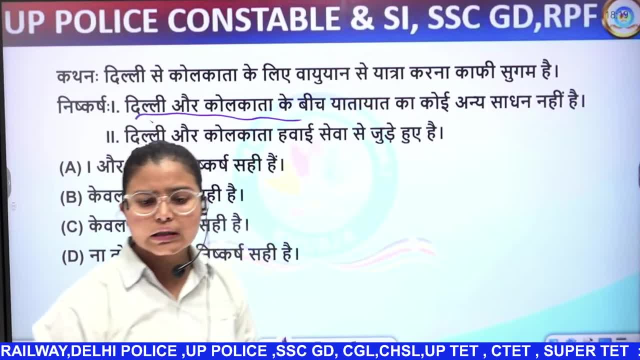 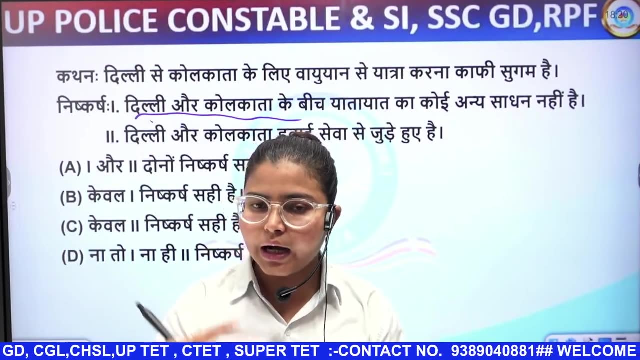 It means easy. It means easy, It means fast. In this we have given the first thing. There is no agreement between Delhi and Kolkata. Is it possible that to travel with air there is no other alternative? We can't say this. 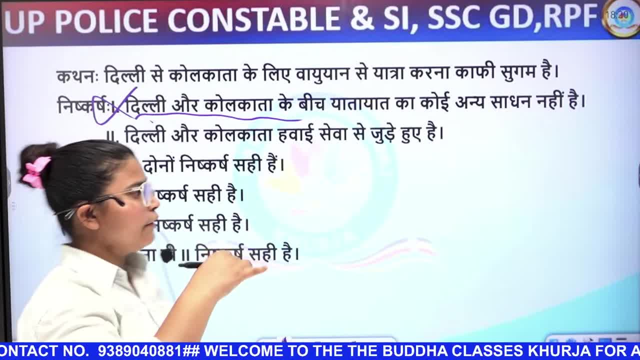 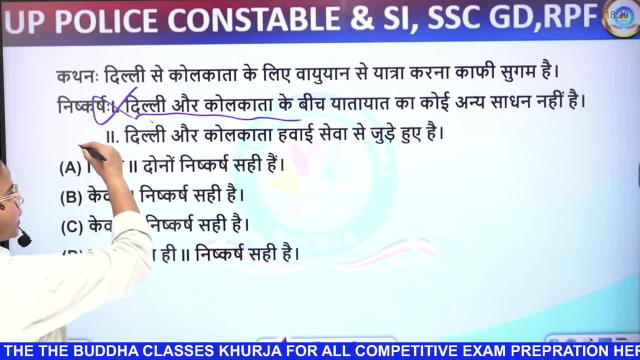 This is wrong. Delhi and Kolkata are connected to the air services. Yes, Delhi and Kolkata are connected to the air services. This is why it is possible to travel with a baiu yarn. This is why it is the correct answer. Only two miscalculations are correct. 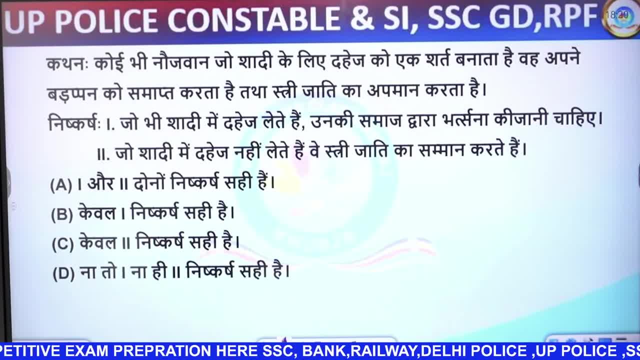 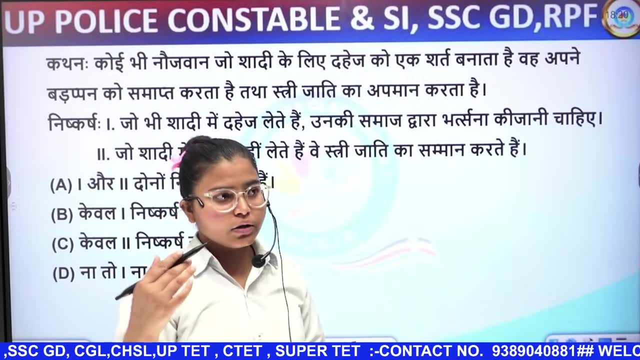 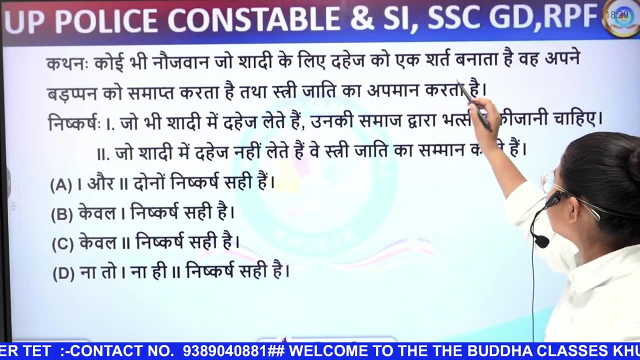 Option number C. Next question: It is said that any young man who considers dowry as a condition for marriage, he ends his adult life. He also insults the women's caste- Any young man who considers dowry as a condition for marriage. 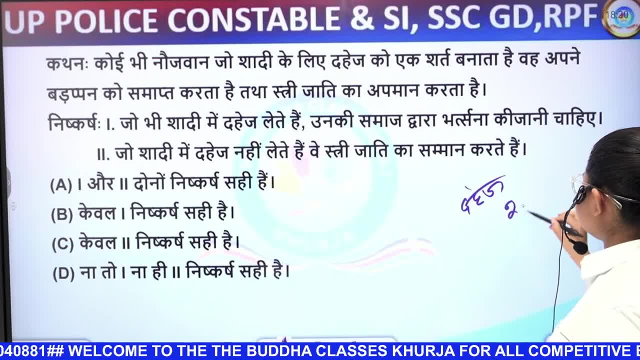 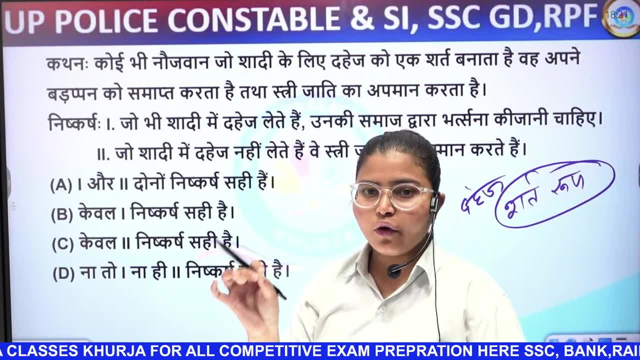 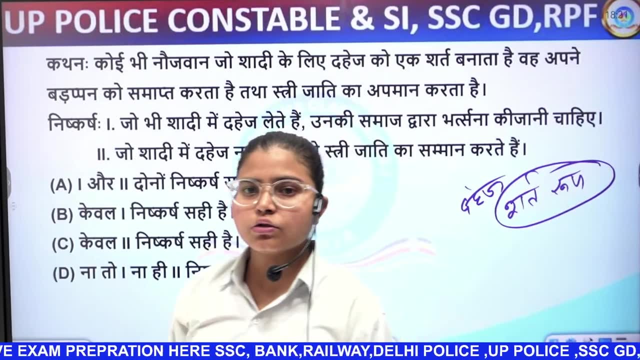 considers dowry as a condition. He considers it as a condition. He thinks that he will marry only when he is fortunate. This is a condition. He has a condition that he will marry only when he is fortunate. If it is a condition, then I will not marry. 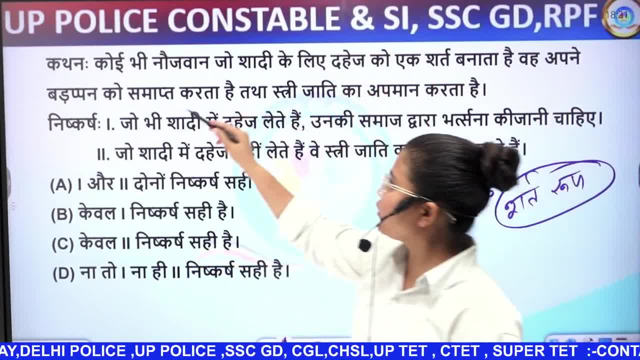 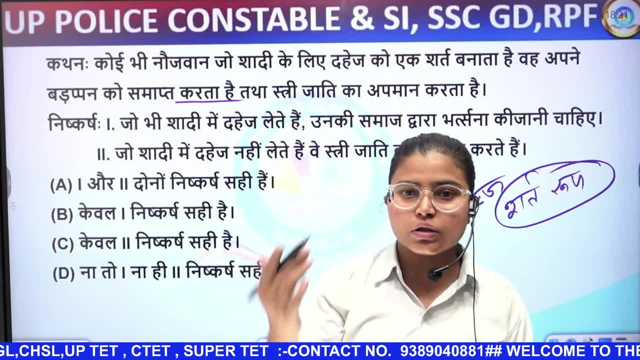 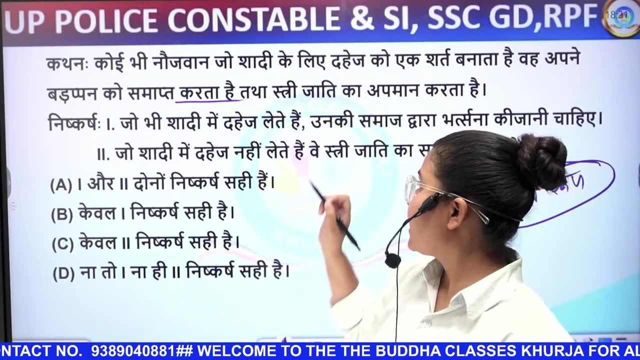 Next question: He ends his adult life, The attitude and adult life which should be there in him. He ends it by considering it as condition for dowry. Next question: He insults the women's caste. He insults the women's caste in dowry. 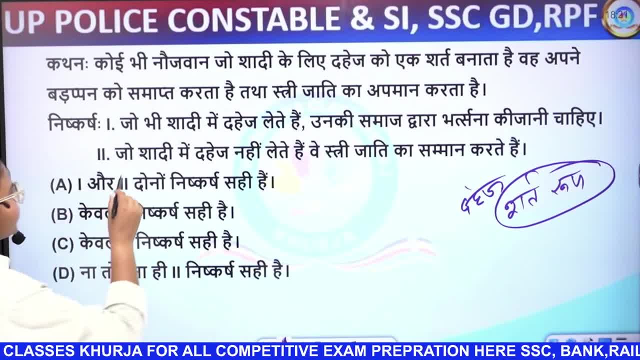 This question was asked in the question Discourse number 1 is given. What is the correct answer to this question? What is the correct answer to this question? What is the correct answer to this question? See this quickly. What is said in this? 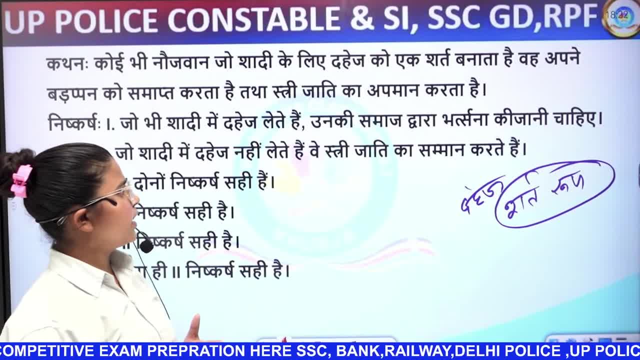 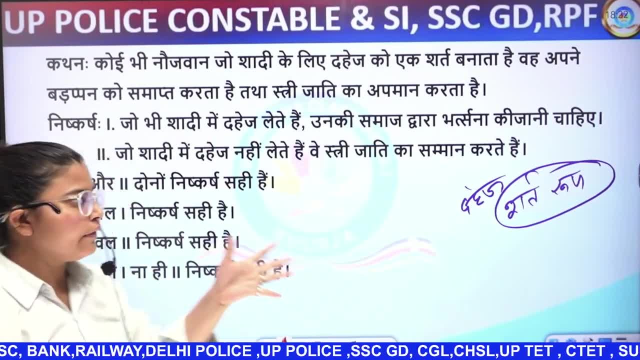 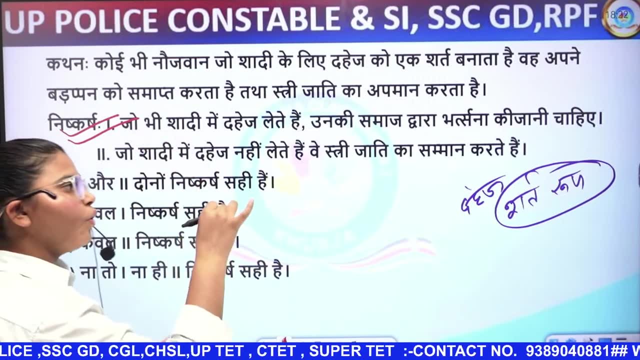 What is said in this: Whoever takes dowry in marriage, he should be respected by his society. Yes, he should be respected by his society. This is the correct answer. Yes, this should happen. This is the argument that should be done by society. 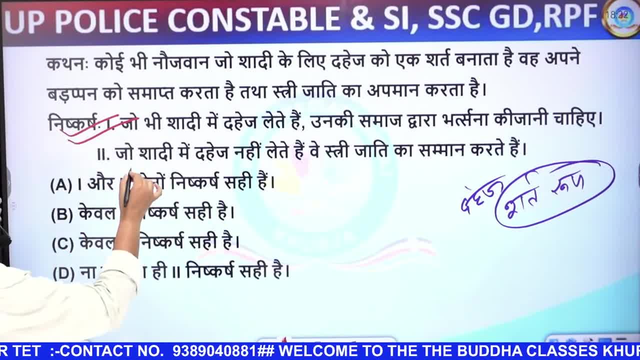 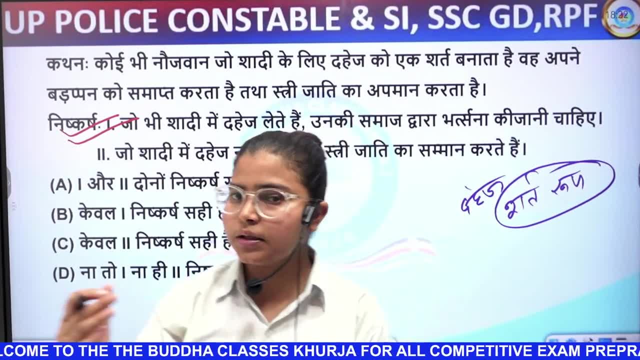 This is the argument of the Tarkh Sangat. Then it is said that those who do not take dowry in marriage they respect the women's caste. Marriage can be said that they respect the women's caste, so they do not take dowry. 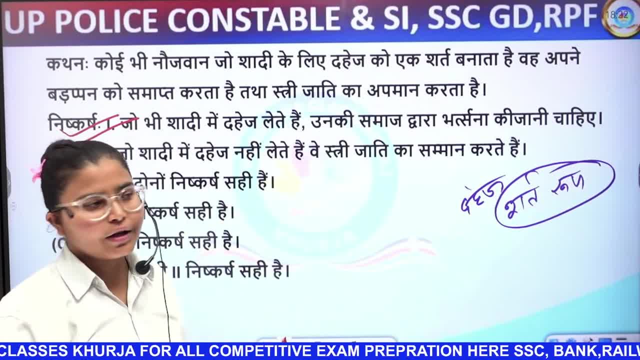 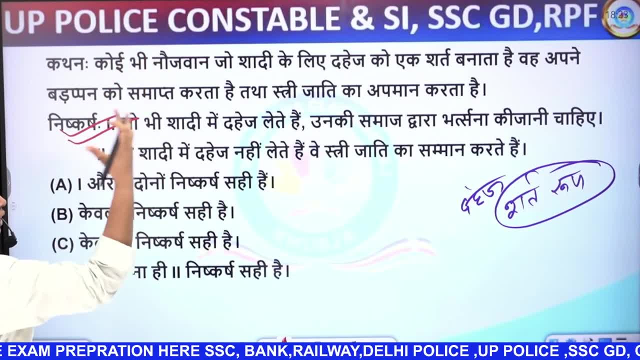 Later, no matter how much they hit the woman, it does not matter. So both things are based on Tarkh. Tarkh is based on the Tarkh. Tarkh is based on the Tarkh. Tarkh is based on the Tarkh. 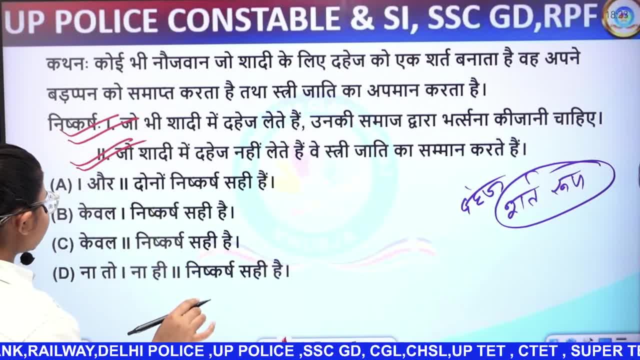 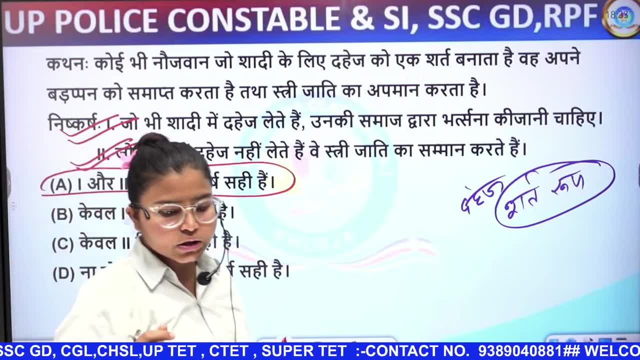 So both things are based on Tarkh. What will be the correct answer to this? Both Niskars are correct. Tarkh Sangat is the correct answer. How do both Niskars come out? Both Niskars are Tarkh Sangat. 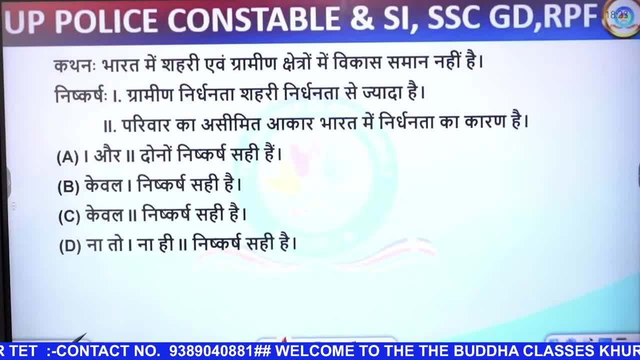 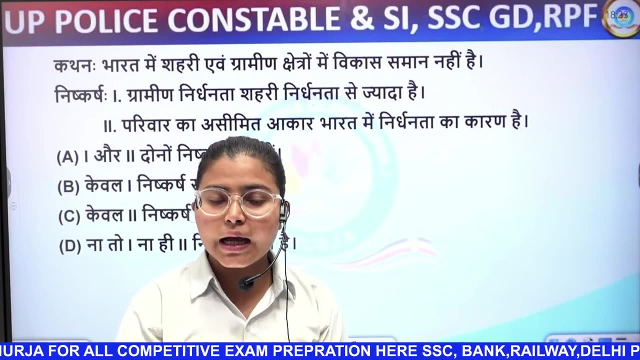 Option number A is the correct answer. Option number B is the correct answer. Next question: In India, development in rural areas and rural areas is not the same. It is said that in rural areas and urban areas development is not the same. 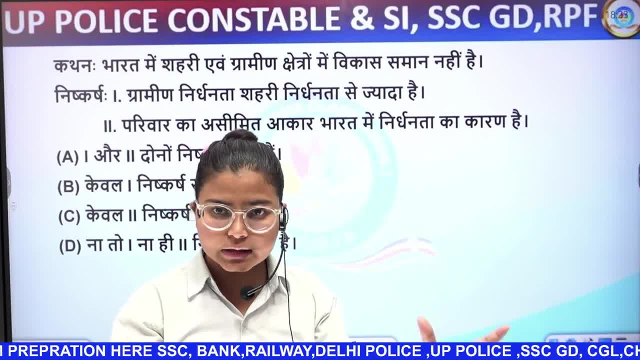 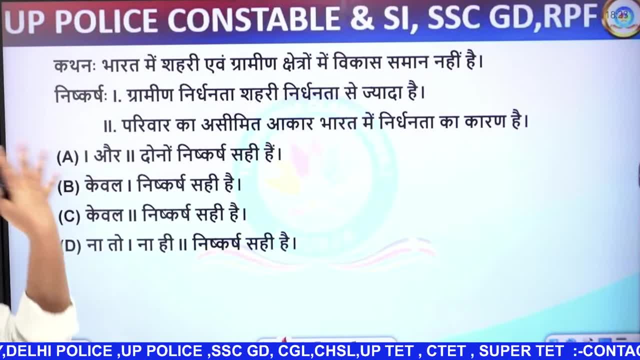 Development is happening in villages and something is happening in the city. There is no equality in both. Discourse, number 1 is given. The rural economy is more than the urban economy. The urban economy is more than the urban economy. The rural economy is more than the urban economy. 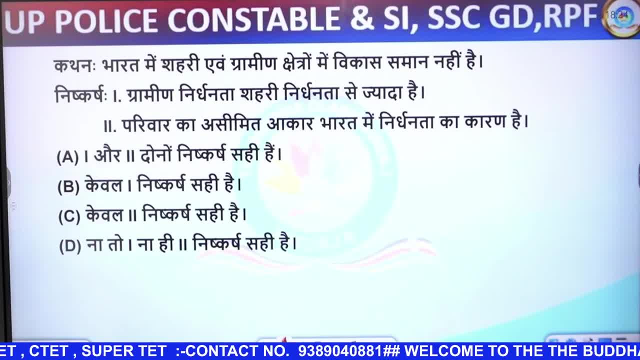 Discourse number 2 is given. The limited size of the family is the reason for the unemployment in India. What will be the correct answer to this? You will tell us quickly what will be the correct answer to this. friends, Please comment once on the correct answer to this. 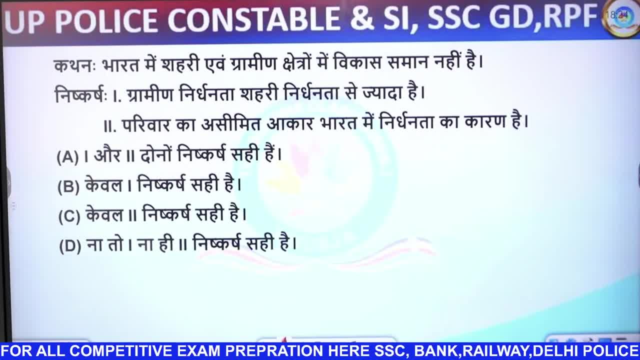 What will be the correct answer to this? What will be the correct answer to this? Look at this, Look at this: The rural economy is more than the urban economy. Is there more unemployment in the village than in the city? We cannot say that. 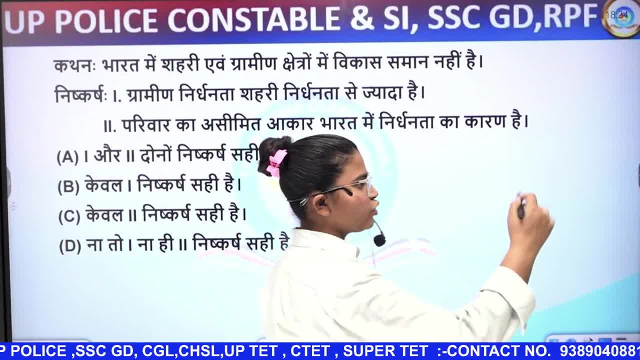 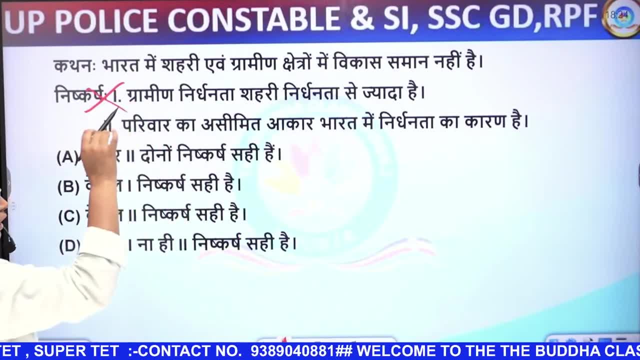 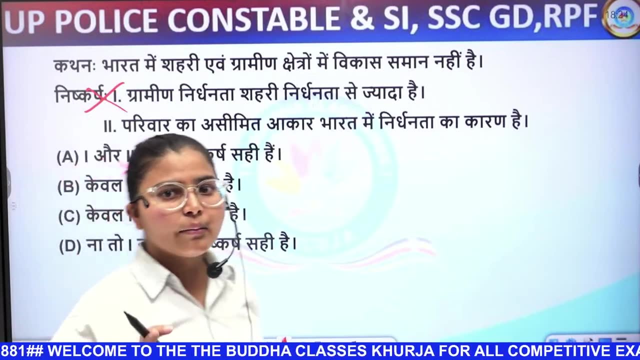 Why can't we say that? I have seen that there are very big people in the village who are not even in the city. So the first discourse is wrong. The limited size of the family is the reason for the unemployment in India. The limited size of the family means that 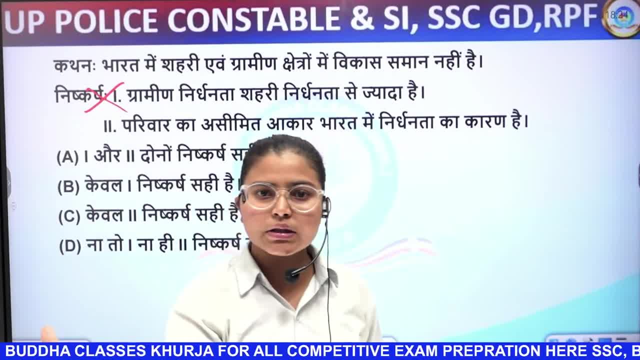 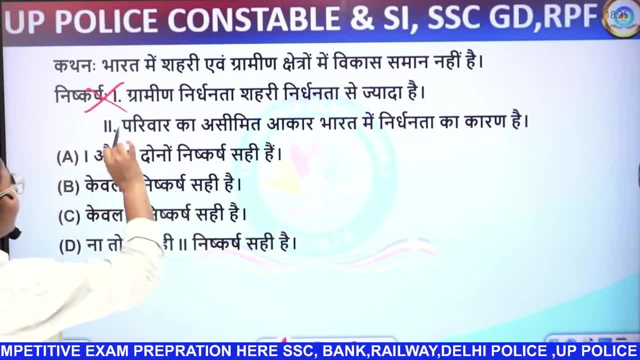 there are more people in the family, Isn't it? There are more people in the family. What is the reason for the unemployment in India? We can't even say that it is the reason for the unemployment. Discourse number 2 is also wrong. 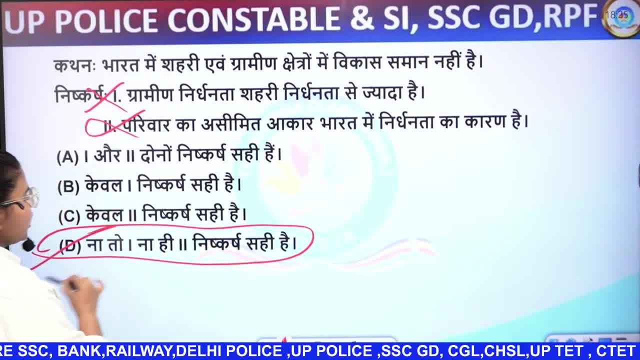 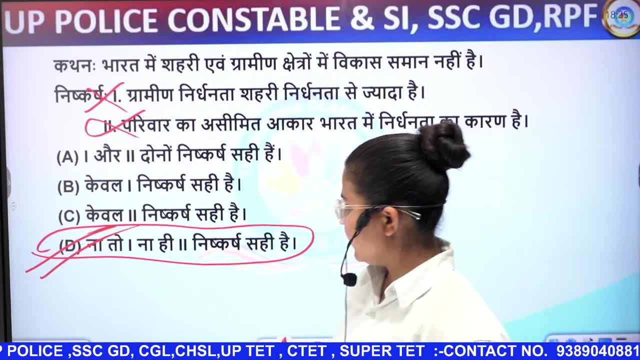 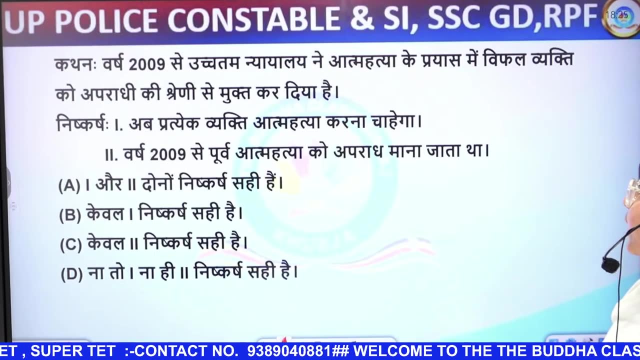 The correct answer to this is option number 2.. Neither is the first discourse right, nor is the second discourse right. None of the discourses are right. Okay, Look at the next question In 2009,. in the Supreme Court. 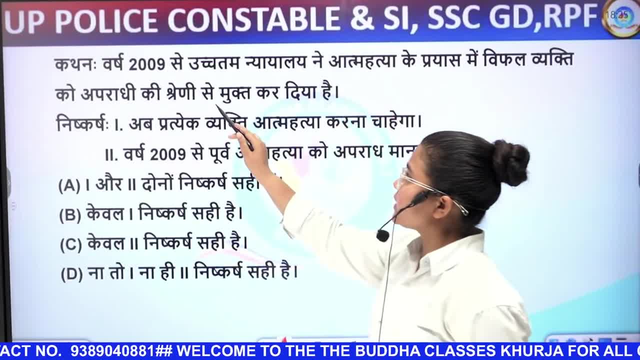 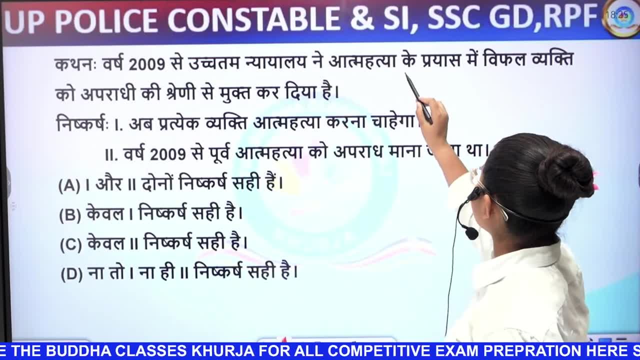 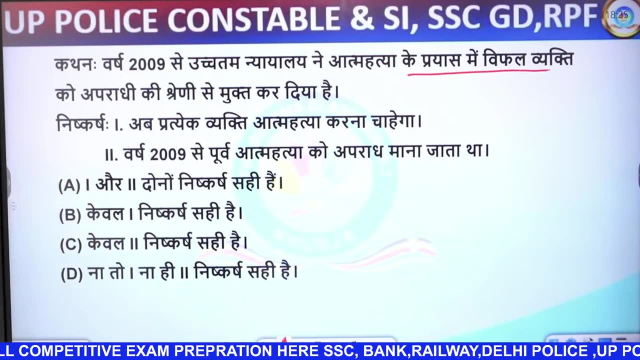 in the attempt to commit suicide. a failed person was released from the prison of crime. The question is from 2009.. In the Supreme Court, a failed person was released from the prison of crime. The person who commits suicide, the person who is a failed person. 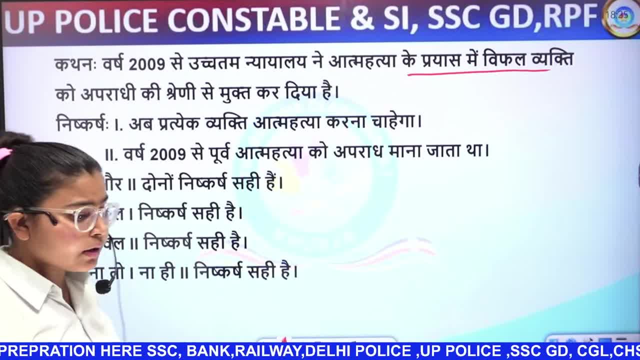 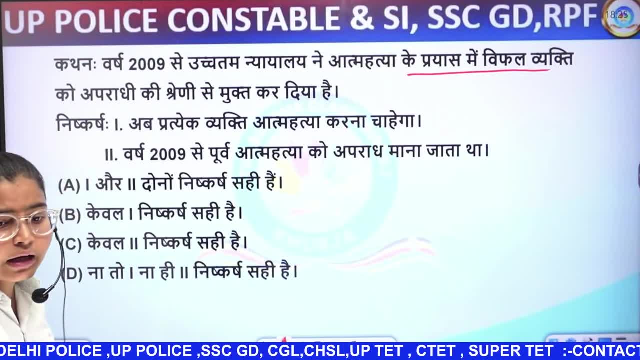 the person who is released from the prison of crime will not be considered a criminal. The person who is committing suicide, he is failing The person who is committing suicide, he will not be considered a criminal. Discourse number 1 is given. 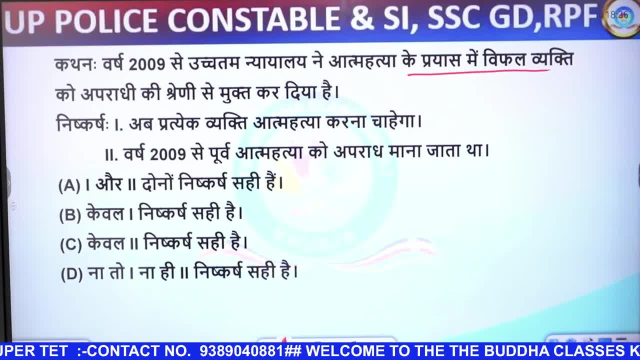 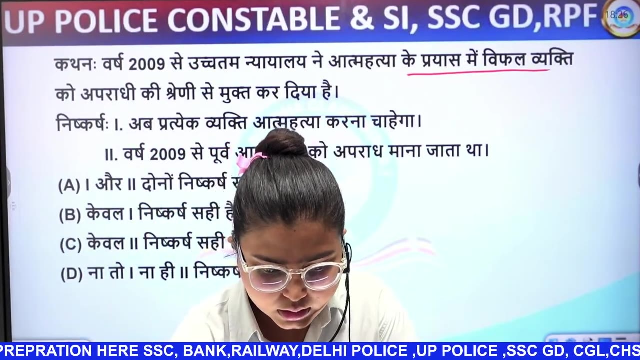 Now every person should commit suicide. Discourse number 2 is given In 2009,. suicide was considered a crime. Which discourse is right? You have to tell this. See what is in it, Friends. it has been said. Thank you, sir, thank you. 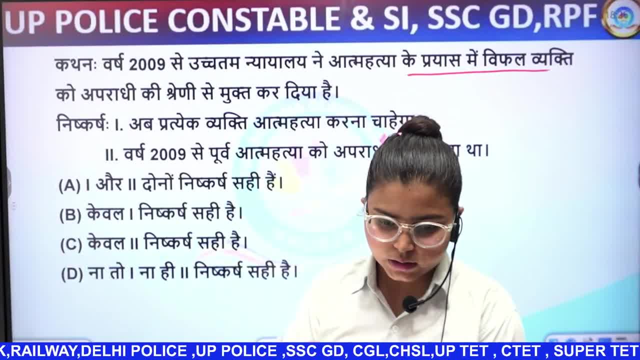 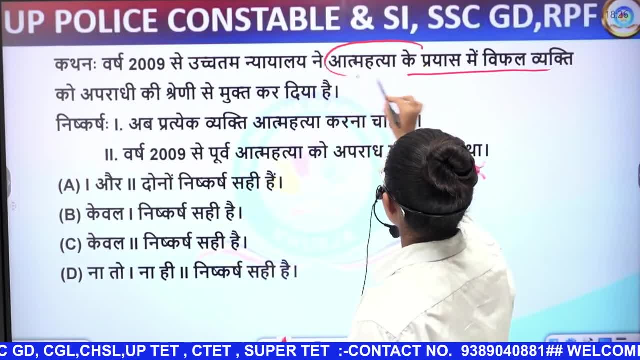 Manoj, Manoj ji. thank you. Thank you so much. See what has been said in it. It is about the Supreme Court In the attempt to commit suicide, a failed person. someone is committing suicide. That person is failing in it. 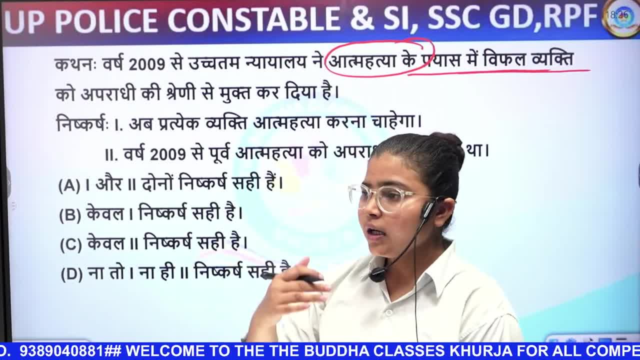 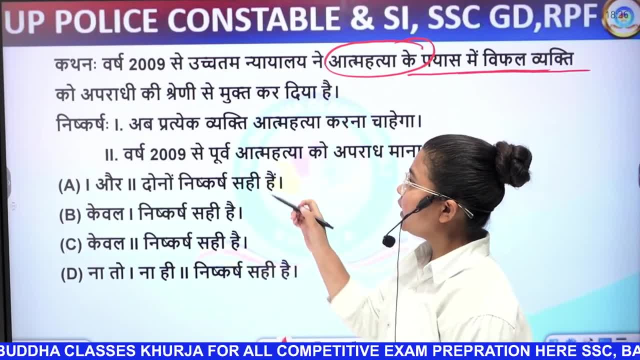 That means he is not being able to commit suicide, So he is not considered a criminal. He is not being cleared out of prison. That's why he is being freed from the prison. Discourse number 1 is given When a person with a disability. 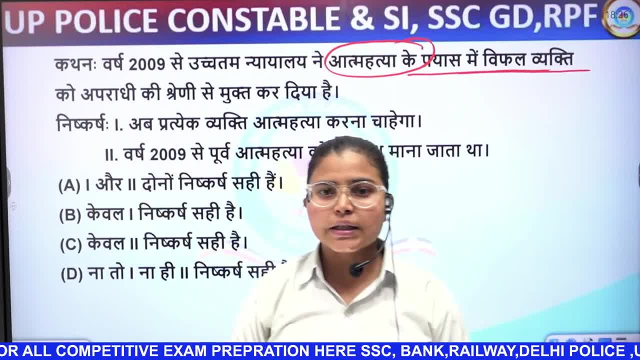 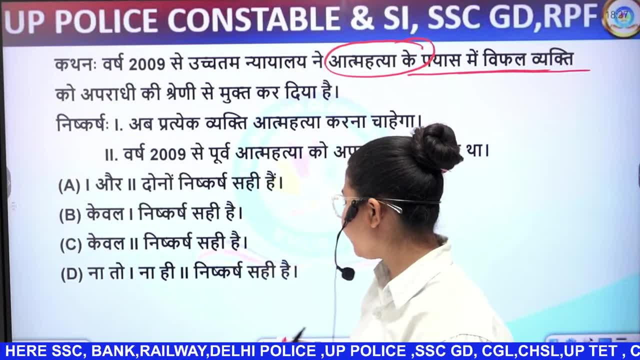 wants to commit suicide. it is not written on someone's face Why he will commit suicide. He is not bothered by his life. He is not bothered about his life. What will happen to him? why will he want to bother about his life? 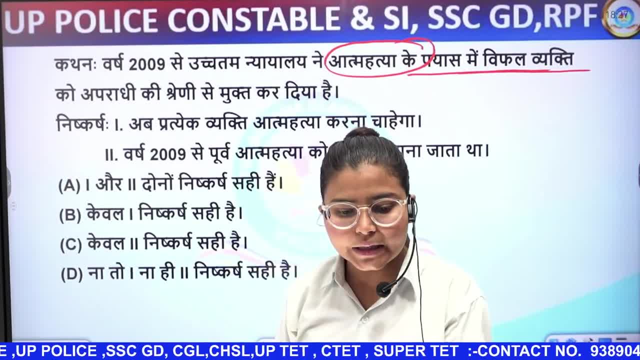 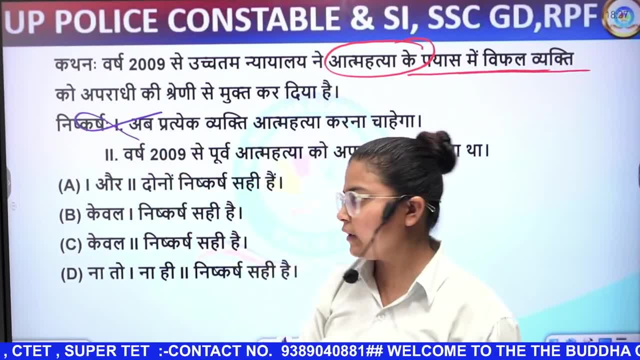 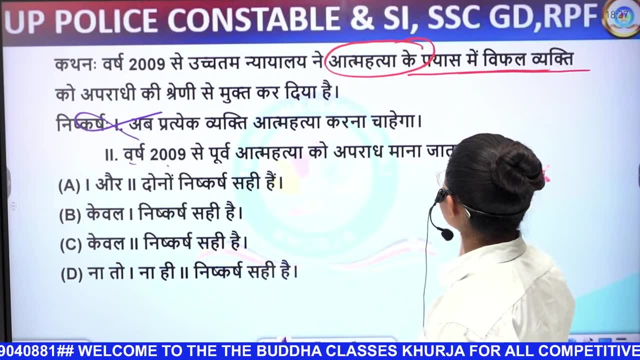 But not every person will do it. Every person, meaning of everyone, will not want to commit suicide. Discourse number 4 is given. Discourse No 1 is wrong. It states that in 2009, suicide was considered a crime. 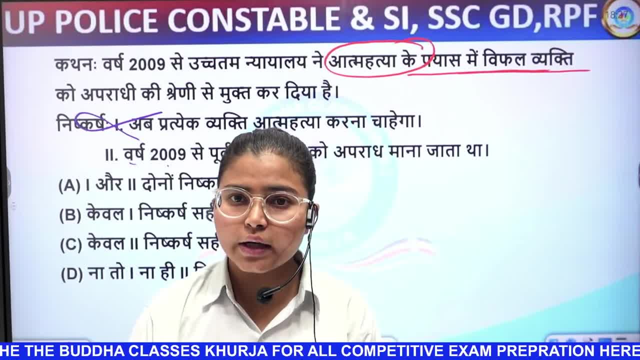 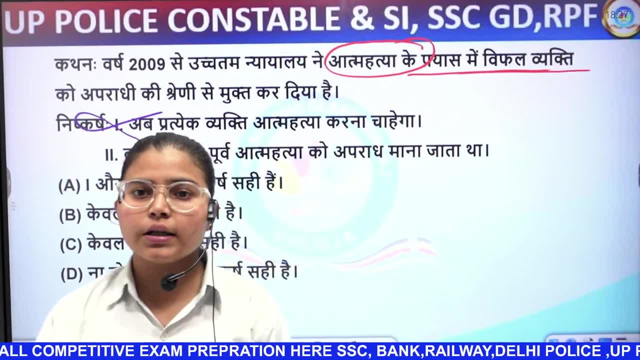 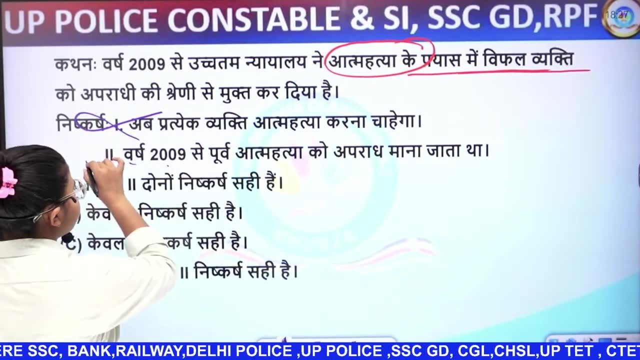 We can say that after 2009,. the Supreme Court has released the person who committed suicide. This means that before 2009, suicide was considered a crime. Discourse No 2 will be absolutely correct. The correct answer to this is that only two discursions are correct. 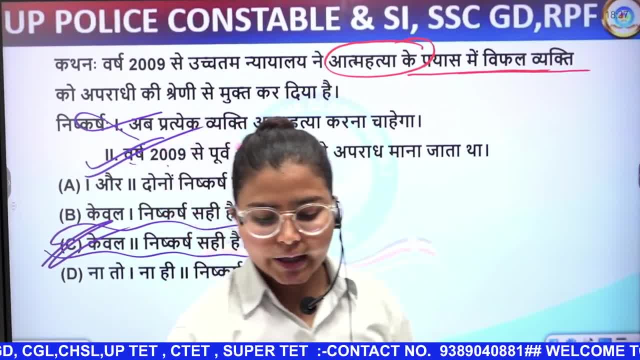 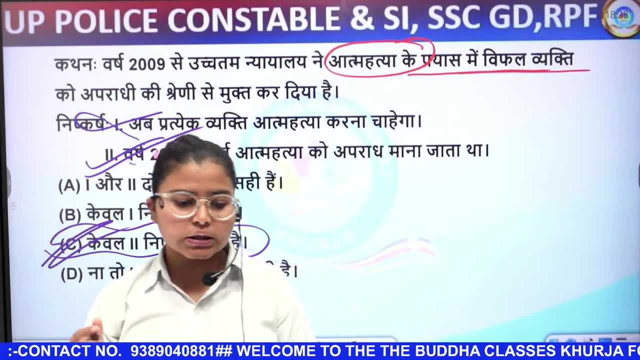 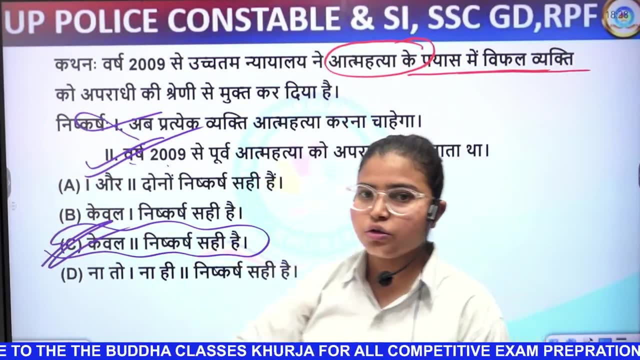 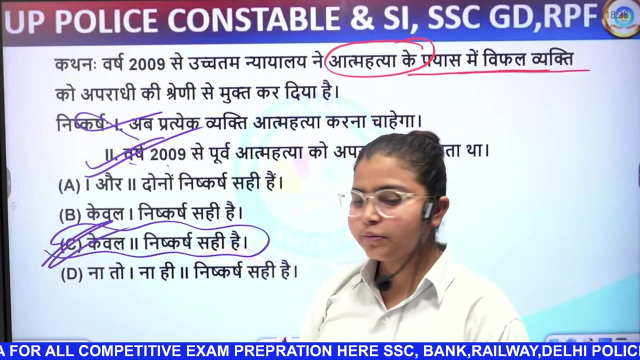 Option No C is the correct answer. Please tell everyone that. do you understand what I am saying? I have asked you 11 questions. If you have any doubt, please put it in the comment section. I will tell you. Option No C. 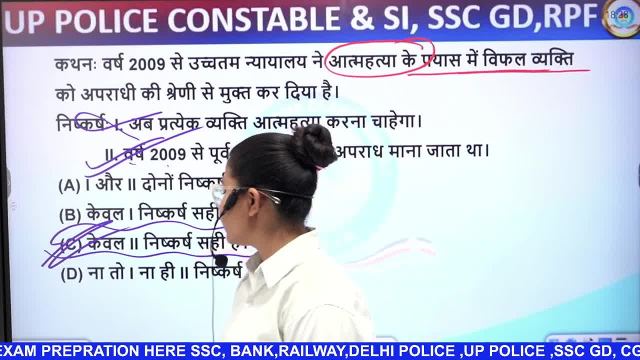 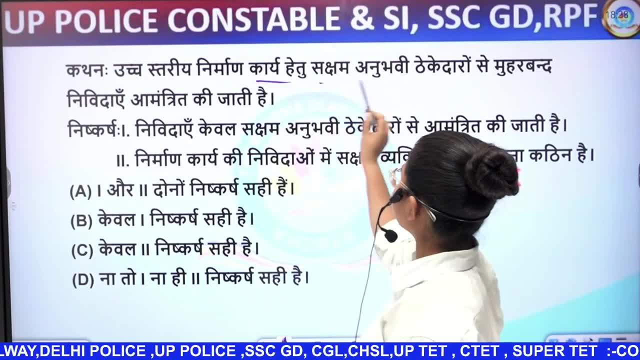 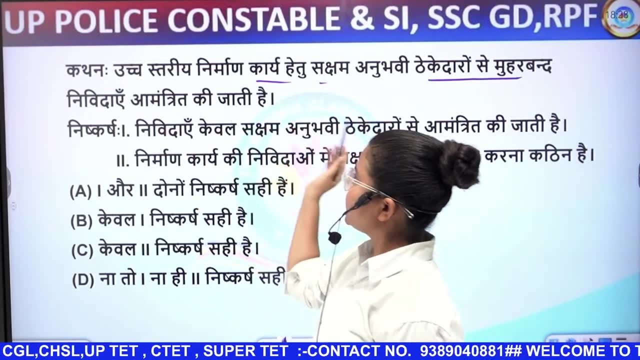 Mr Manoj, you have given a very good answer, Very nice. Next question. The question is that some women are invited to the Moharvand Nividaay by a professional contractor. Moharvand Nividaay are invited to the Moharvand Nividaay. 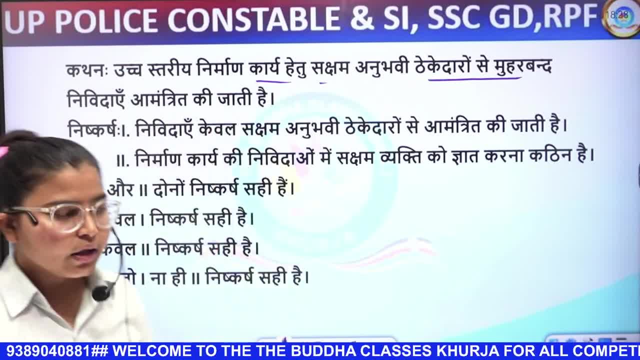 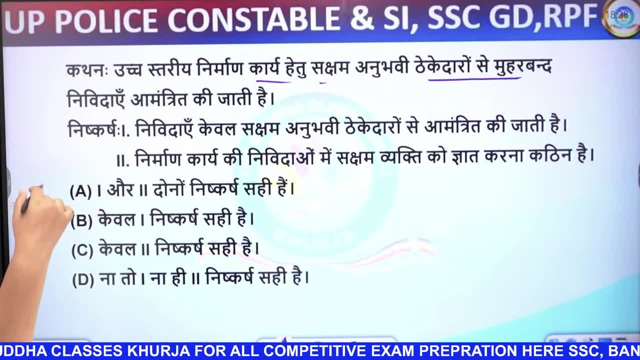 I can understand Very good. Discourse No 1 is correct. Discourse No 1 is correct. Discourse No 1 is correct. All policies areinchеня in Moharvand, Nividaay. Only competent private PATs are invited. 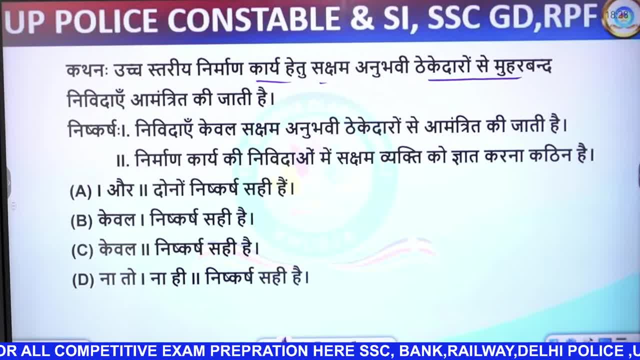 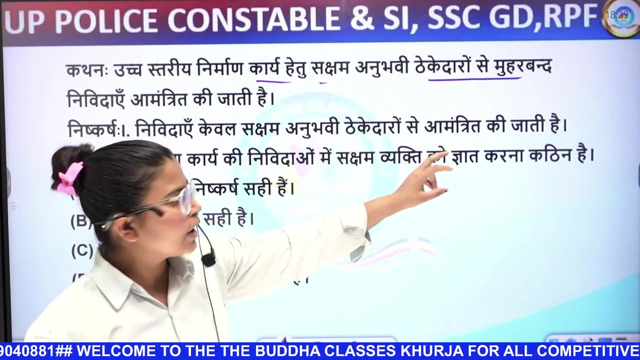 Discourse No 2 is called 크리에 거죠. Correct What is correct. It'sucks. We will comment on the answer. we will see here. we will understand. first we understand the meaning of Muharband and Nivida. 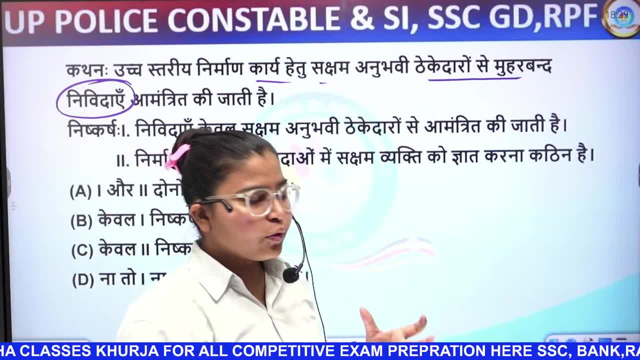 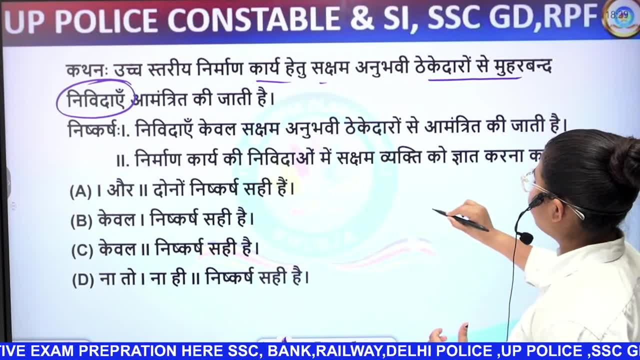 What is the meaning of Nivida? Who is called Muharband and who is called Nivida? Look, it is said in this that a high level of construction is being done. some high work is done. high work is done. 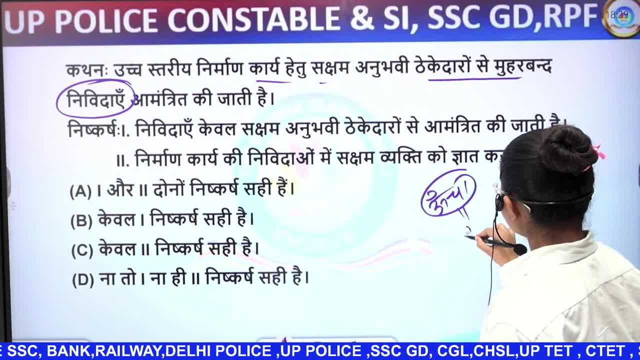 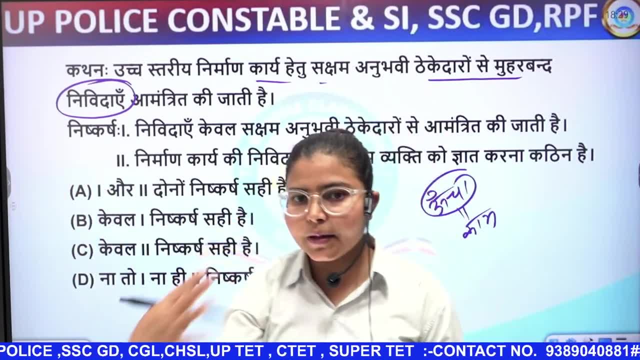 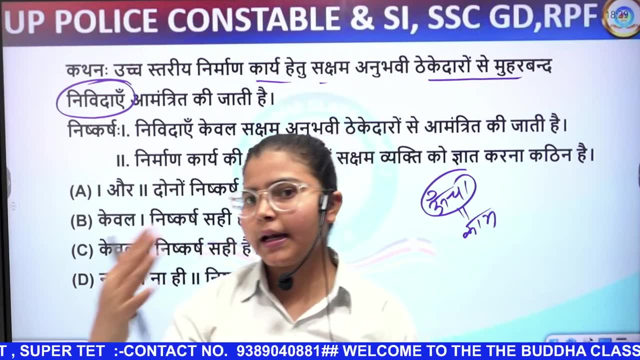 Like we said, high work is done Somewhere. there is a very high level of construction. I have understood that no one has ever gone there. it is a waste, And there it is said, it is said to the common man that you have to take out the highway here. 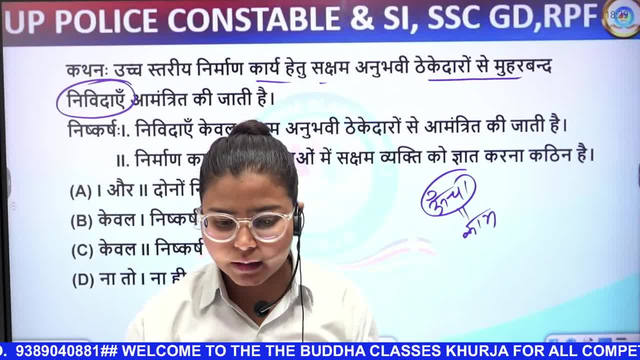 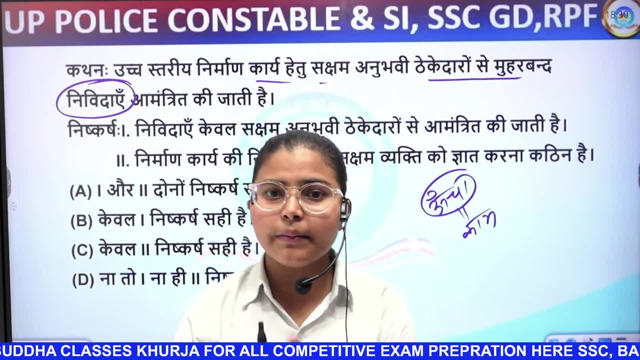 Will the common man be able to do this work? He will not be able to do it. Why will the common man not be able to do this work? Because he has never done it in such places, in such an atmosphere. He has not seen it. 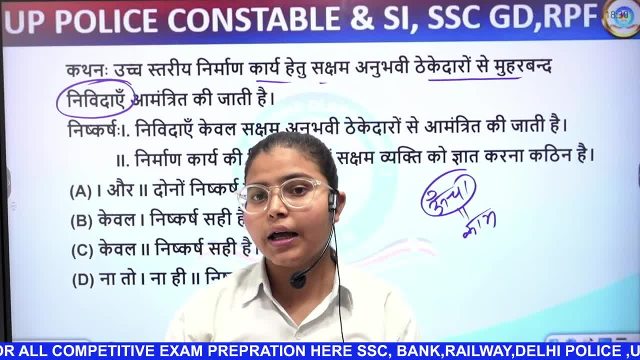 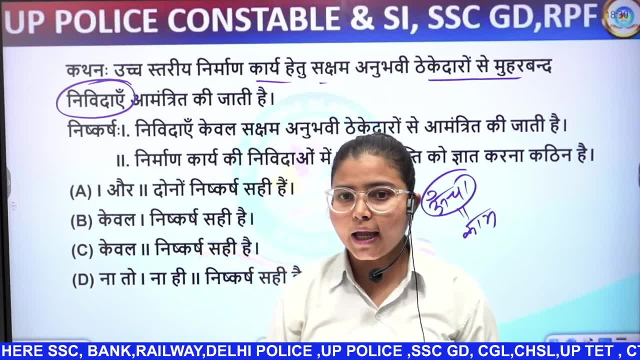 So he will get confused that how to get me out of the highway. Okay, And the engineers who are there? they have experience. What they have is experience. They do such things every day, So they will make a map of this thing. 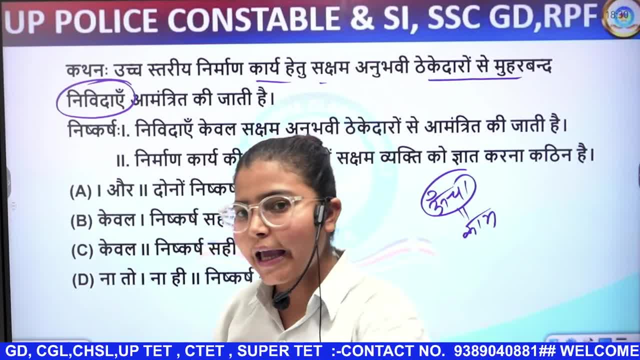 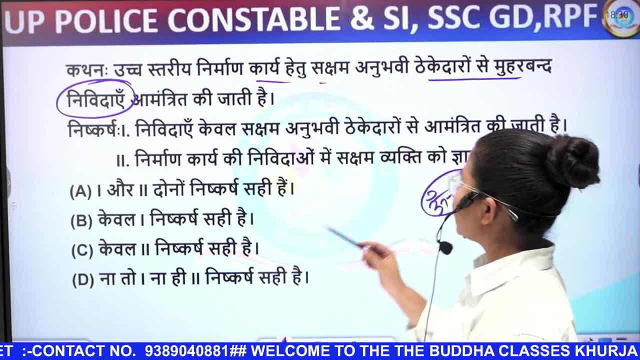 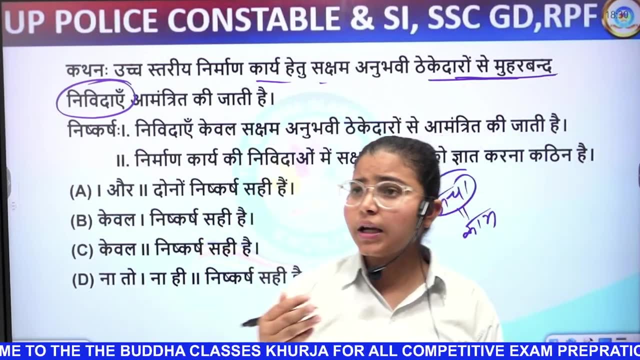 That you have to take it from here and turn left from here, turn right from here. whatever you have to do, they will tell you all the things in it. Okay, So in the same way, what is said in it? It is said that a person is invited to do some difficult work. 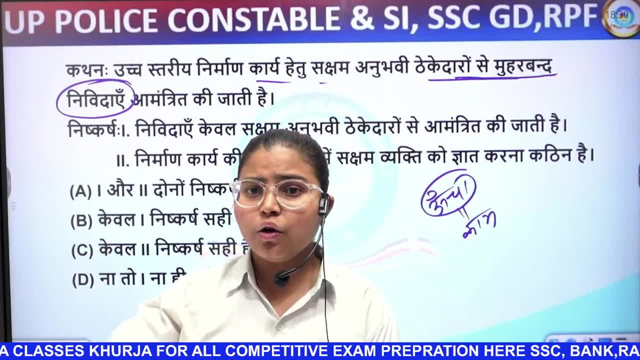 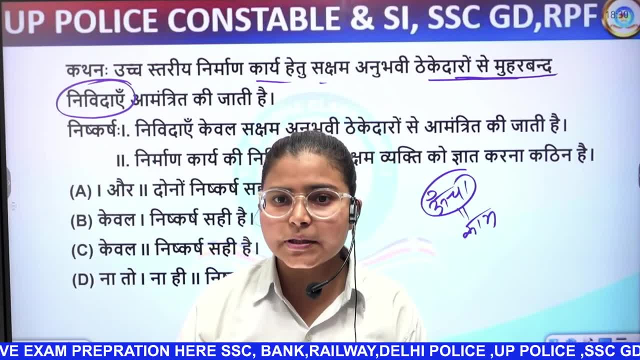 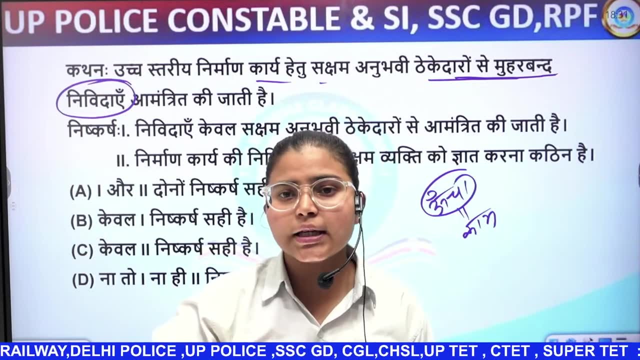 It has been said that someone is doing some high work, So we are a new person. So to give him experience. only some unfaithful people are invited. That you handle it, give it experience, Is it clear? So on the basis of this, you have to see its conclusion. 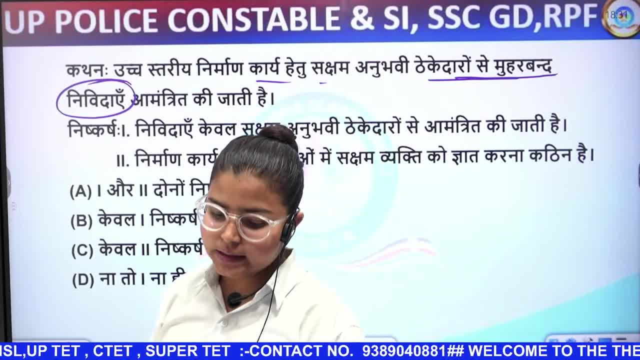 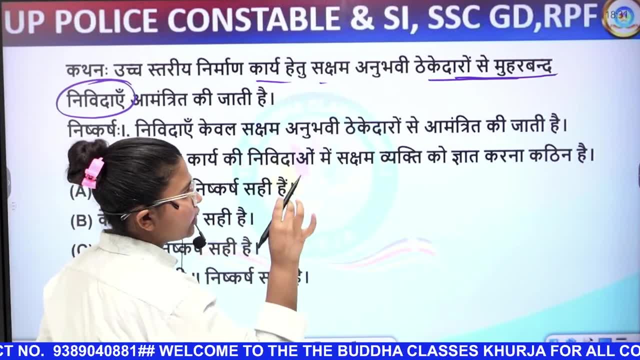 And you have to comment on the answer. What will be the correct answer to this? It has been said in this Discourse, number 1.. Only capable and experienced contractors are invited to the construction site. Yes, this has been said in the question. 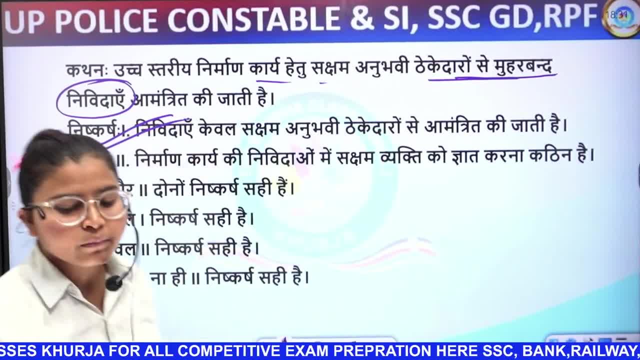 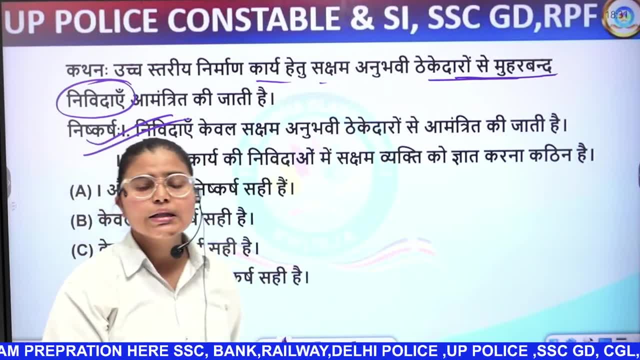 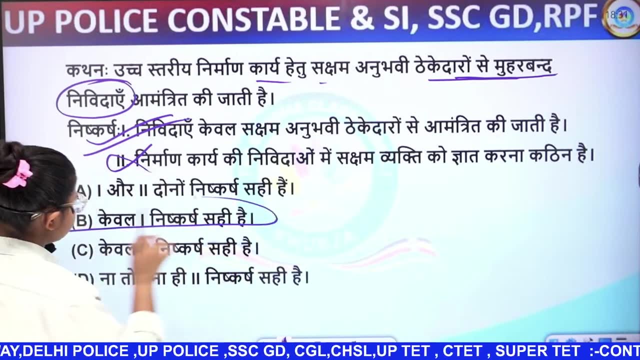 So the first one will follow The second one has been said It is difficult to find a capable person in construction sites. No, We can't say that It is difficult. This will be wrong. Only one of its discurses will be correct. 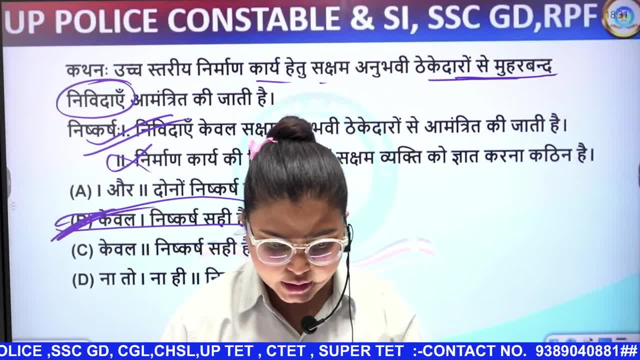 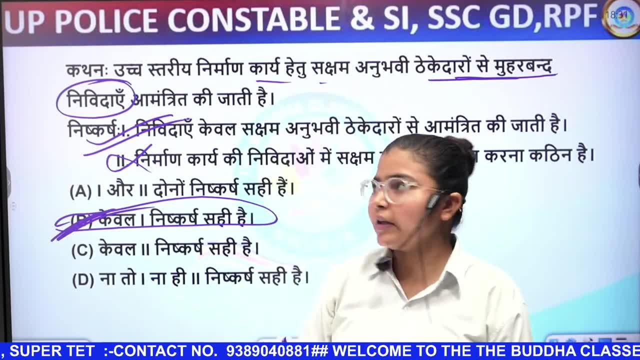 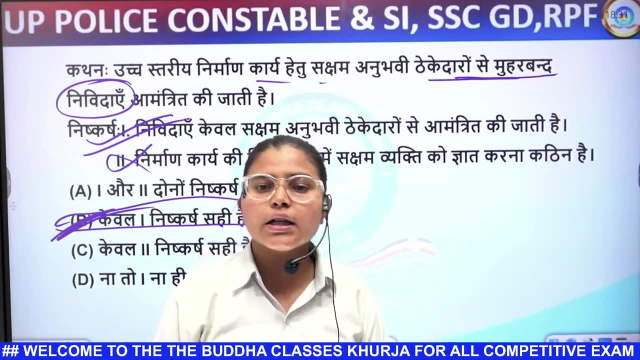 Option number 2.. Manoj ji is saying: Since when have I been taking the batch of RPF Constable? The batch of RPF Constable will be started soon On your demand, By the way. this is the reasoning batch. 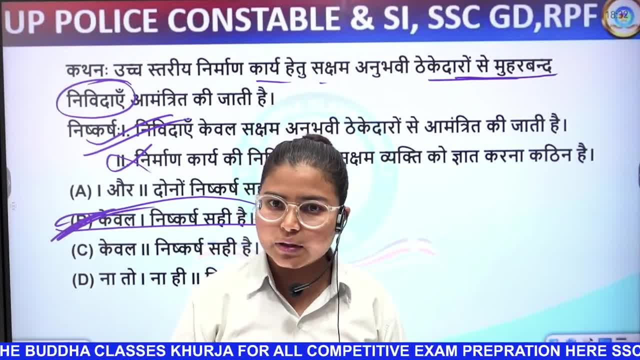 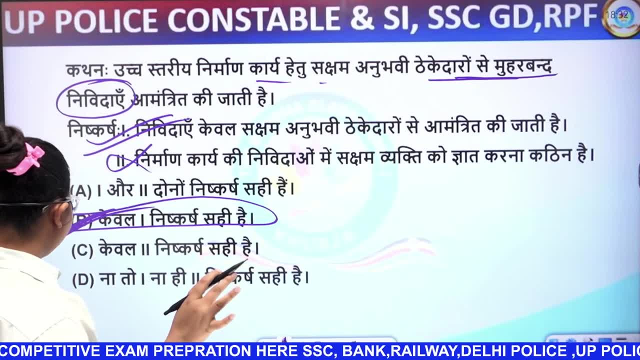 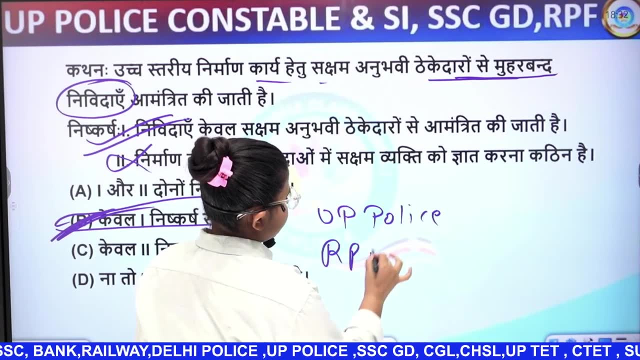 This is the foundation batch of reasoning. All the chapters will be completed in it. Okay, This is the reasoning. After studying in this batch, you want to give the exam of UP police, Or give the exam of RPF, Or give any exam of SSC. 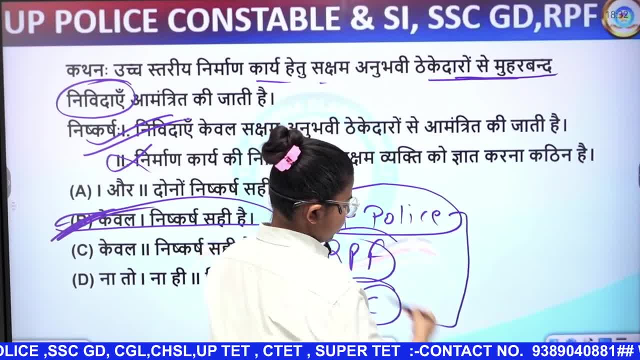 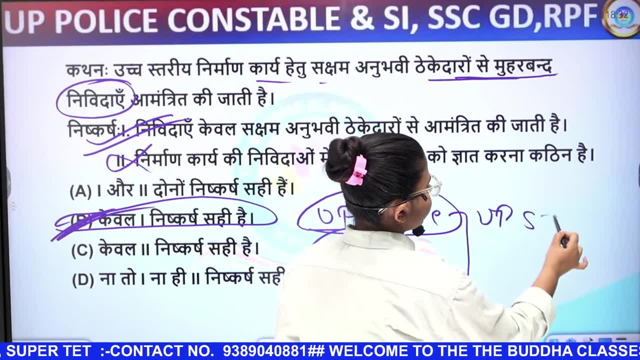 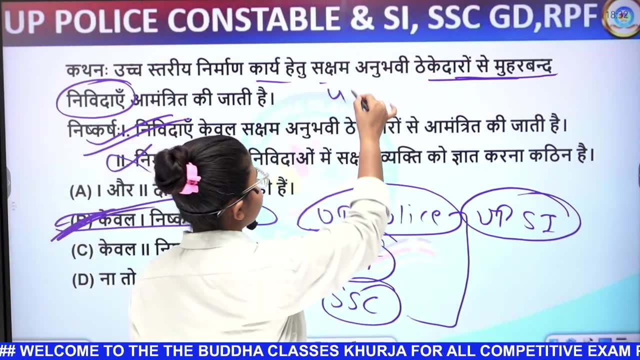 Or if you want to give, then you can also give the exam of RPF, SSC, UP, police, UPSI. You can also give UPSI. This is the foundation batch of reasoning In this. 46 to 46 chapters will be completed. 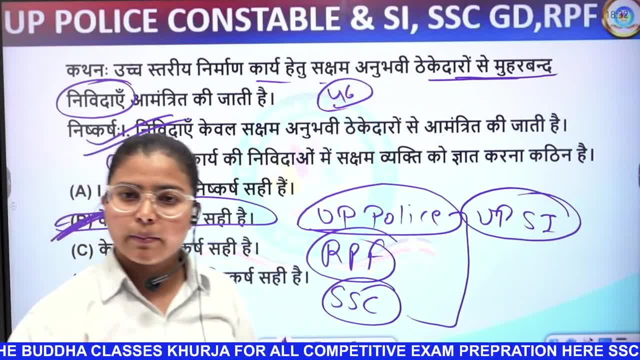 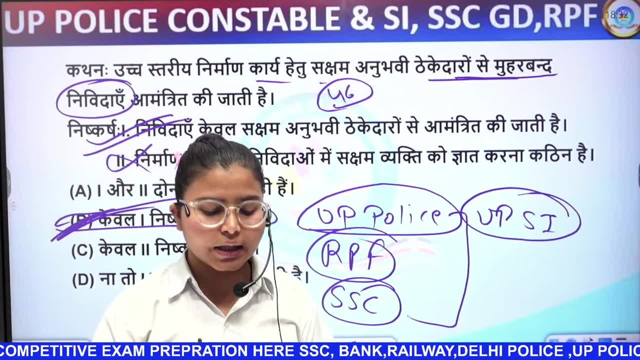 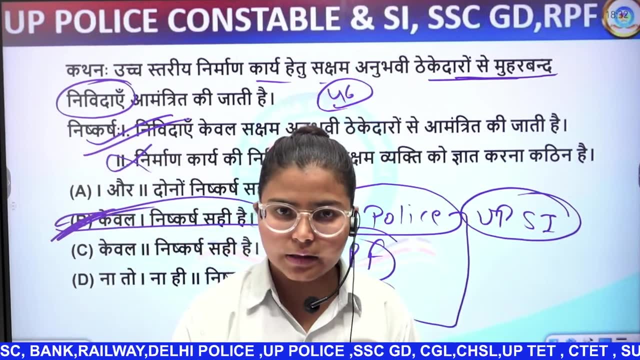 Which is in our total reasoning. Okay, Now some things are going on. first, I have mixed some chapters, Which is also for your UP police, Okay, For RPF too. After this, for SSC too, After this. Now, this is Kathan Discourse. 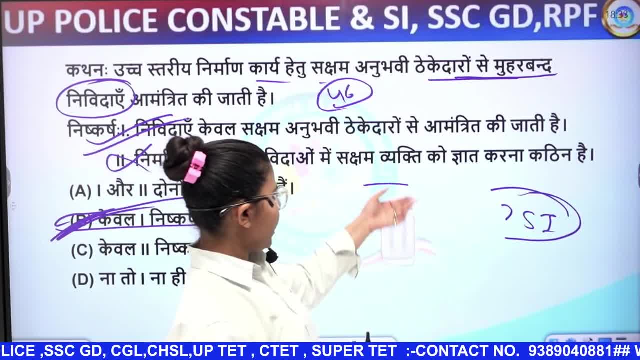 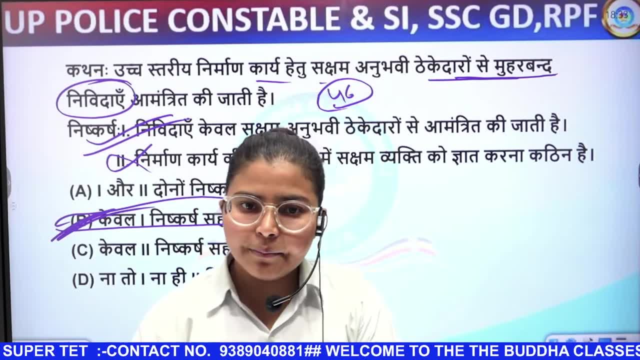 And Kathan Targ And chapter of Justice Enigman. These are mostly asked in UP police and UPSI. So that's why these chapters are going on. But you don't take tension for RPF at all. You will get the batch for RPF too. 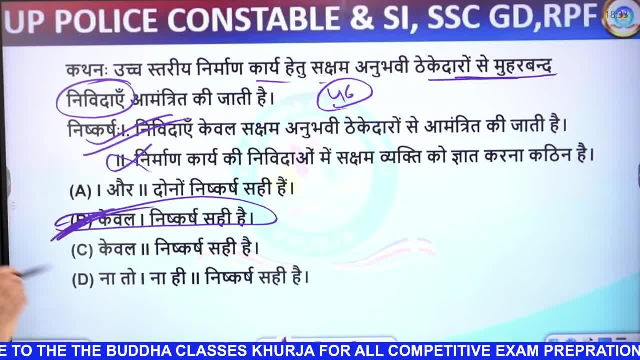 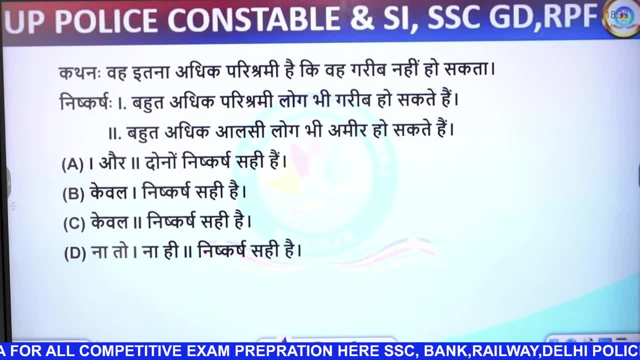 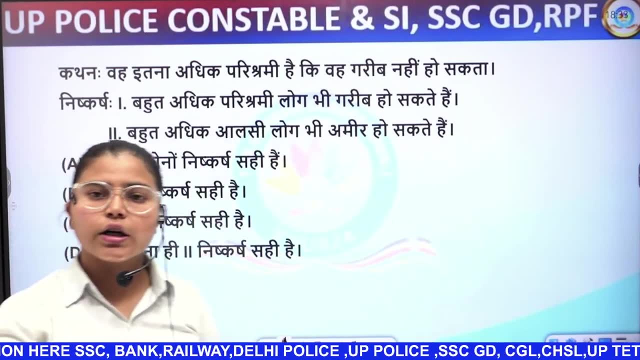 Okay, So the right answer for this Option number will also be the correct answer: See the next question. He is so hardworking that he cannot be poor. What is said in the question? That he is so hardworking that he cannot be poor. 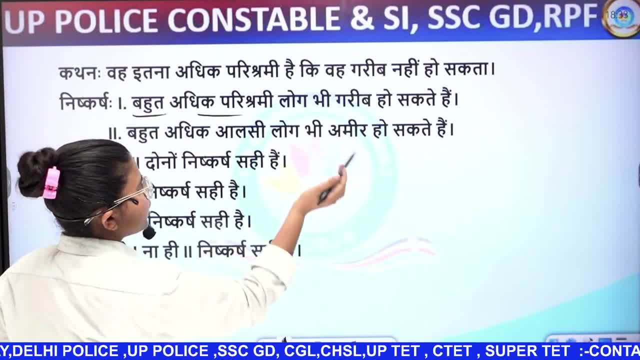 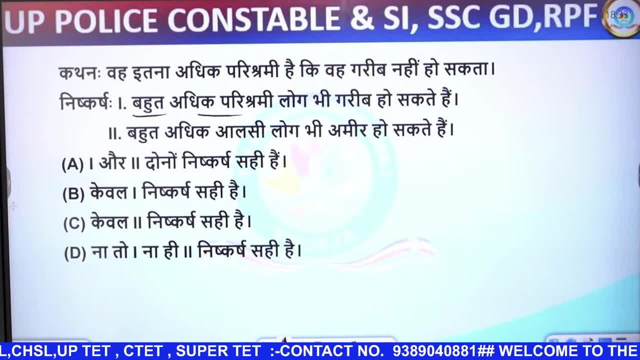 Discourse number 1 is given. Very hardworking people can also be poor. Very lazy people can also be rich. Which discourse will you correct for this Once? tell me by commenting the answer: Which discourse will you correct for this Once? all the companions will say it quickly. 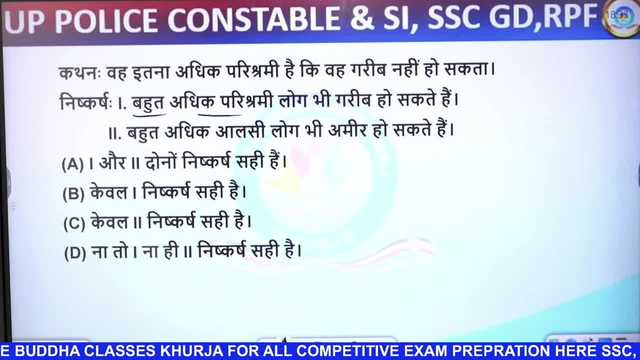 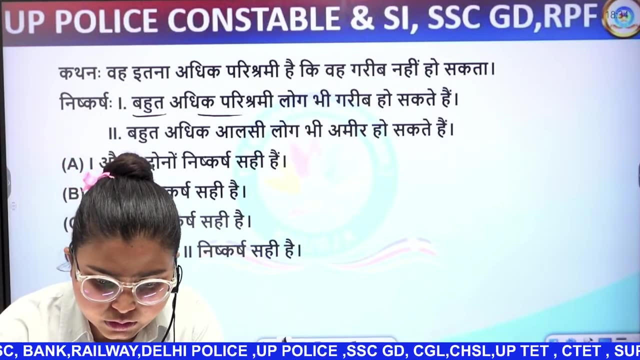 Which discourse will you correct for this? Use great easiness. You know he is intelligent Just once he says the right answer. What happened? Hurry up that comment Quickly. What vinegar will you 듣, comte sir? Which mathul one will you read, comte sir? 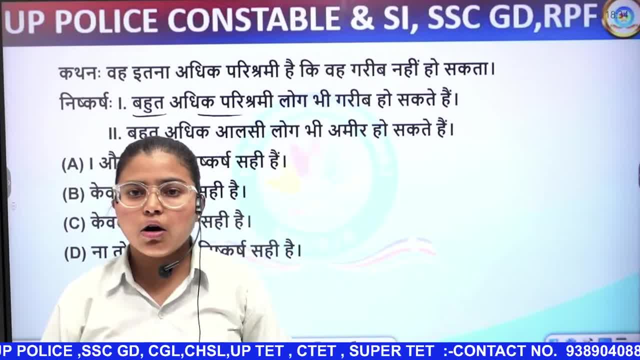 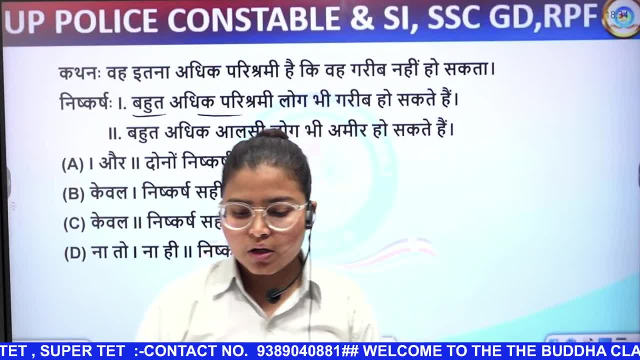 Mathe one. Mathe is used by Anil Sir & Manoj sir, But the math for RPF will be surprises to you. through. Manoj sir, your class is going on at 2 o'clock right now. there are two to three math classes going on, okay. 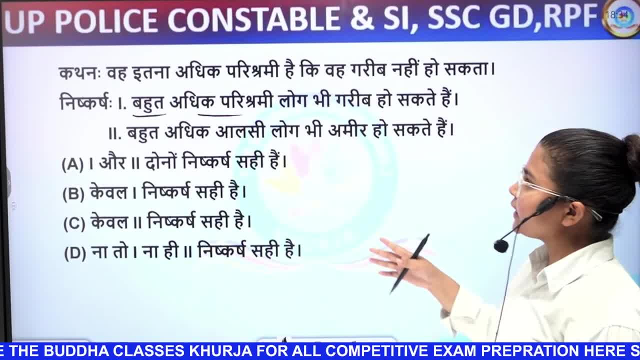 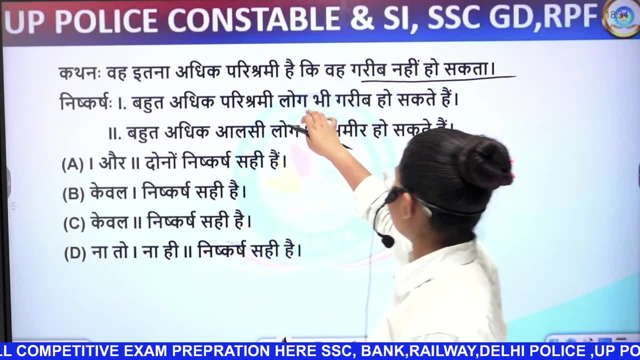 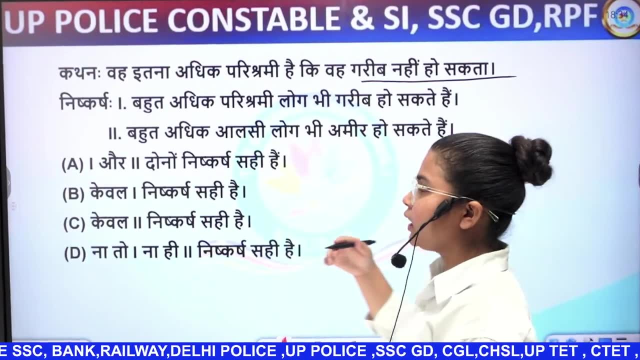 yes, okay, let's see this. they are so hard-working that they cannot be poor. it has been said that very hard-working people can also be poor. yes, this is absolutely right. no matter how many people are there, they work very hard, even after working very hard. 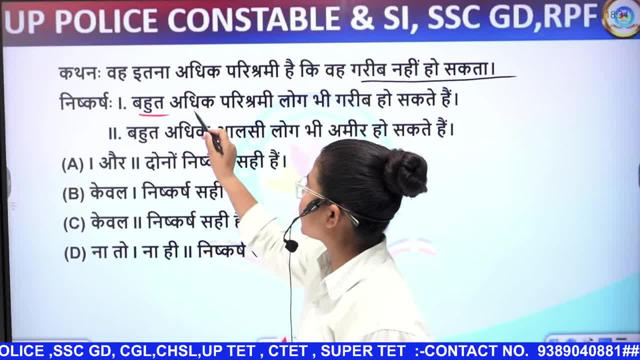 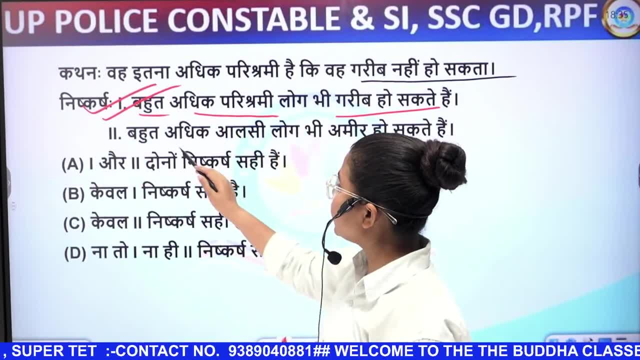 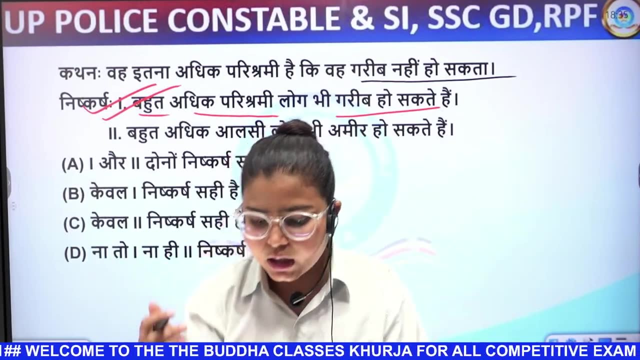 they do not have anything. so we can consider this thing absolutely right. even very hard-working people can also be poor. this is right. option number is right. it has been said that even very lazy people can be rich. yes, this can happen, it is possible. 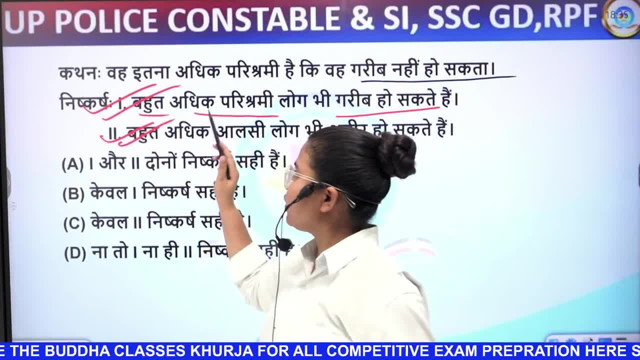 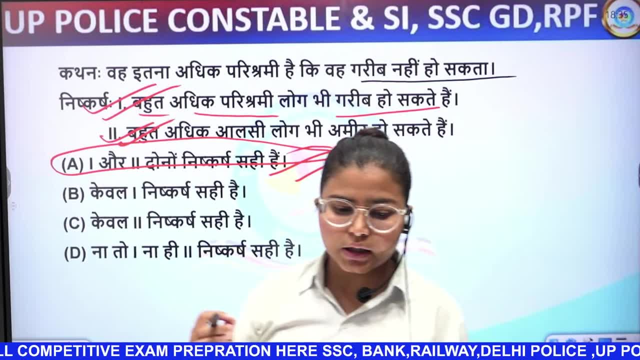 so what we will do is correct it. which one will be right? one and both will be right? option number a: the answer to this question will be correct. the answer to the question given will be correct. okay, I understand so much. 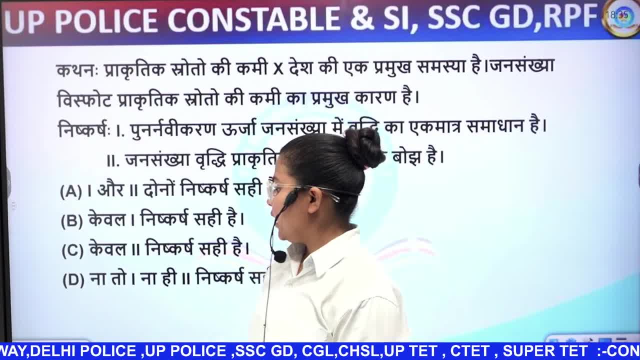 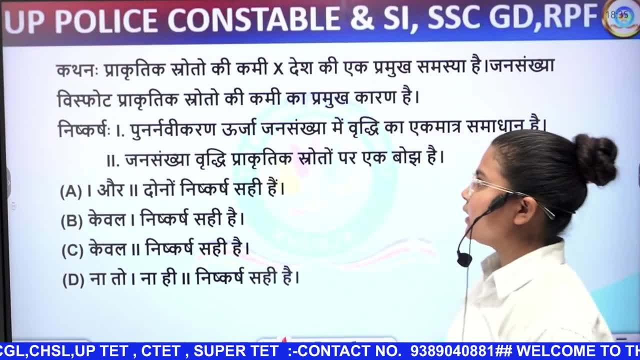 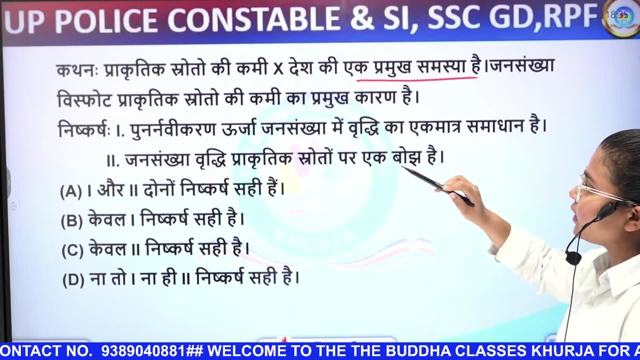 once. tell me quickly, I do not understand. after the class, I will tell you the timetable that our classes are going on. at what time? okay, the question is given. the lack of natural resources is a major problem of the country, which is the main reason for the lack of natural resources. 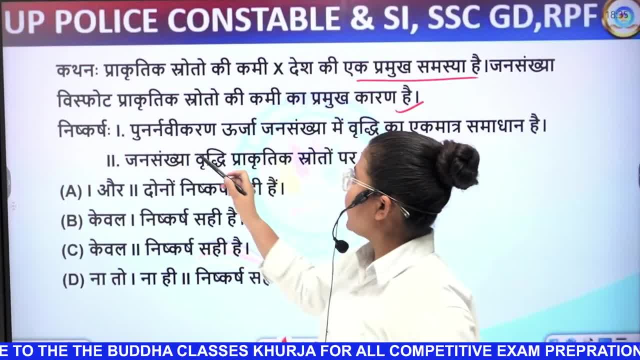 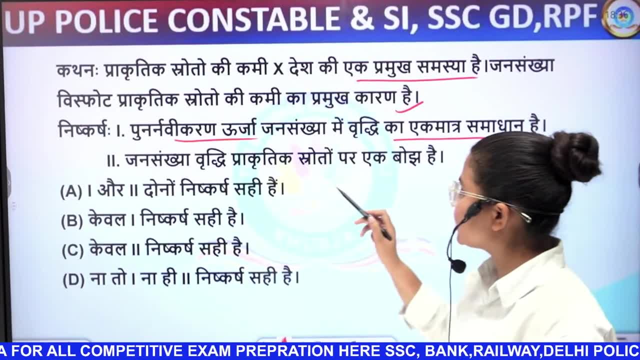 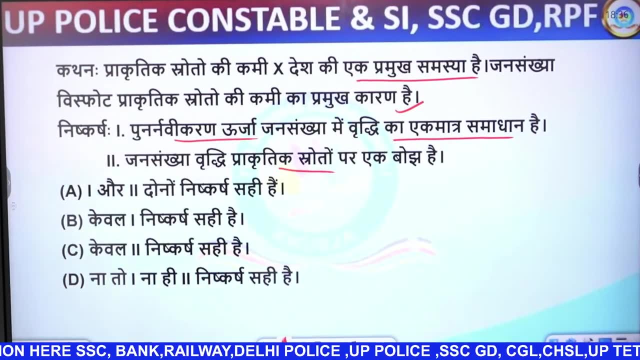 number is given to you first. there is only one solution for the lack of natural resources: the number of natural resources is a burden of the natural resources. what will you find the right answer to this? once, tell me in the comment box what will you find the right answer to this. 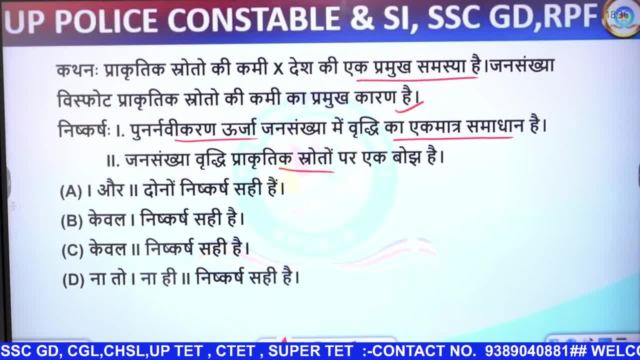 quickly comment on the answer to this. which one? are you going to find the right answer to this? I forget. I better not tell you people now answer. question is opened once. try to add your answer to the comment section. this is should be a question according to the question we have come up with, comin. 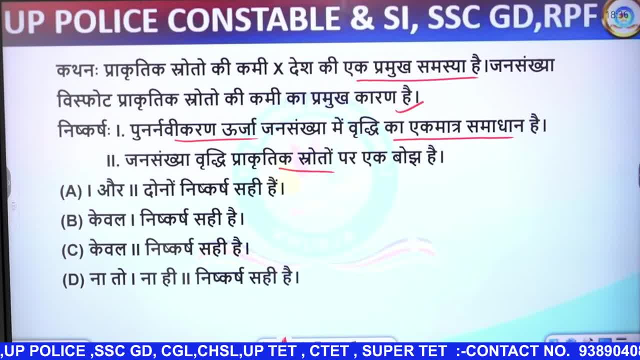 now try to write and answer the questionets you will find in the comment box, as it is written in English: Friends, what will be the right answer to this question? What will be the right answer to this question from your point of view? 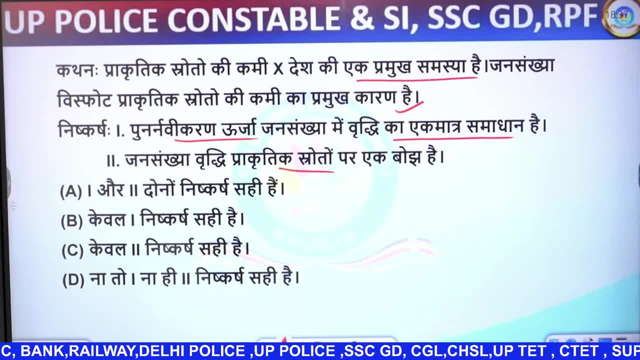 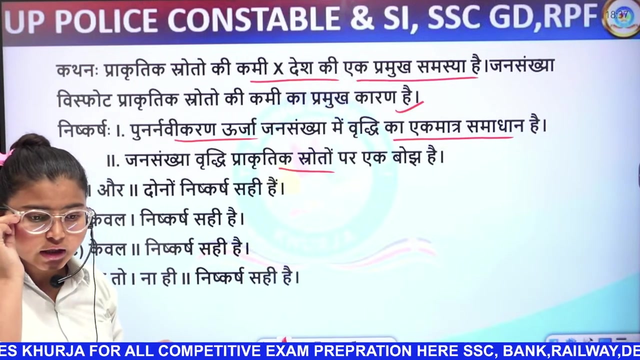 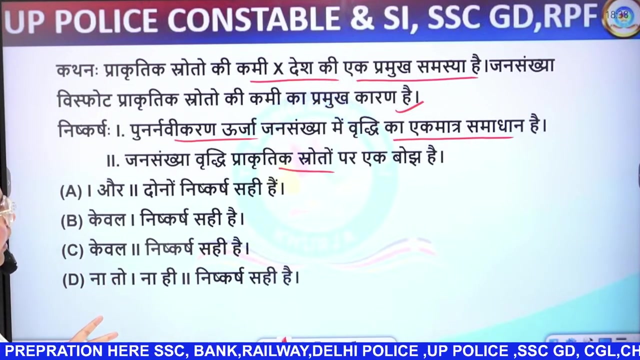 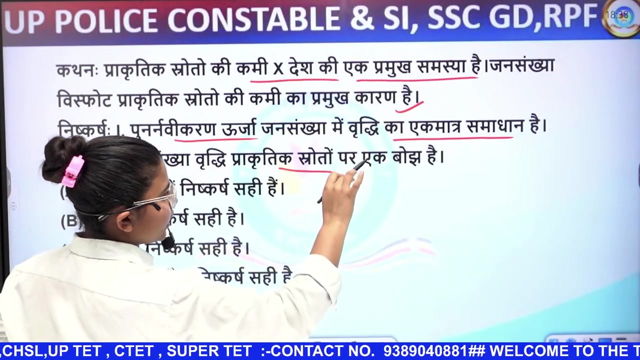 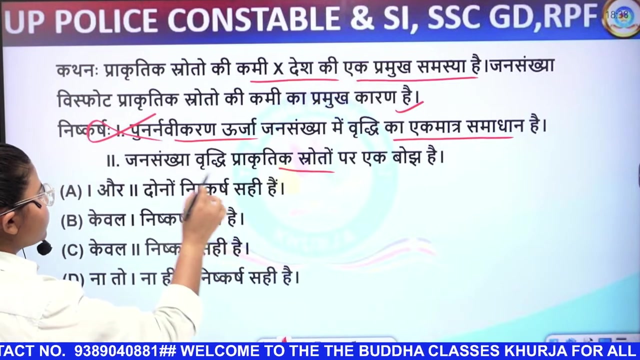 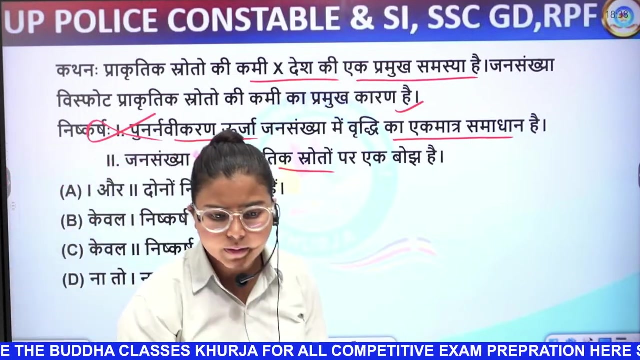 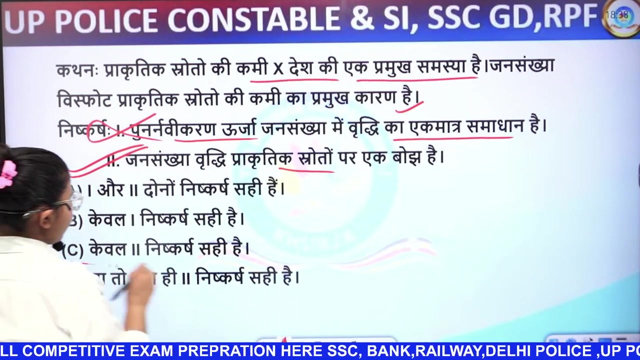 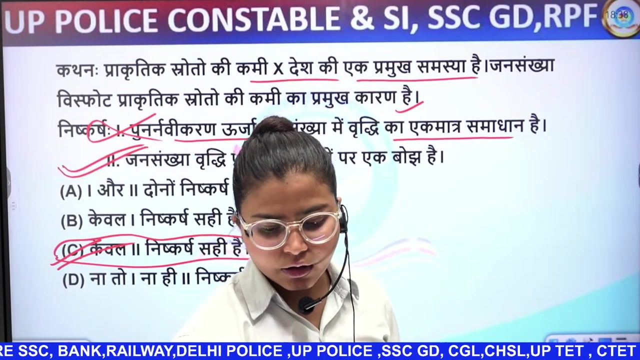 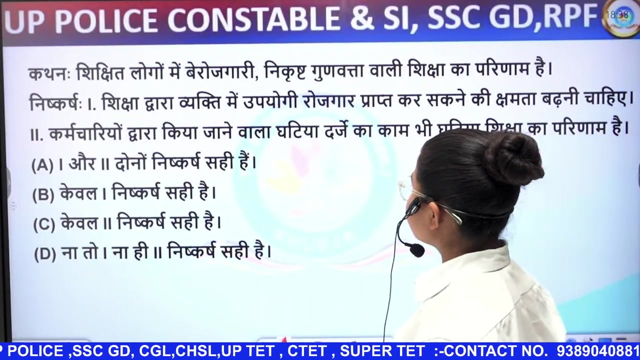 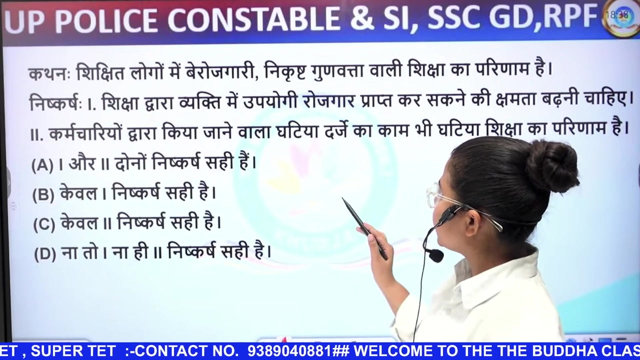 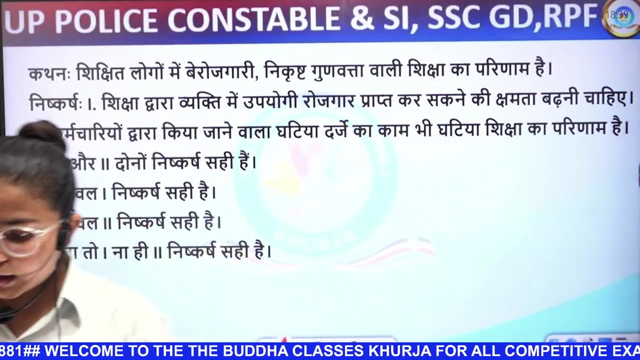 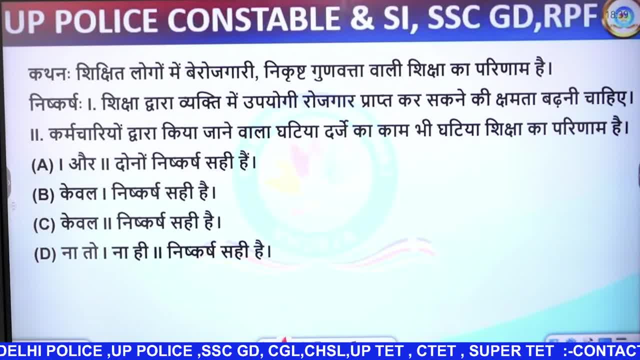 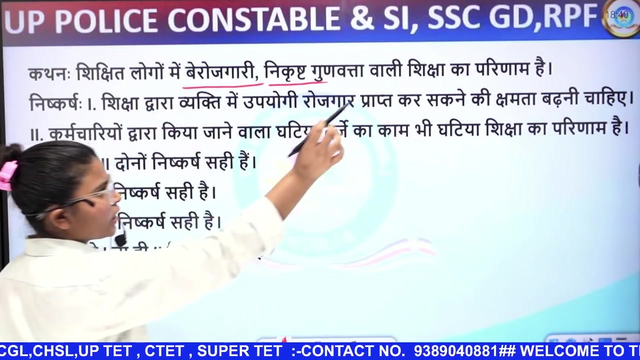 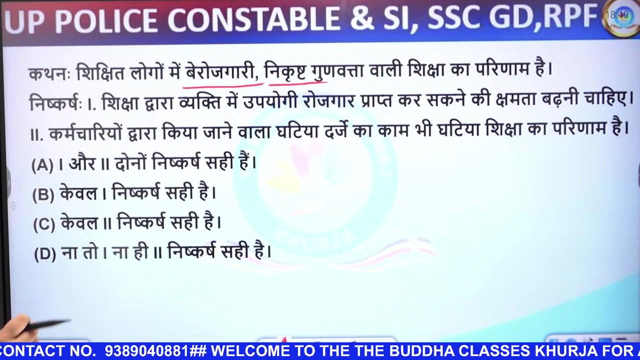 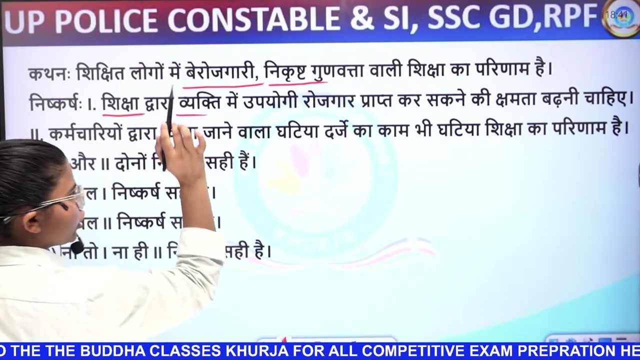 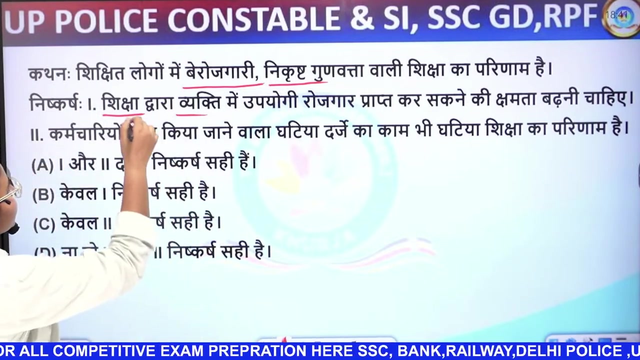 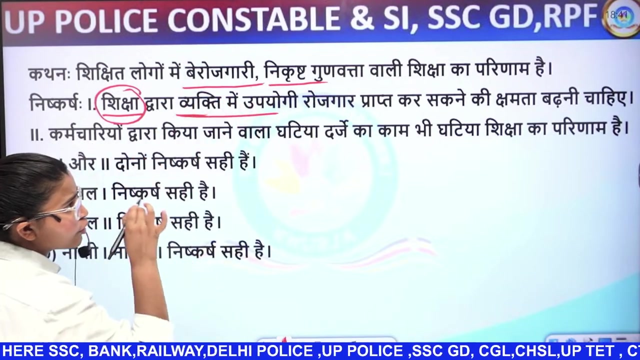 What will be the right answer to this question from your point of view? Yes, it's a very easy question. Yes, it's a very easy question. Tell me quickly. Yes, it's a very easy question. Yes, it's a very easy question. 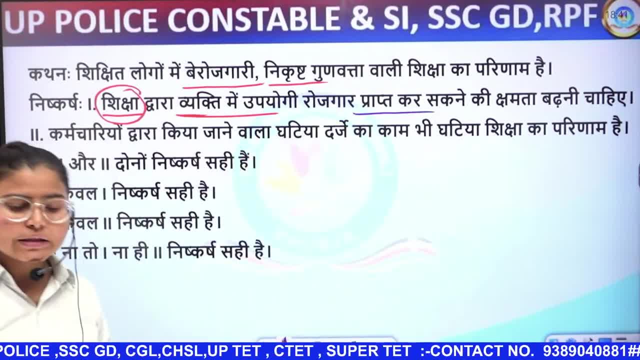 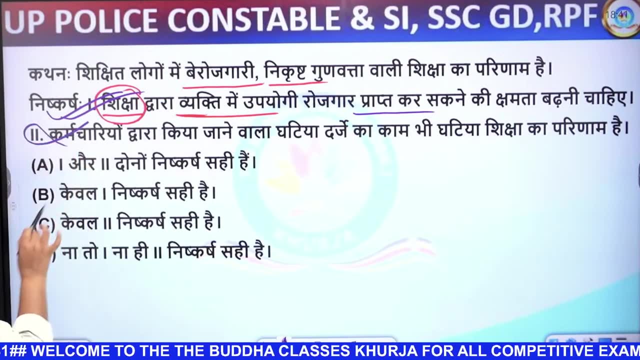 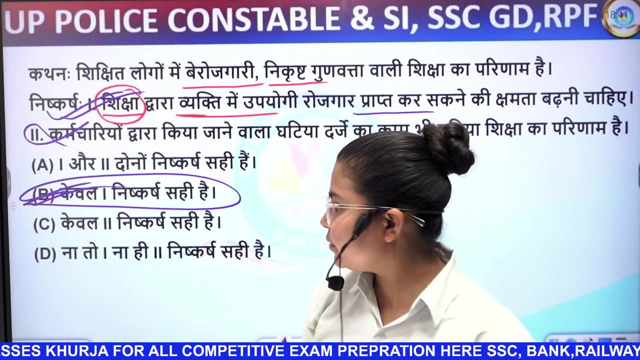 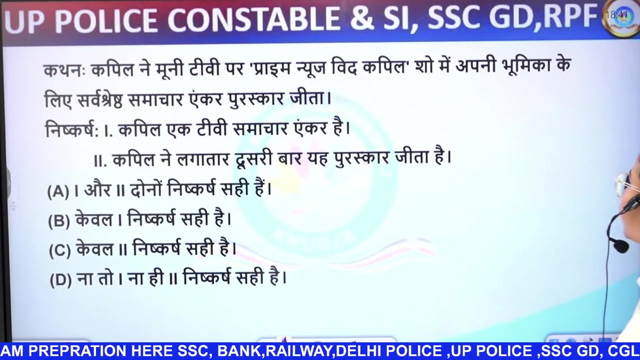 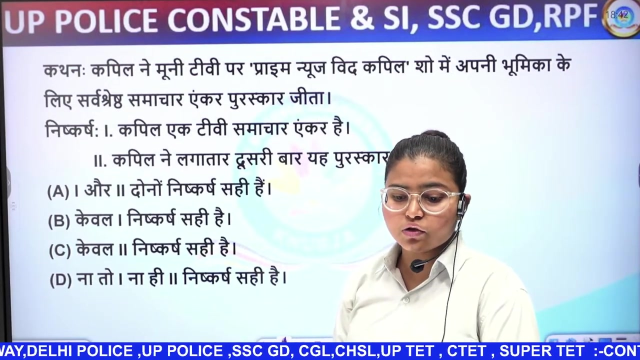 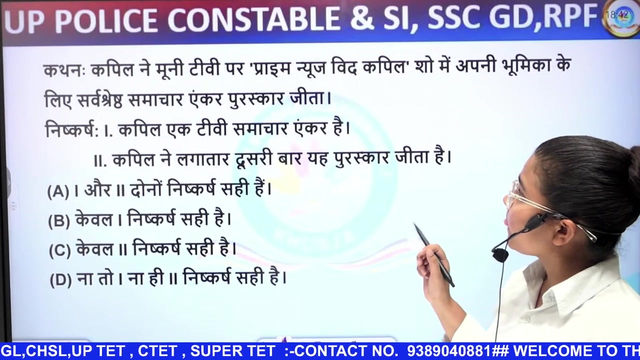 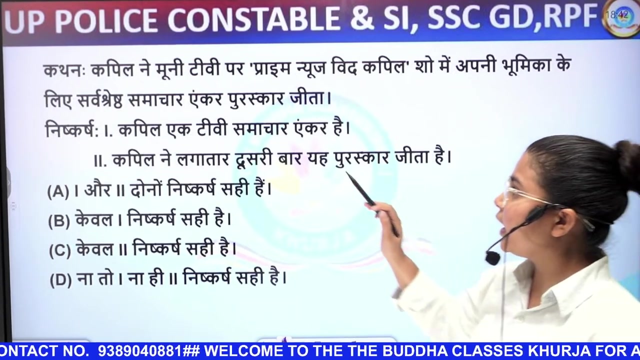 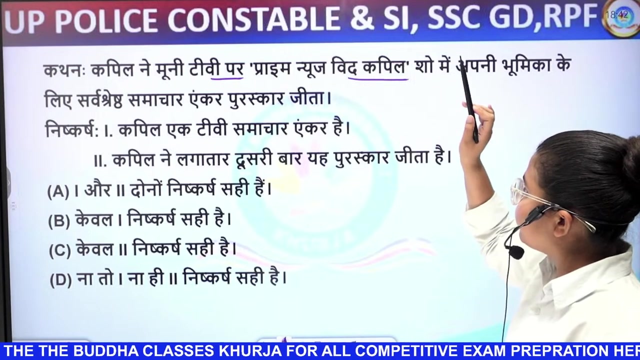 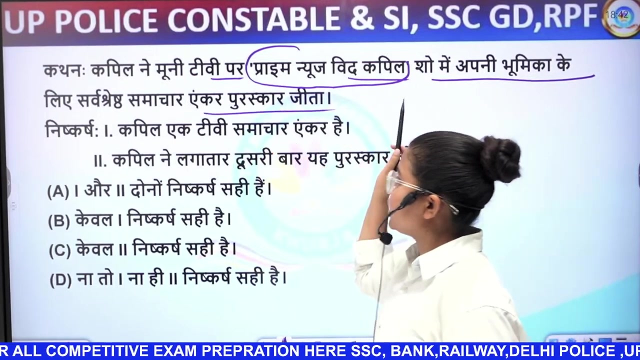 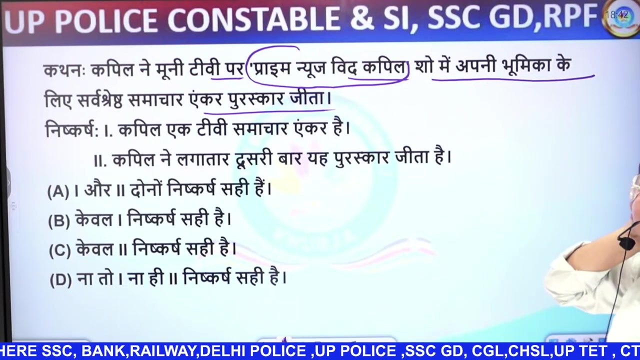 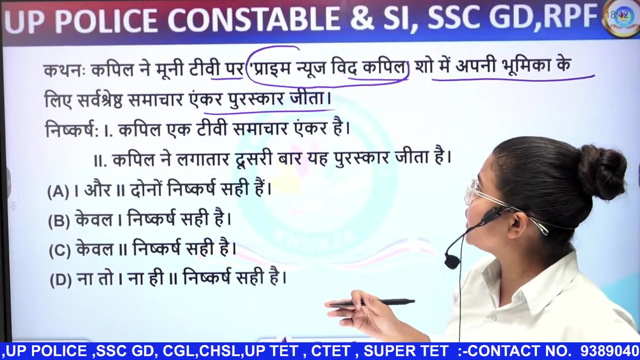 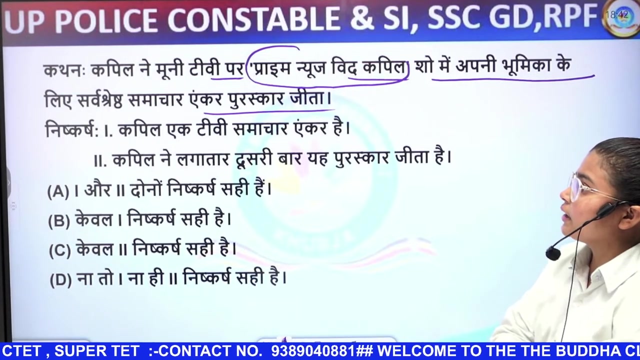 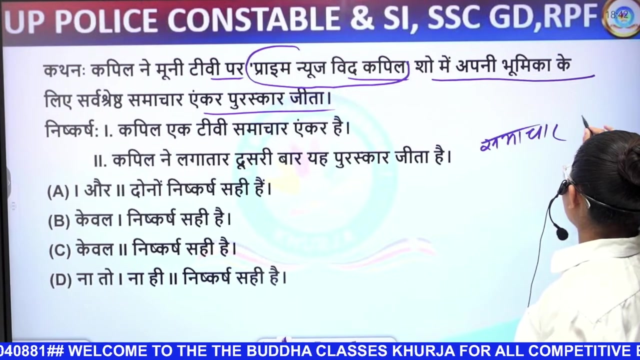 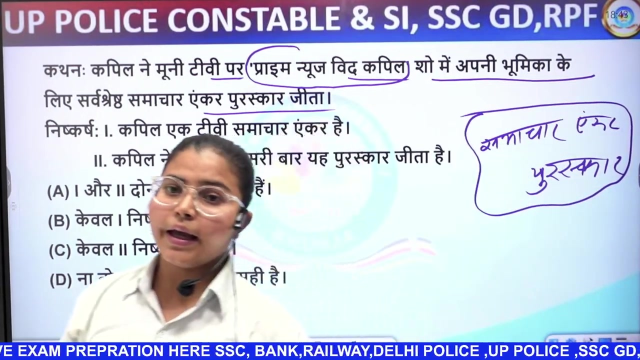 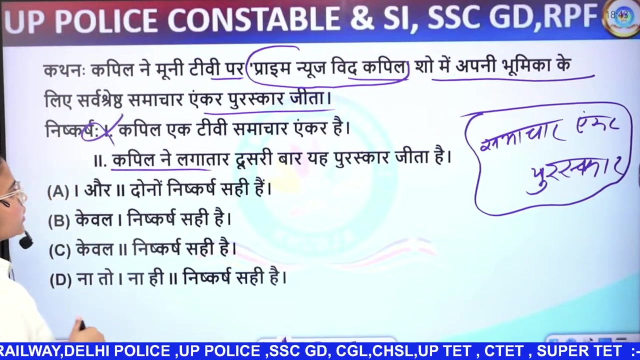 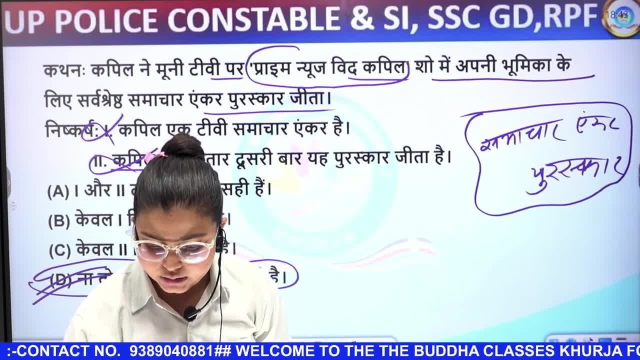 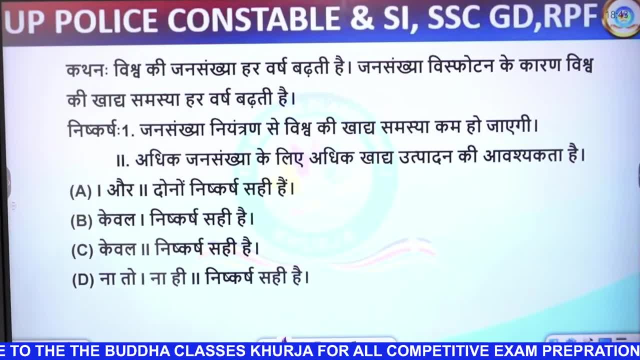 Neither the discussion is correct nor the other is correct. What do you say, friends? Okay, Go ahead, And this will be the last question of our class, And this is the last question of our class. This is very important for you. 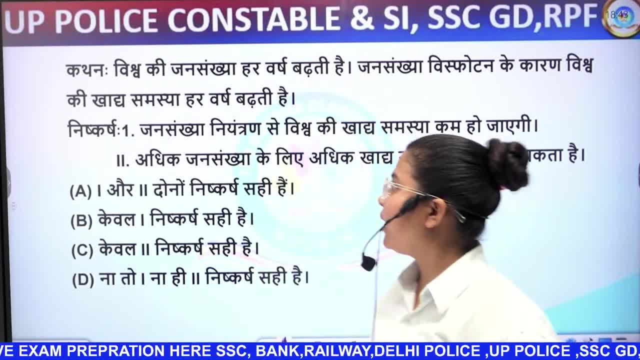 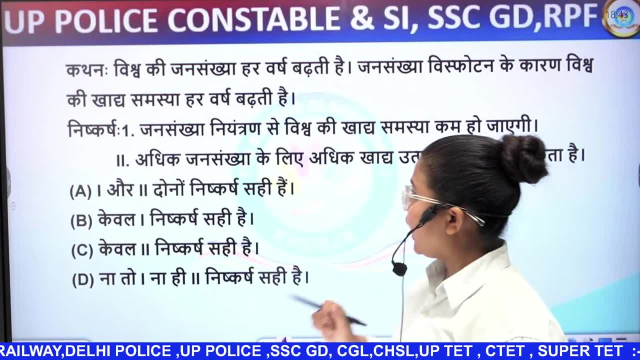 We will comment on the answer soon. The question has been given to all of you. So the population of the world increases every year. Due to the export of population, the problem of food for the world increases every year. The question number 1 has been given. 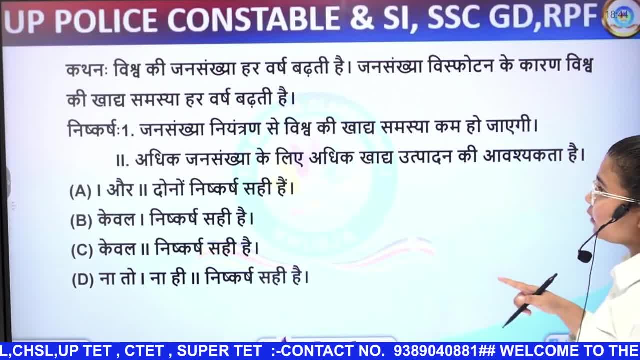 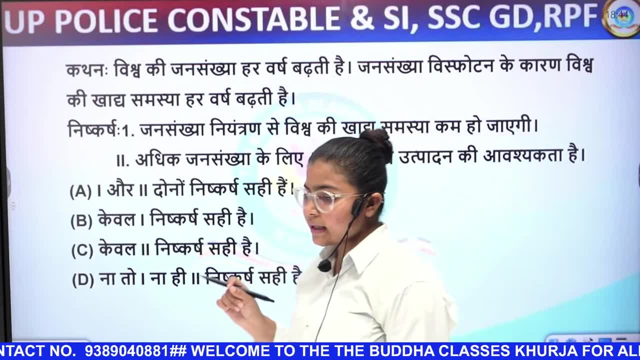 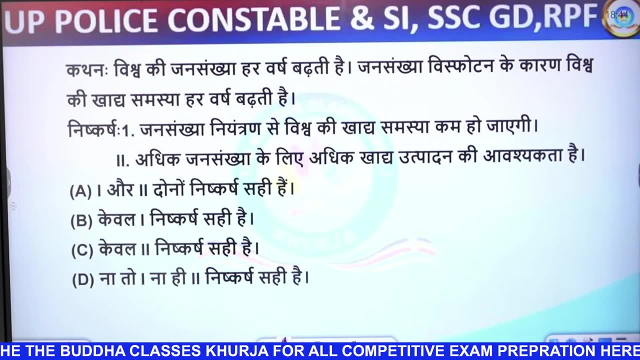 Will the problem of food for the world reduce in the population control Or will there be a need for more food for the population? Which of these questions will you correct? You have to give the correct answer in the comment box Quickly. what will be the correct answer? 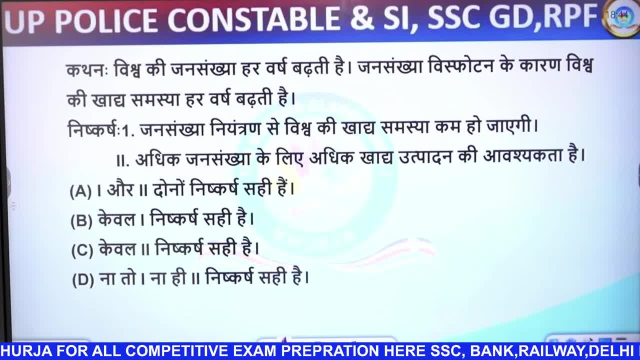 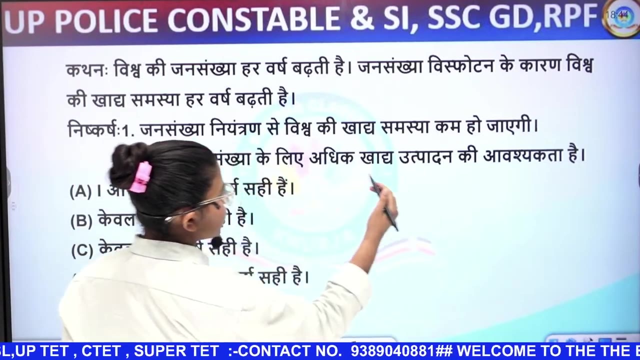 Please give us the correct answer. It has been said that, due to the population control, the problem of food for the world will reduce. Is it true? If population control is controlled and the population is reduced, the problem of food for the world will reduce. 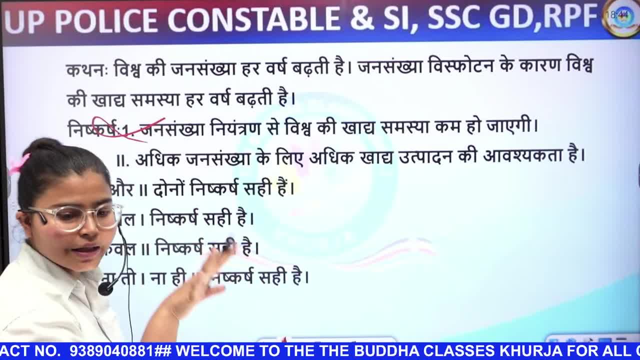 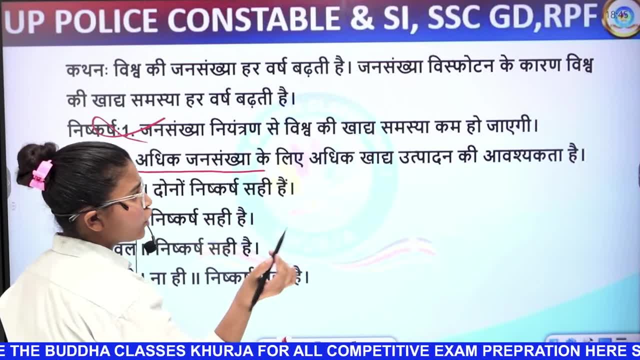 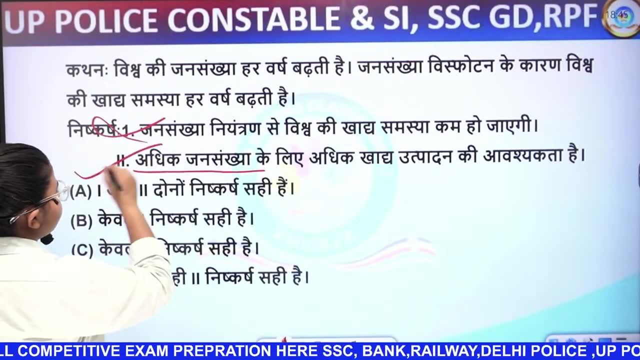 No, this is wrong. He has written it by mistake. Niskars number 2 is given: For more population, more food production will be required. Yes, for more population, more food production will be required. He has said the right thing. 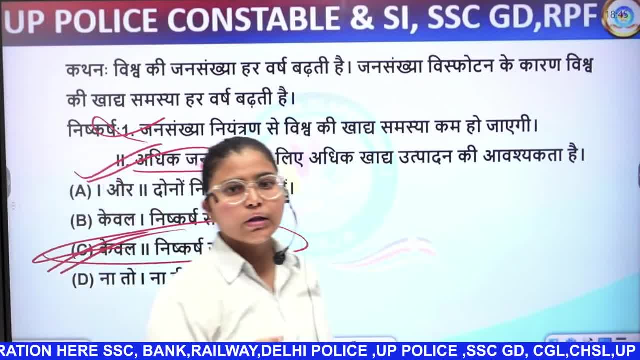 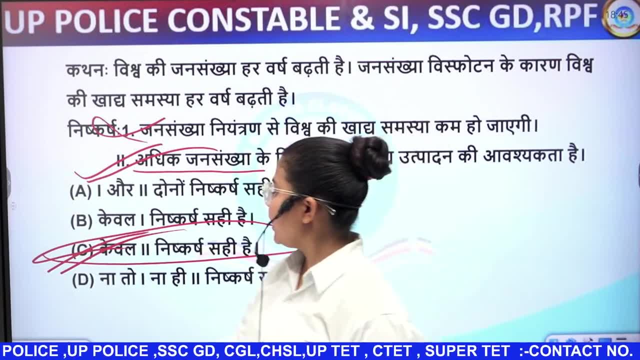 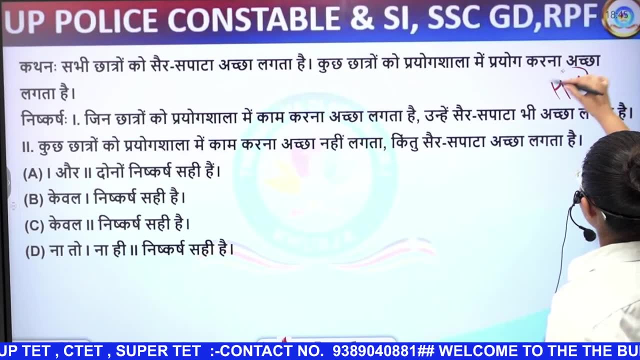 The correct answer is option number C. Only Niskars 2 follows. What does it do? Only Niskars 2 follows. Next question: This is the last question of our class And once you answer this question in the comment box. 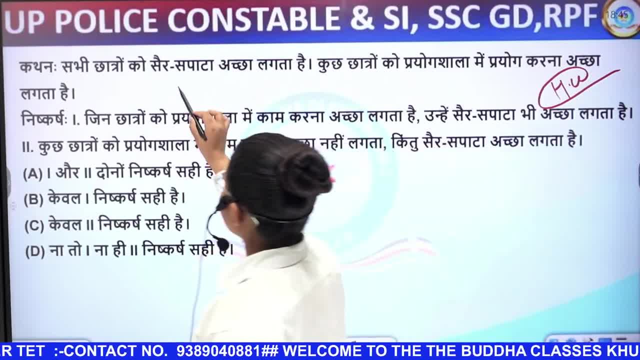 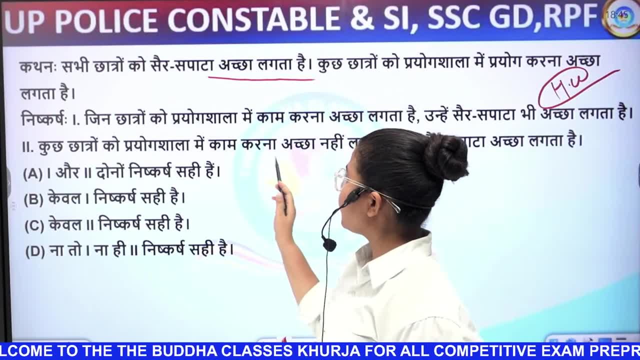 comment it. All students like to use the chair. Some students like to use it in the practice room. The students who like to work in the practice room. they also like the chair. Some students don't like to work in the practice room. 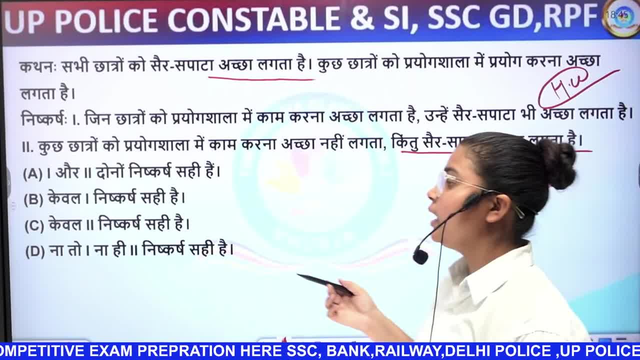 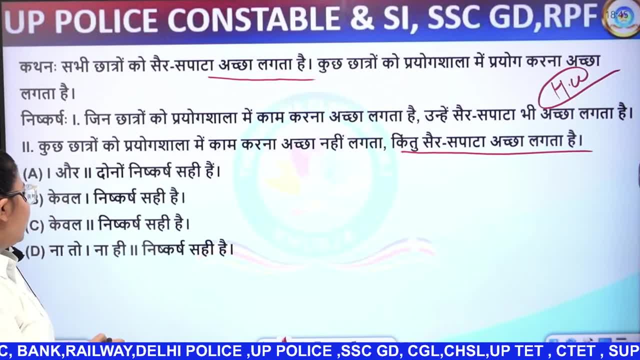 but they like the chair. Which Niskars will you choose? Once we will tell you which Niskars will be the correct one, We will quickly tell you which Niskars will be the correct one. It is said that the students who like to work in the practice room. 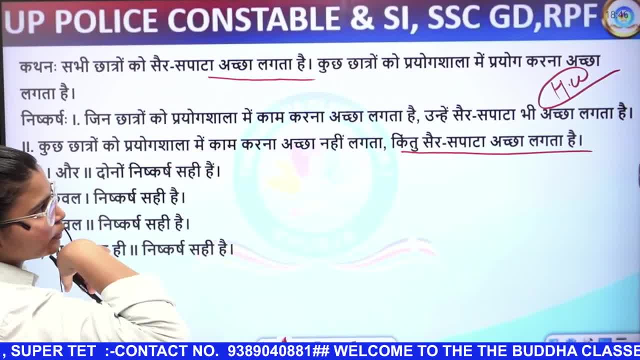 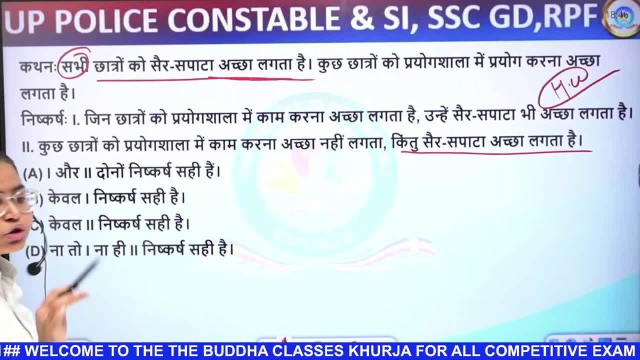 all students like to use the chair. Some students like to work in the practice room. But what all students like, They like the chair. Hold the language of the question: The students who like to work in the practice room. they also like the chair. 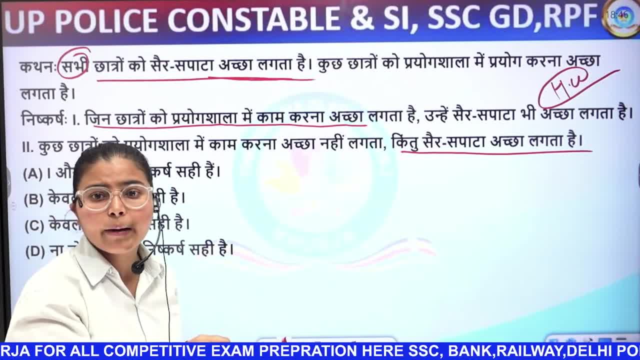 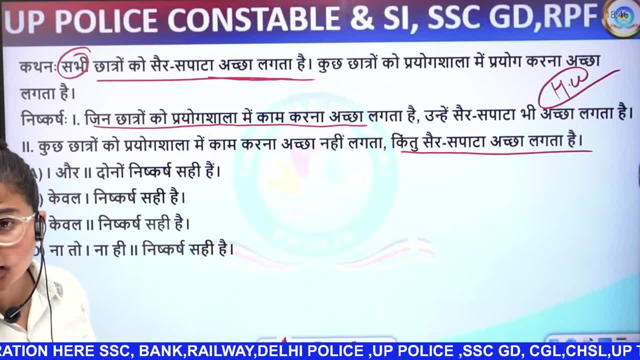 They also like the chair. This is impossible for us to say. This is very difficult for us to say. The students who work in the practice room, they also like the chair. We cannot accept this If we look at it according to our logic. 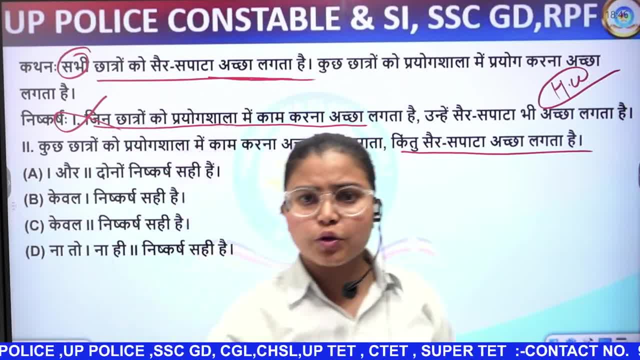 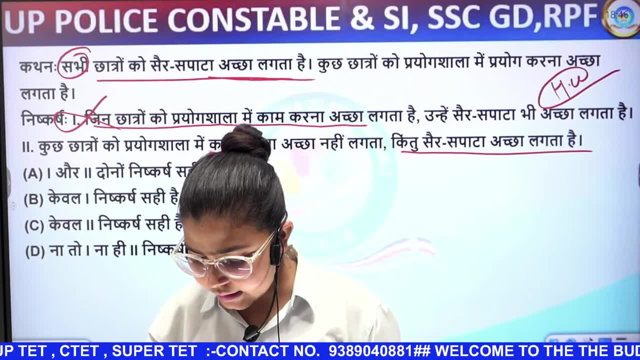 it is possible that the students who work in the practice room they also like the chair. That is why they are happy in the practice room. What is the matter? Is it okay? Is this right? Yes, it is. Yes, it is. 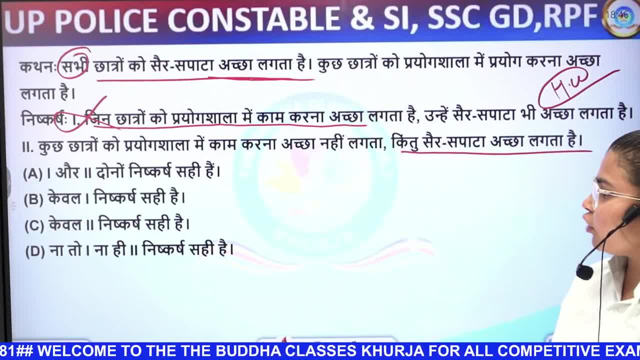 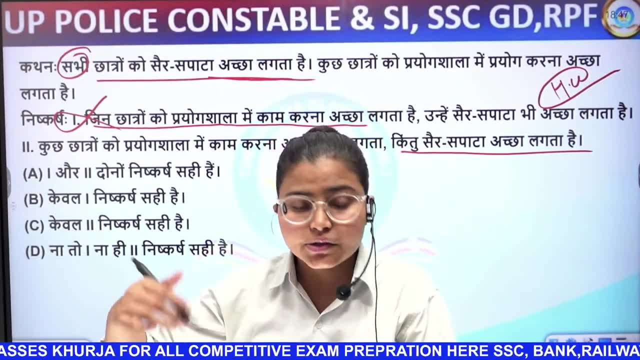 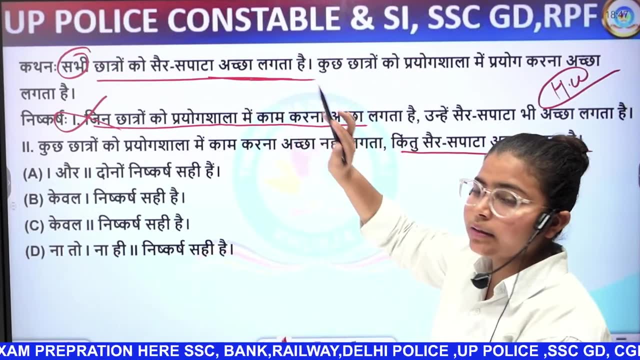 We will tell you soon. Some students do not like to work in the practice room, but they like the chair. Yes, this is absolutely true. Those who do not like to work in the practice room, they like the chair, Because it is said that all students like the chair. 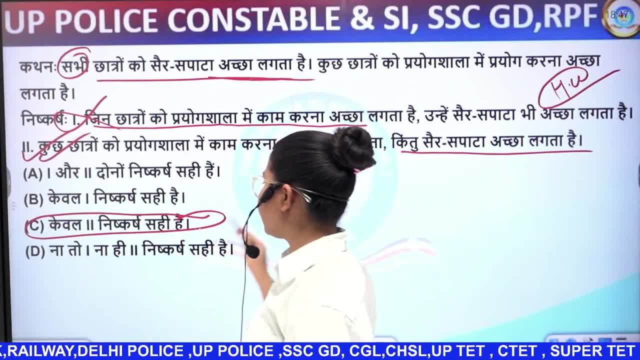 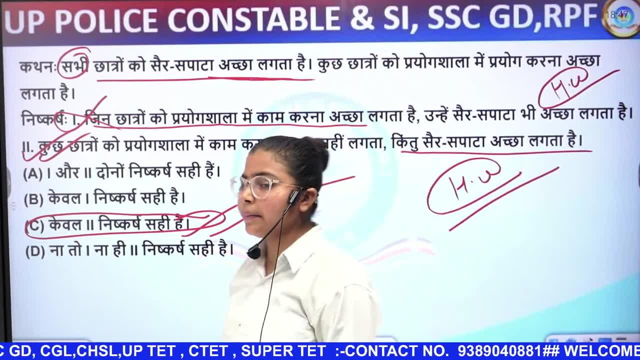 There are only two answers to this question. Option number C is the correct answer. Once all students will answer this question in their own language, They will answer with their own logic. They will answer with their own logic. Okay, Let us talk a little about our time table. 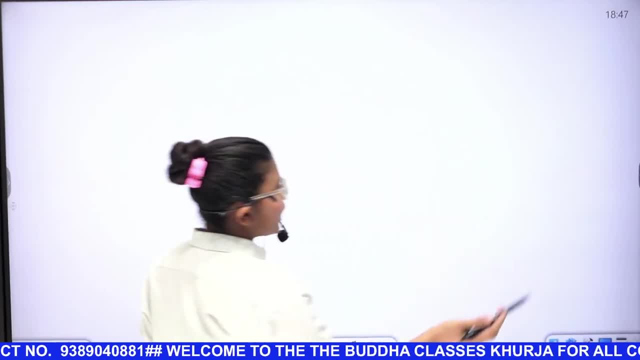 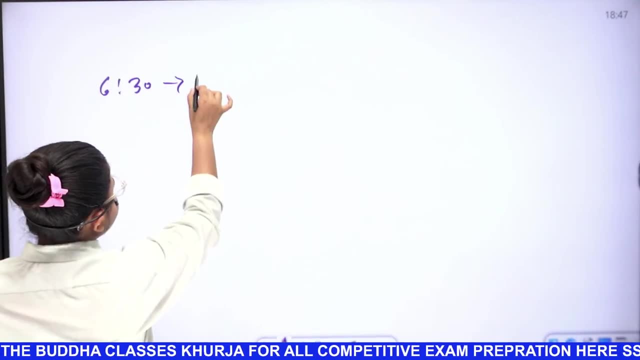 Let us talk a little about our time table. What are the batches going on at what time? What are the batches going on at what time, Friends, from 6.30 pm it becomes 7.30 pm or 7.45 pm. 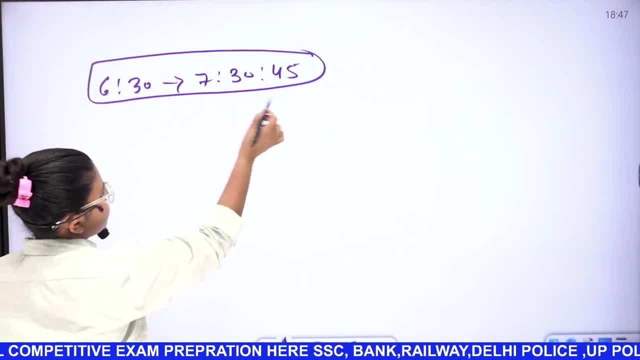 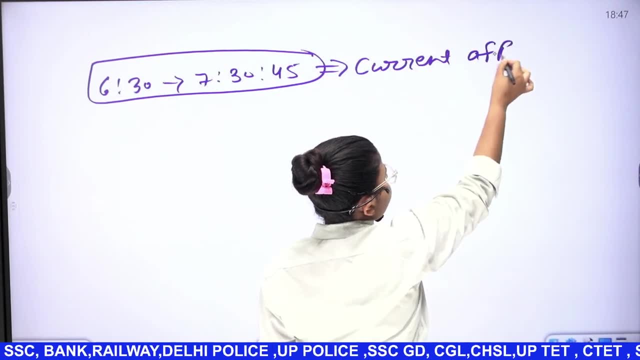 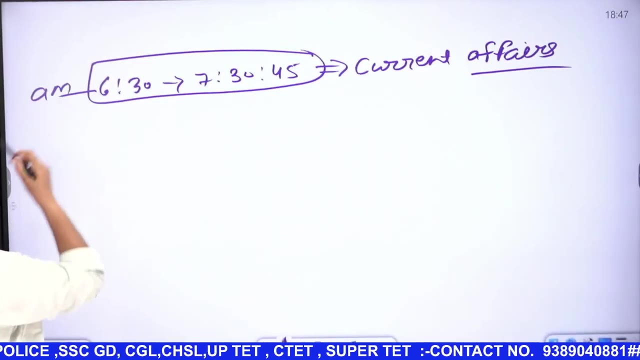 At this time, current affairs are carried out. Current affairs, Current affairs. Current affairs are carried out in the morning. Current affairs are carried out in the morning. This is the time of the morning. The time is 6.30 am. Okay. 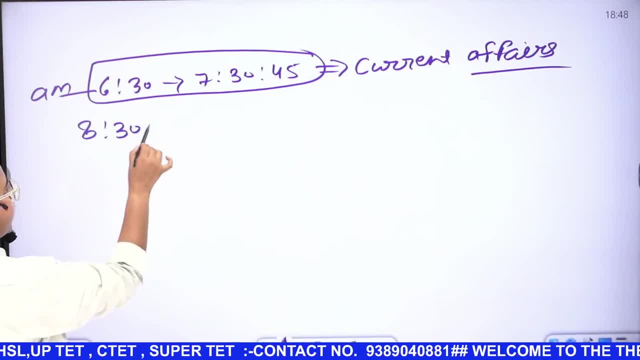 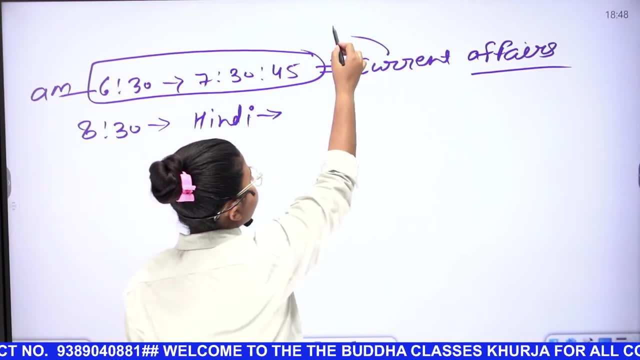 After this, the class is at 8.30 am. At 8.30 am there is a class of Hindi, which is taught by Anandveer sir. This current affairs class is taught by me only. My name is Priyanka Pal. 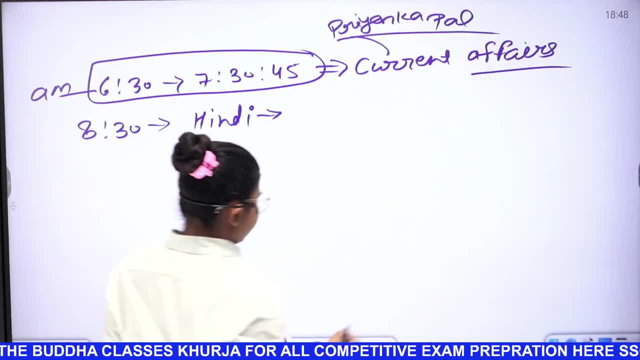 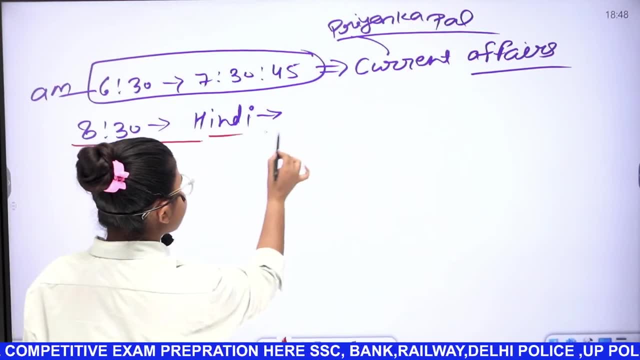 My name is Priyanka Pal. Priyanka Pal is my full name. This is current affairs. Current affairs are taught by me only After this kind of 8.30 am there is a hindi class, which is taught by Anandvir sir. 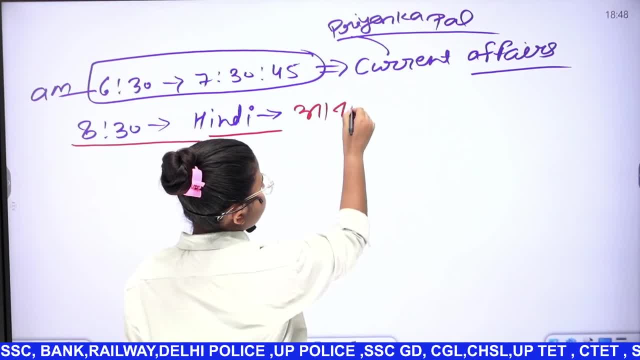 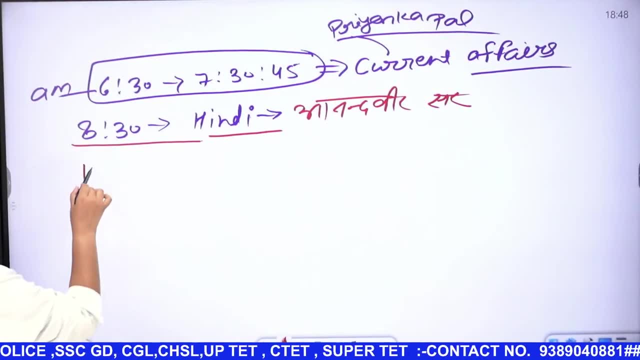 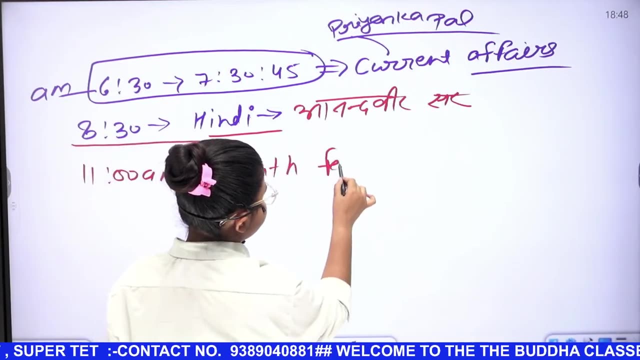 Anandvir sir. is there right? Anandvir sir legally focuses to the class. After this: the class is at 11 am. After this: the class is at 11 am. This is a class of Maths. This is a Maths Foundation Class. 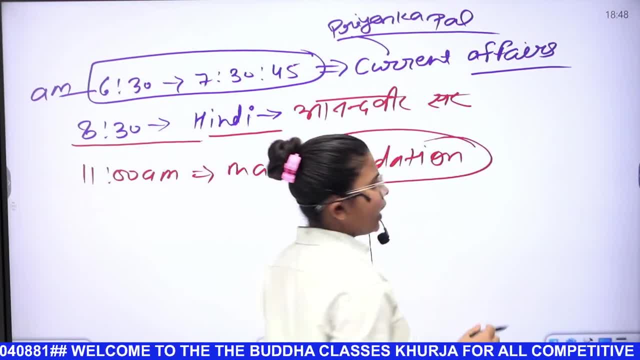 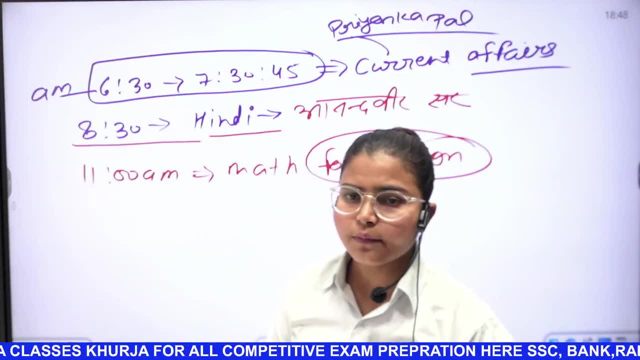 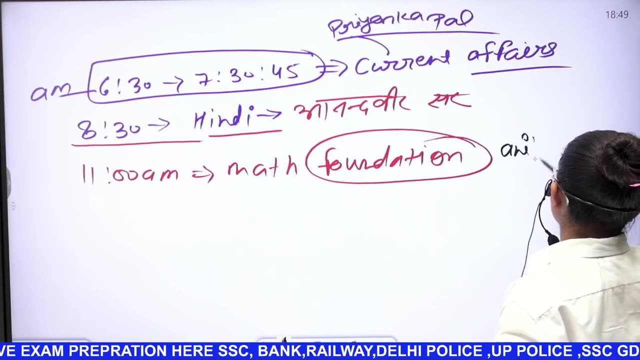 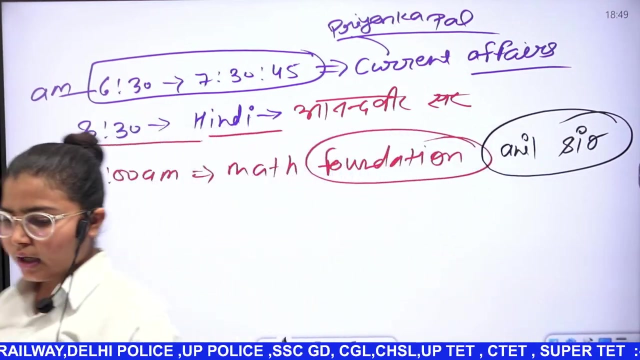 This is foundation class. You are preparing for UPP, RPF, SSC Bank. you are preparing for anyone. this is a chapter-wise foundation class which is taken by our Anil sir. he teaches in a very dangerous way. he clears the concept in a very good way. he teaches you math in a very good way. 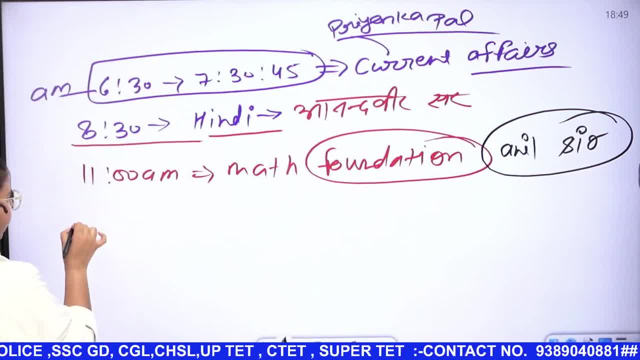 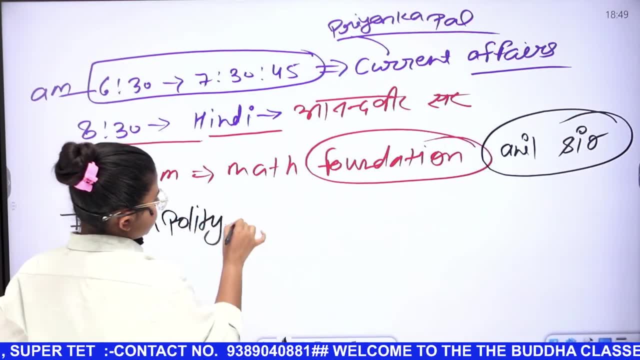 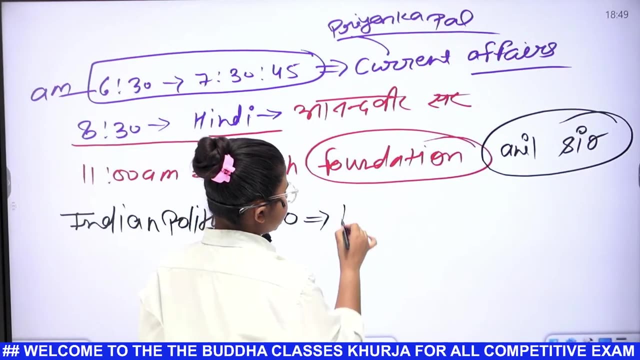 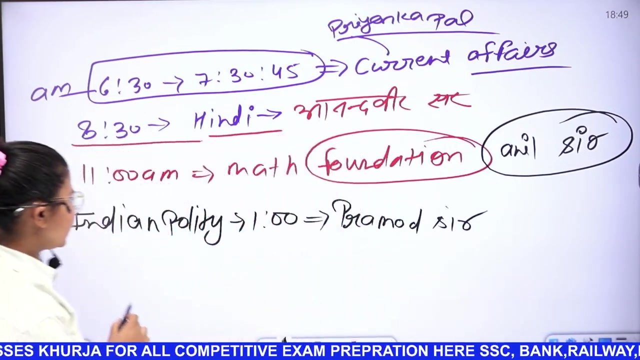 After this I will talk after this: your Indian quality, which comes in GKGS Indian quality. the class of quality runs from 1 o'clock, which is taught by our Pramod sir, right, taught by Pramod sir. after this, the class runs from 2 o'clock. our math is again special. UPP, RPF, SSC. 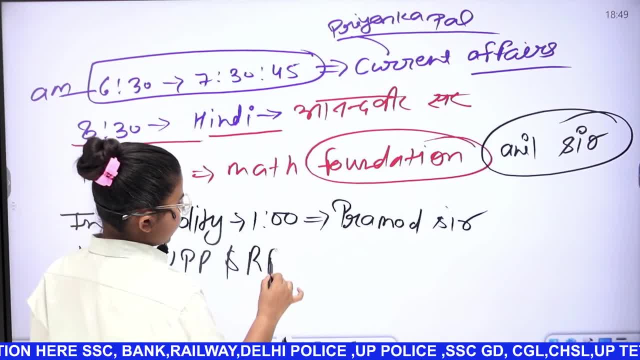 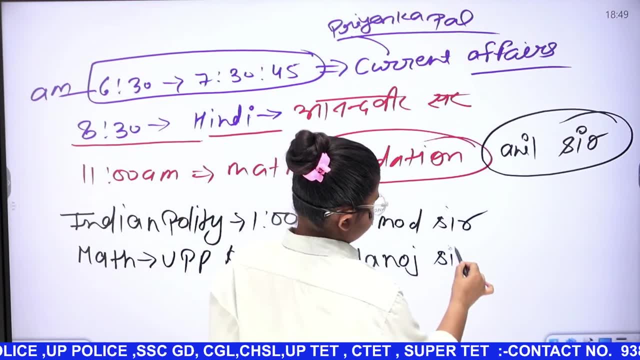 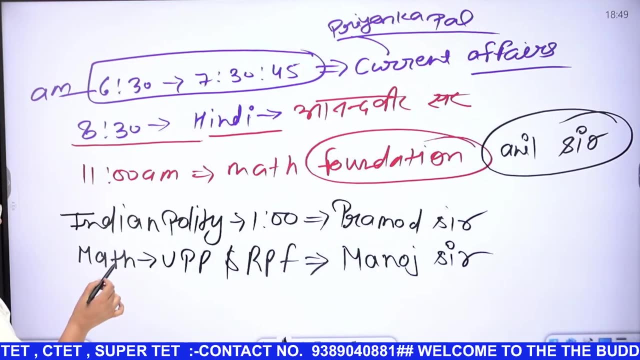 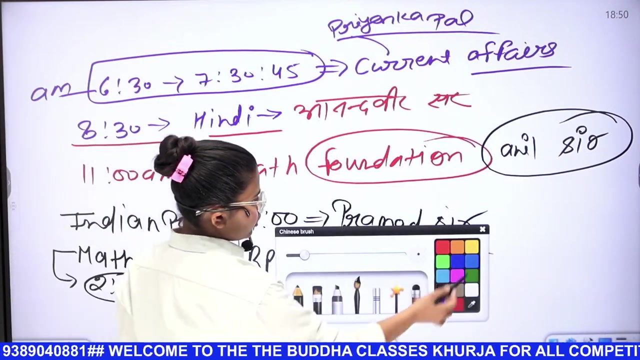 Special UPP and RPF daily class runs, which is taught by Pramod sir. right, which is taught by Pramod sir. remember this: after this, the practice runs from 3 o'clock, this runs from 1 o'clock and this class runs from 2 o'clock. okay, runs from 2 o'clock. after this, its practice set runs: special UPP, RPF, SSC. 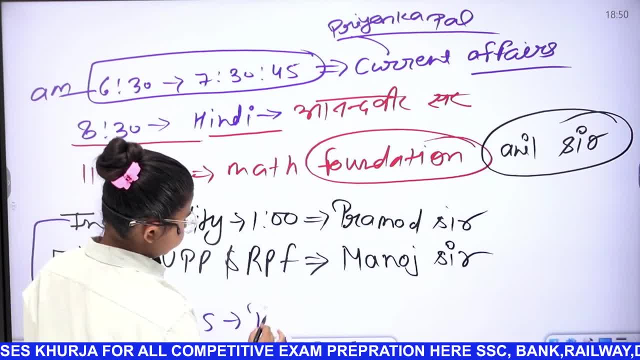 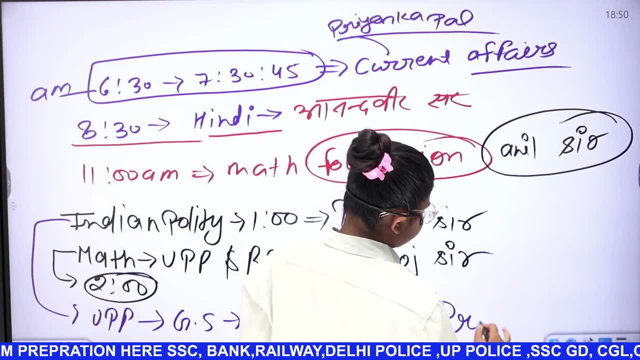 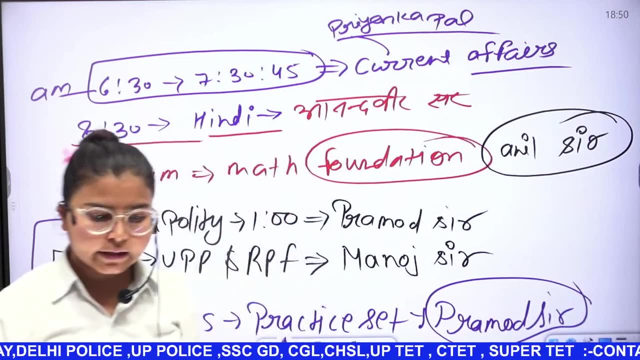 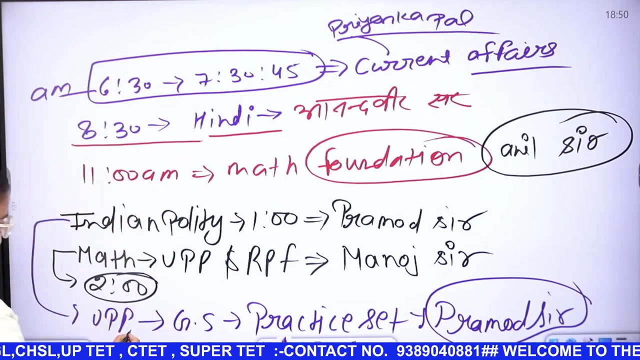 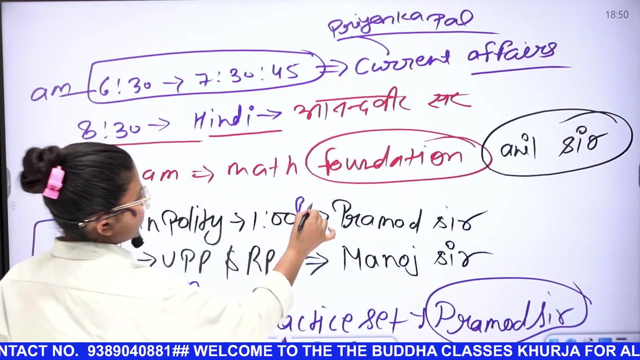 For UPP, there is a practice set of GKS which is being done by the promoter in a very dangerous way. This practice set is being done for all of you, for special UPP, which is taught to you by the promoter After this. this class runs from 3 pm to 1 pm. 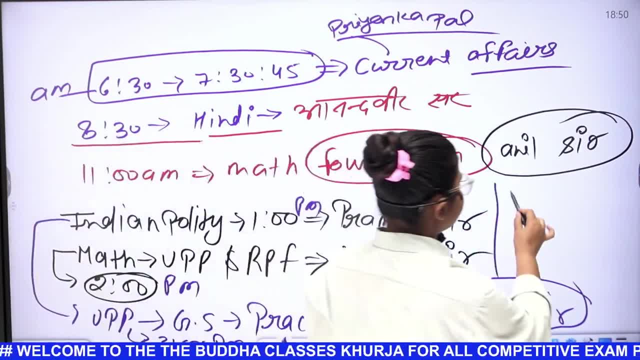 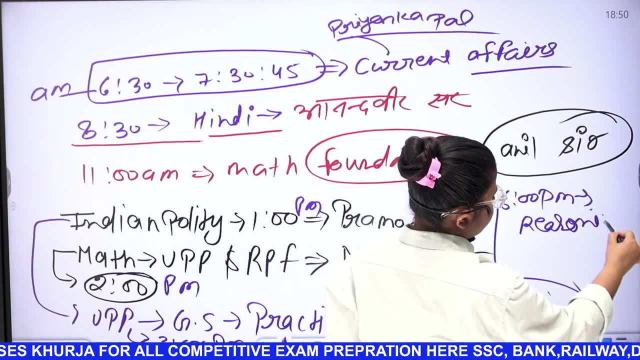 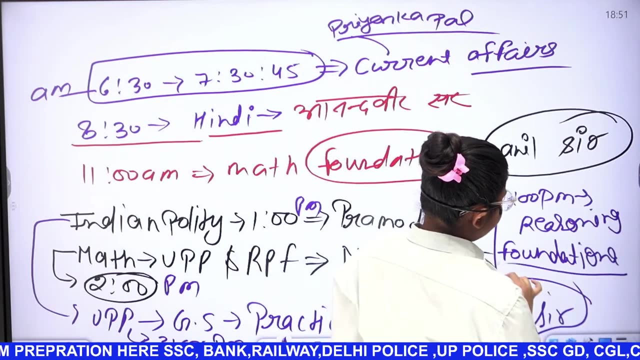 After this, the reasoning class starts from 6 pm in the evening. Reasoning class starts from 6 pm in the evening. Reasoning class is a foundation class. In this all your syllabus will be completed. You will be the founder of this reasoning. 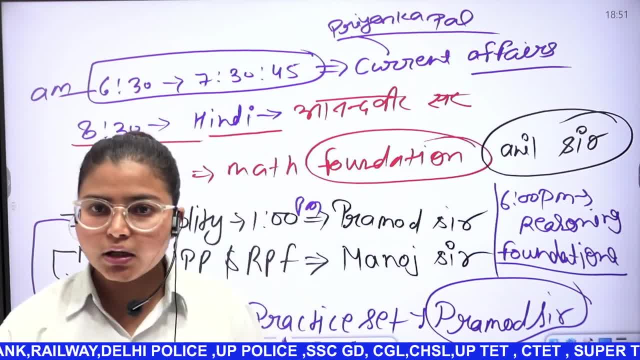 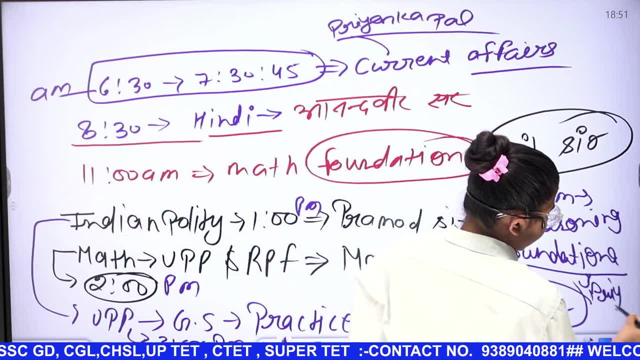 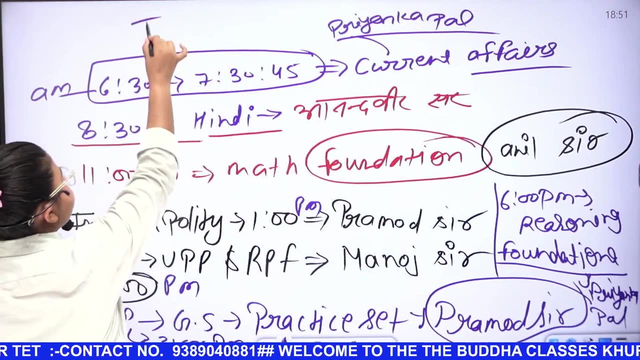 After studying the foundation class. it will not matter if you sit in any exam. This class is done by me. My name is Priyanka Priyanka Pal, Priyanka Pal. This is the timetable of our class Timetable.